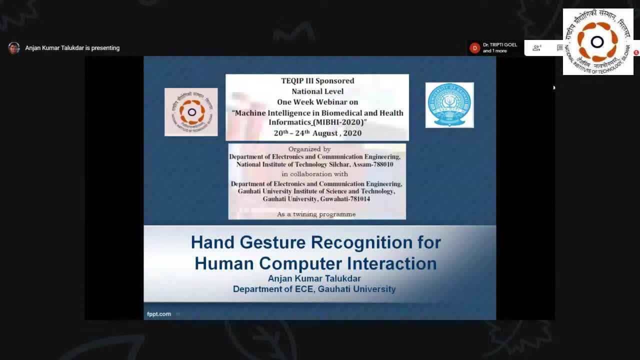 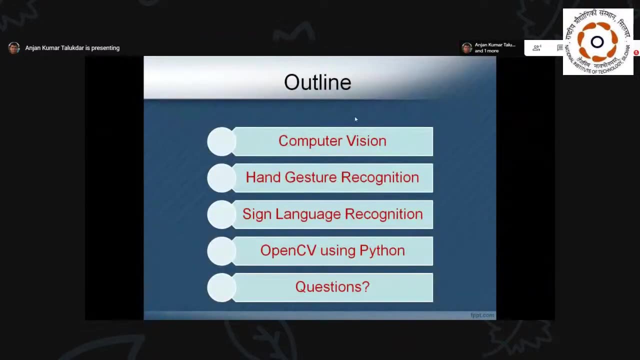 So today I am going to present hand gesture recognition for human-computer interaction. So this is the outline of my presentation. First I will briefly talk about what is computer vision, because some participants may not be familiar with this subject, So I will go through briefly about it. 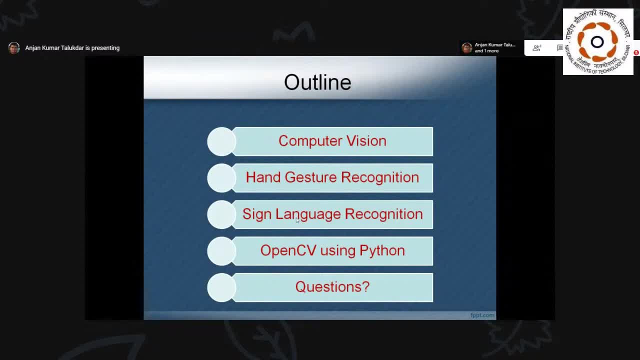 Then I will shift to hand gesture recognition, one of the prominent fields for human-computer interaction. Then one of the major applications of hand gesture recognition is sign language recognition. So I will talk on that also, Then also talk some research problems in both these fields. 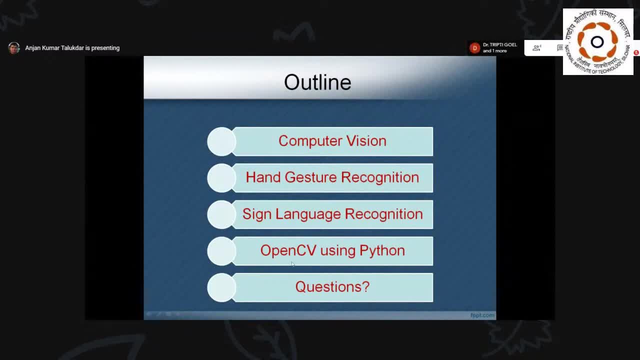 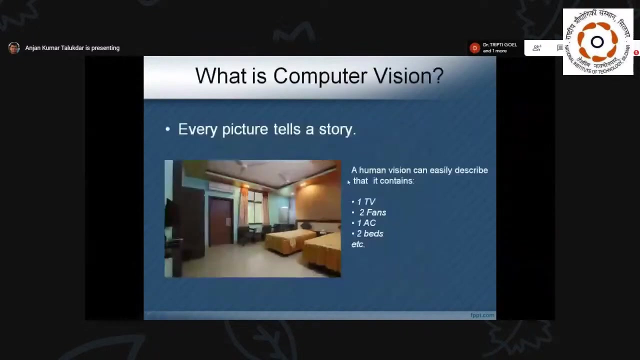 And then, finally, I will show you how to implement some practical computer vision system. Thank you, Using OpenCV on Python. So, finally, I will take your questions. So what is a computer vision? So, as we know, every picture tells a story. 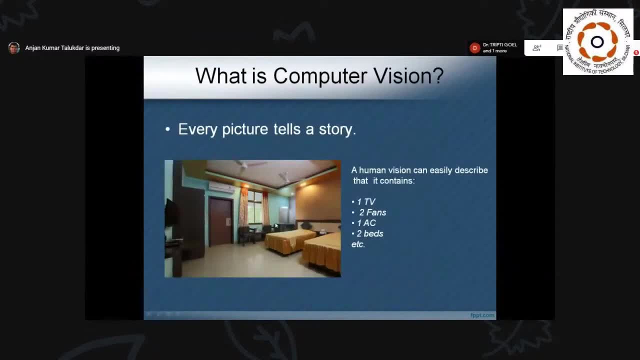 So if I ask any one of you what will you see, what you see in this picture, then you can easily answer. But answer may be various. Something someone may say: I have seen: one TV, two fans and one AC, two beds. 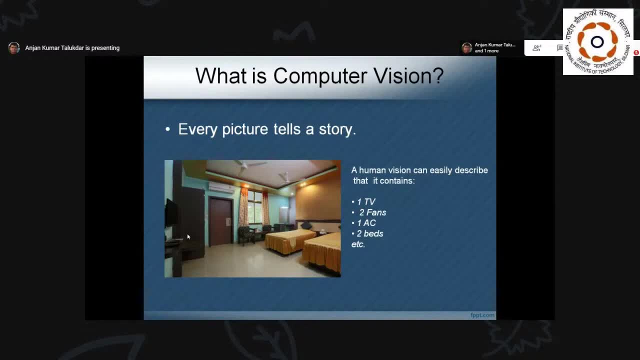 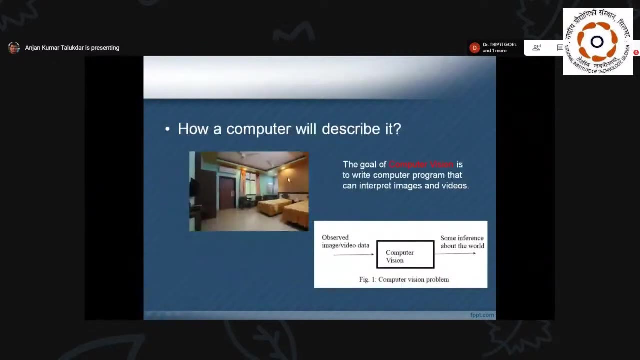 Then a color of the bed: yellow, So like that. So we can describe this image in various ways. So now how a computer- actually actually this- will describe this image. that is the basically the goal of computer vision: to write computer program that can interpret images and. 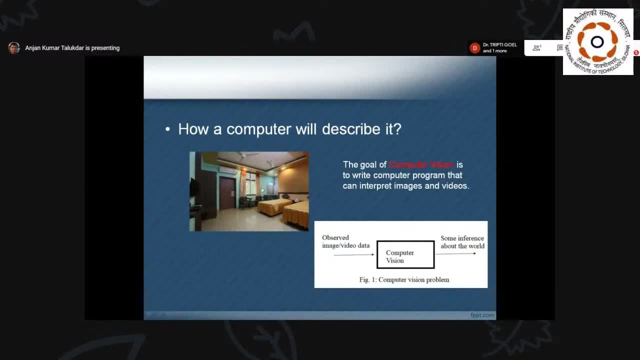 videos. our human visual system can easily describe this image. but how a computer will describe or interpret this image? that is basically the goal of computer vision. so input to the computer vision system is an image or video data and output is some interference about the world or the 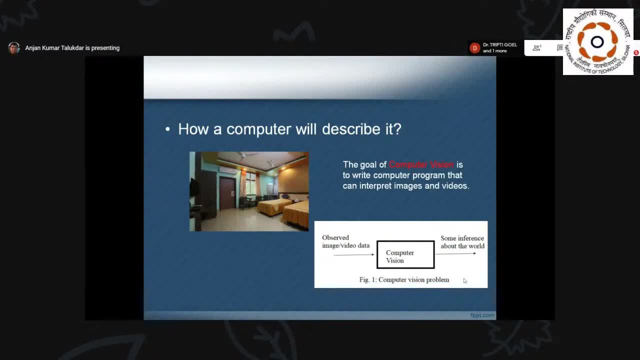 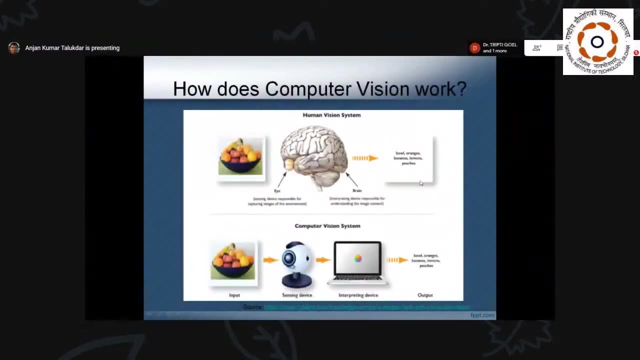 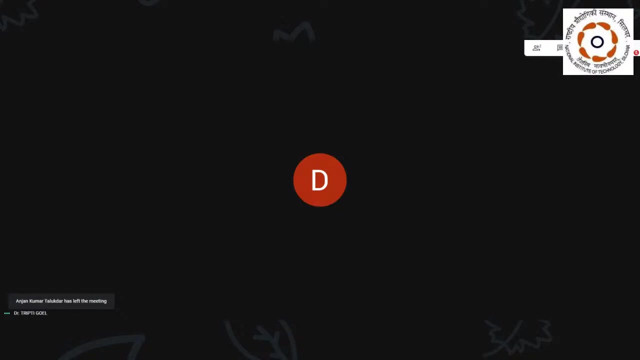 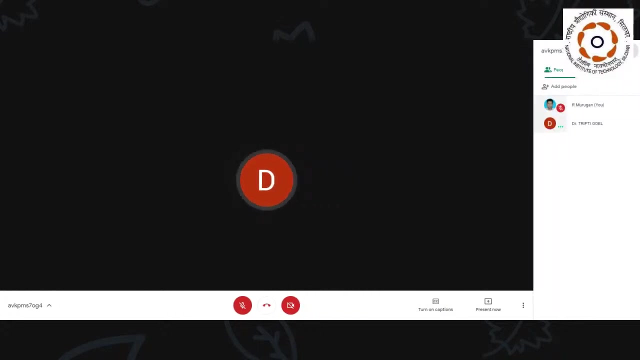 interpretation of the image or video data. so how does a computer vision work? so the top figure shows our human you. Hello sir. Sir, network issue may be there, so wait for some time. Yes, sir, Thank you, Thank you, Thank you. 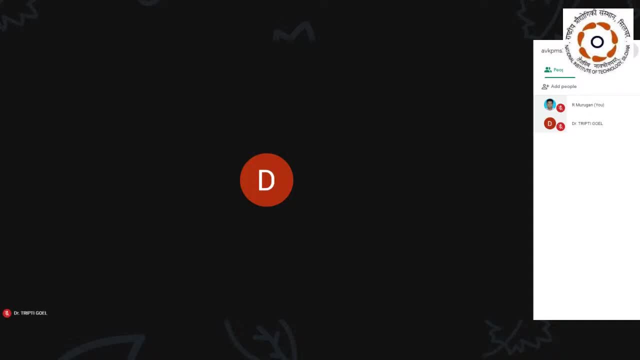 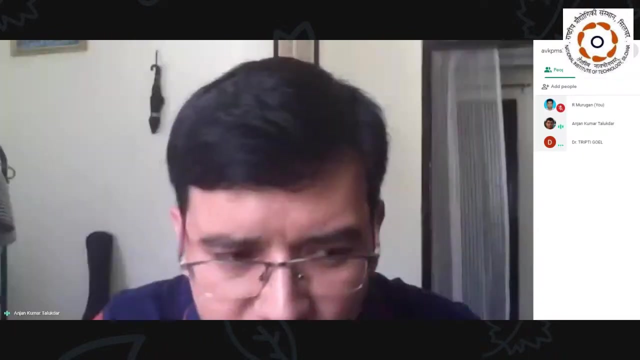 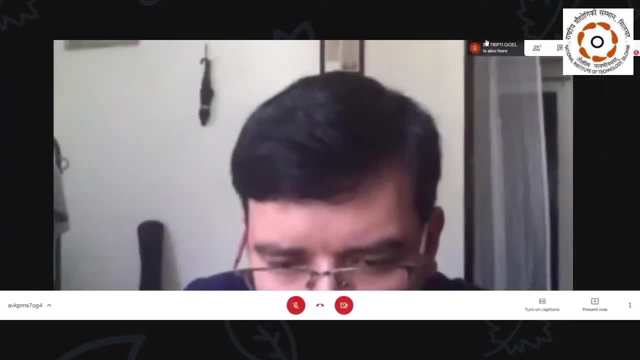 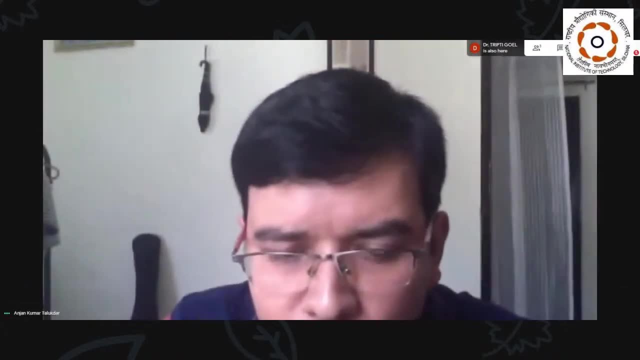 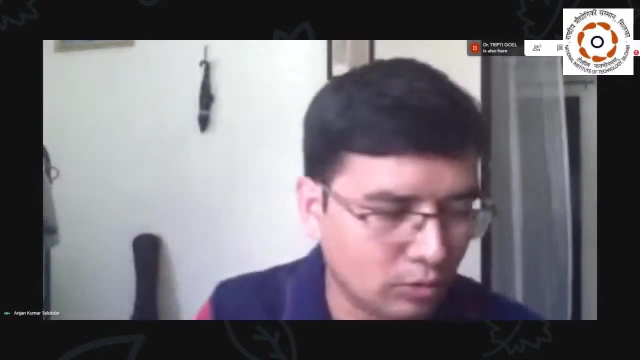 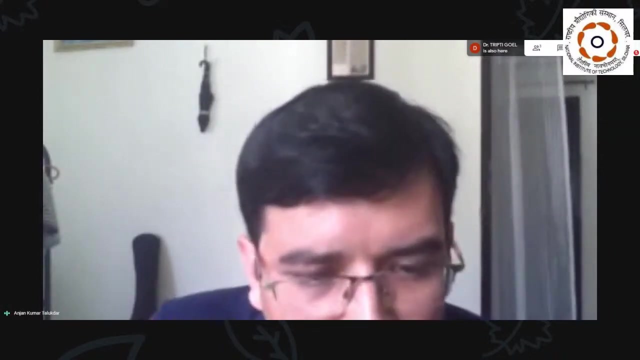 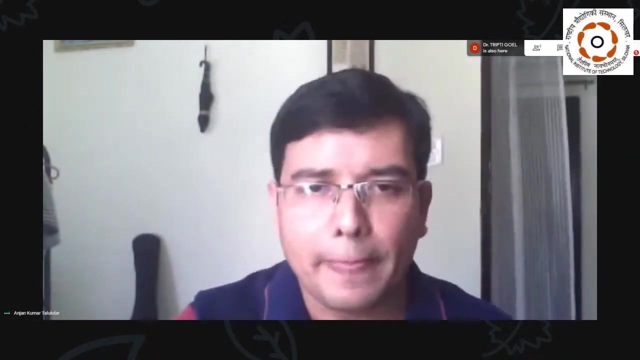 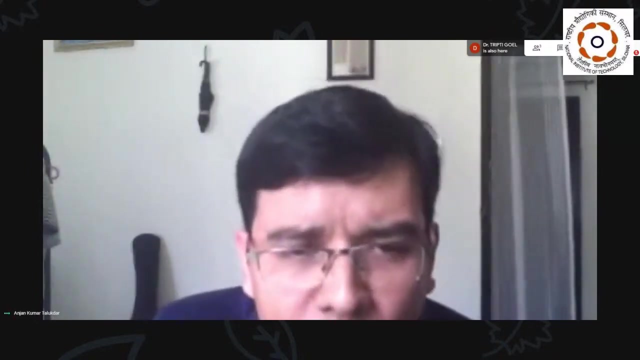 Yes, sir, You have to start from first slide. Okay, So very good afternoon to all of you. So I'm going to present hand gesture recognition for human computer interaction. So this is the outline of today's presentation. First I'll briefly talk about what is computer vision, because some of you may not be familiar with this. 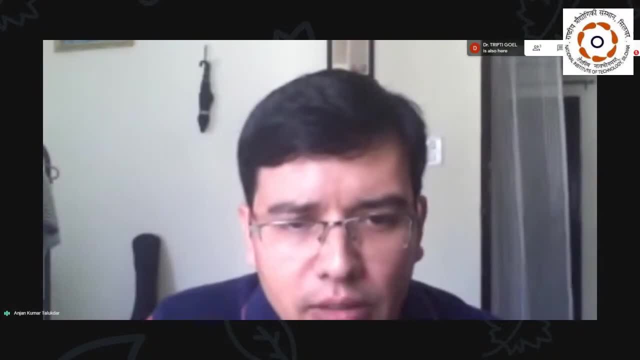 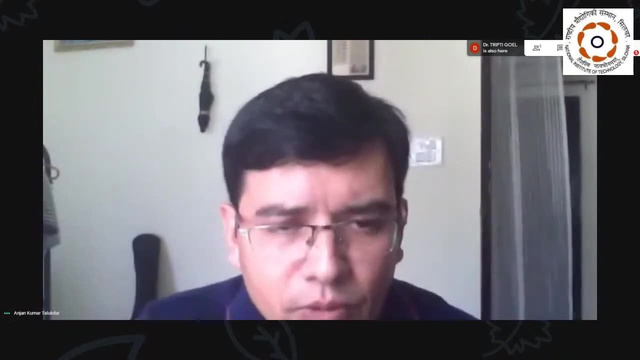 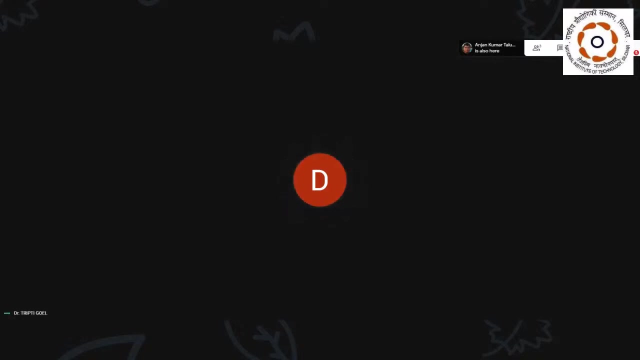 So I'll briefly talk about that. Then I'll, Okay, Talk about hand gesture recognition, which is one of the Hand gesture. Yes, Please share your presentation slides. Share the slides Slides. Okay, Slides are not visible. 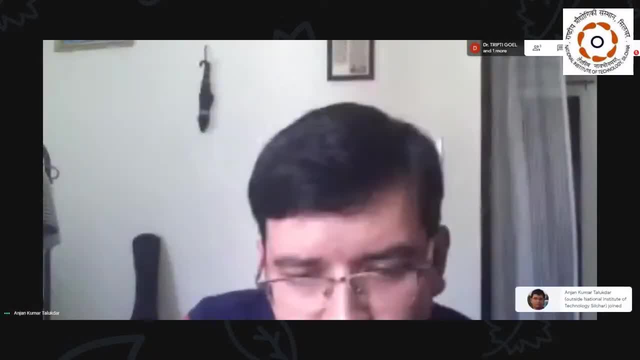 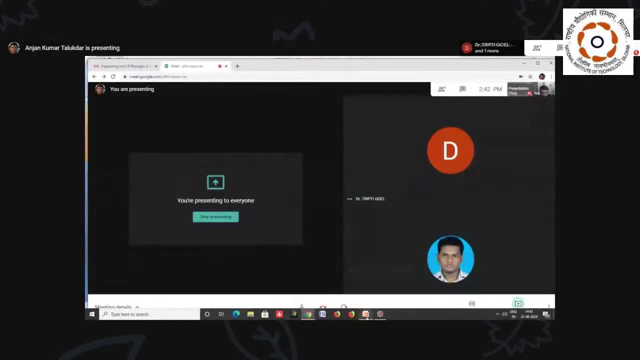 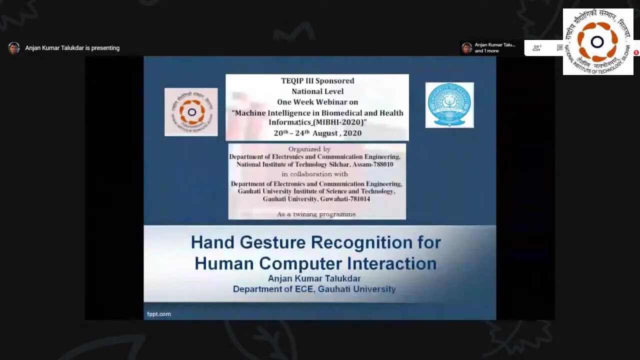 Oh, yes, yes, yes, I can see it. Okay, I'll share the slides. I think that's good. Yes, sir, So this is a hand gesture recognition for human computer interaction. I see, Okay. So good afternoon everyone. 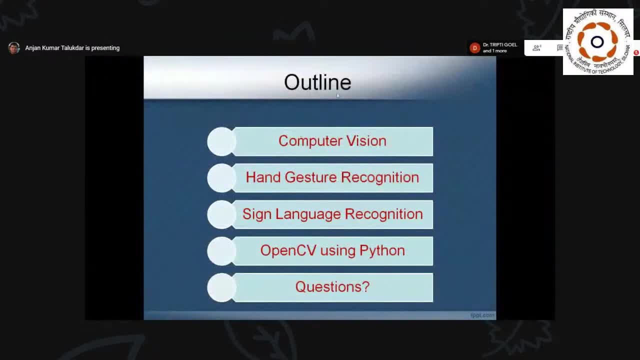 So you can see that this is my hand gesture recognition. I hope you can see that sign in, please, And also you can see with the hand gesture recognition. you can see that there are only eight of us. Okay, Thank you. 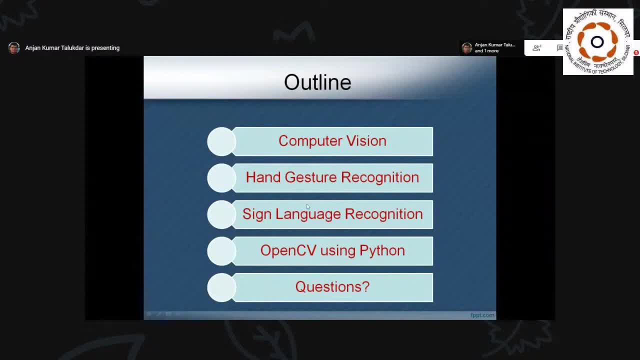 So, okay, That's it. Okay, So, okay. So that was it. I will now talk about hand gesture recognition for the future of Human-Computer Interaction from this field. so I'll briefly go through that, Then I'll talk about hand gesture recognition. 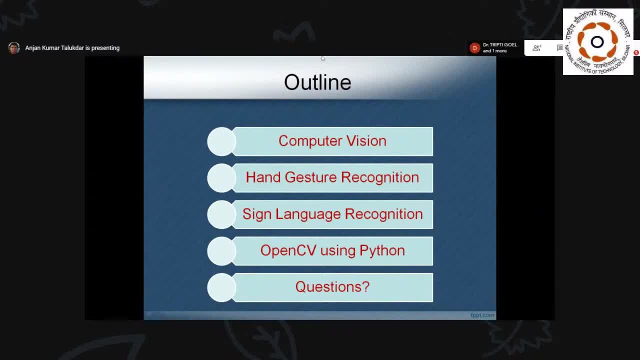 which is nowadays a prominent technology for human-computer interaction. Then I'll talk about sign language recognition, which is one of the major applications of hand gesture recognition. Then, finally, I'll briefly show you OpenCV, Open Computer Vision Library for implementing any computer vision project using Python. 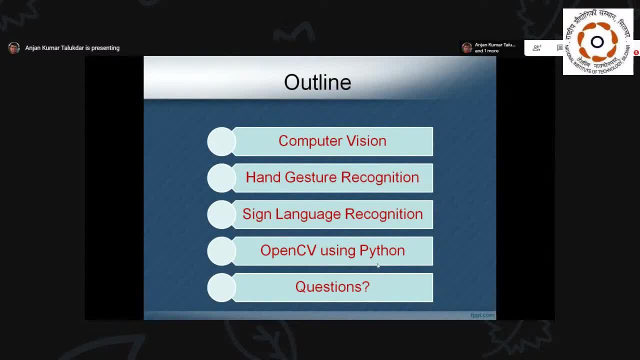 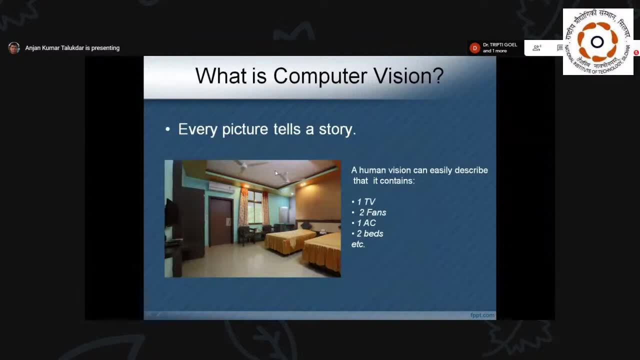 Then finally, I'll take your questions. So what is a computer vision? So every picture tells a story. If a human is asked what he or she has seen in this picture, so he or she will quickly give answers like I have seen a TV, or he or she may tell: 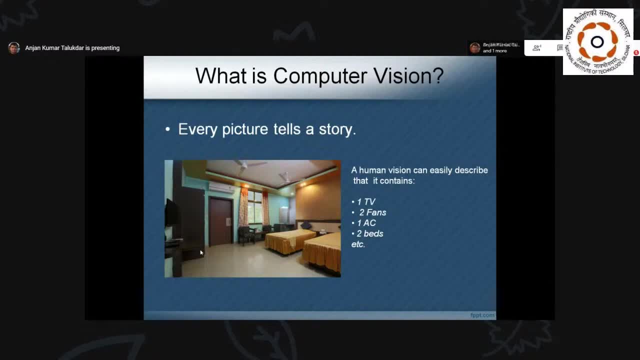 that I have seen two fans, one AC, two Beds et cetera. So it is not a difficult task for a human being, except a child or an adult human being. It is not a very difficult task to do absolutely. 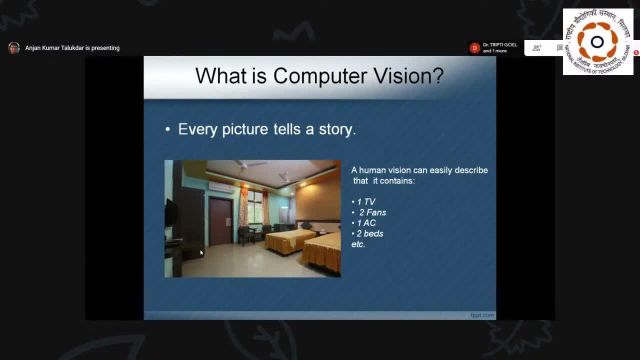 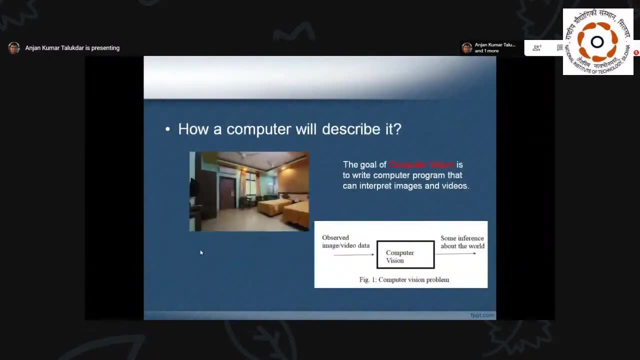 very difficult problem to describe this image in various ways, but how a computer will describe it. that is the basically goal of computer vision: to write a computer program that can interpret images and videos. okay, so input to computer vision systems is image or maybe video data and this computer vision block will take this input and do some. 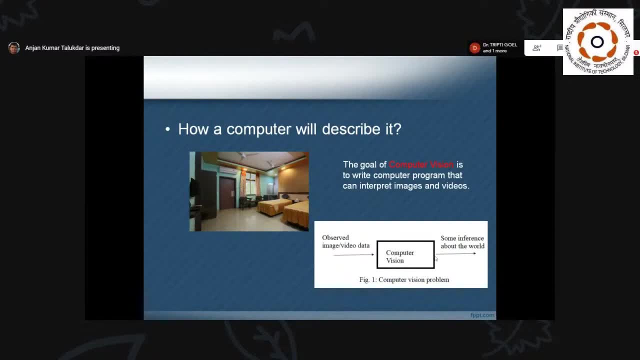 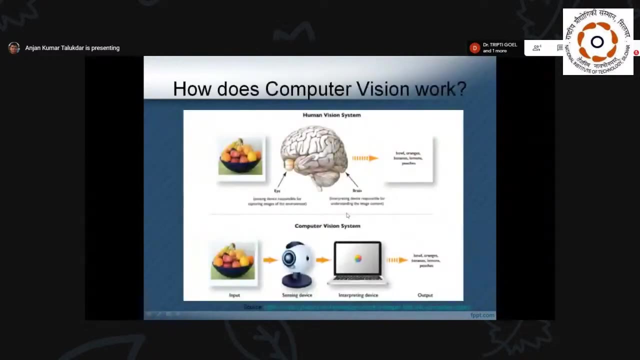 processing on that input and give some interpretation of the image or video as output. okay, so this is a basically the computer vision problem. so now, how does computer vision work actually? uh, so this above uh figure shows how a human vision system uh works. so suppose this is one picture. um, uh, so, uh, we look at this, suppose, image. 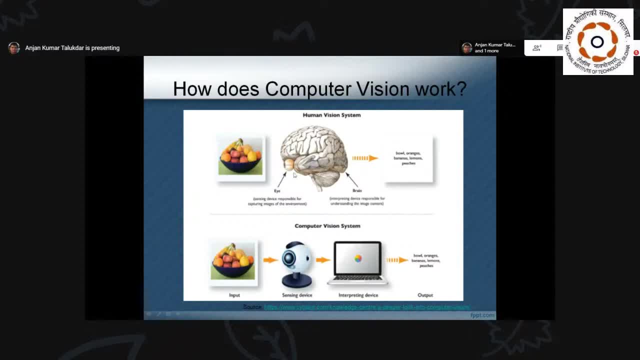 uh for eyes and does uh so i. i will keep. uh signals will be formed on the retina of the eye and those signals will go to the processing image of brain. the brain will process those uh signals and will give some output like uh bowl, oranges, bananas, lemon. 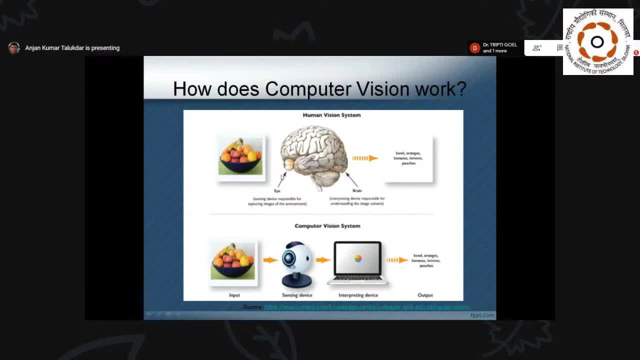 etc. so here, actually, our, our eyes are the um sensors. they work at some sensors and human brain works as uh processing in it. now, so in computer vision, actually, we are uh trying to uh replicate this human vision system with the help of a computer and a sensing uh, a sensing device. so in computer vision uh. 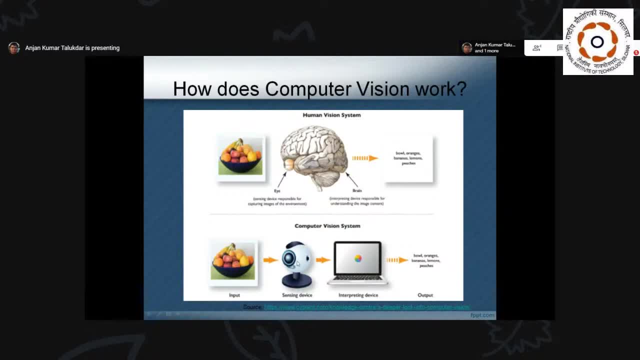 suppose input is same and our sensing device is generally a camera or some other kind of sensor or some other devices also. i'll discuss about those also. uh, then, suppose the camera captures the image, then that image is uh sent to the interpreting device. suppose a computer, and the computer will process that image and apply these various algorithms, various models. 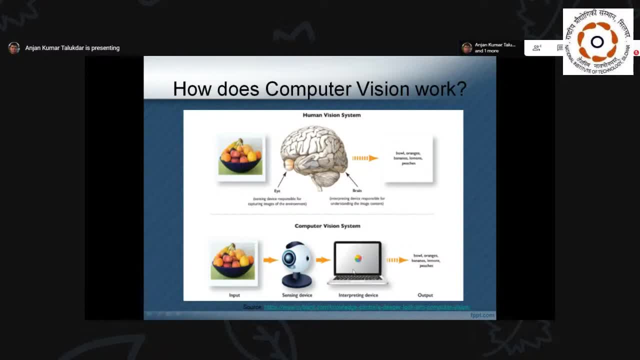 so ultimately it will give outputs like bowels, orange, bananas, lemon and cooled down the images, lens and finances, let us say a glass of cool, qualquer big camera. so the maps will come out. so only one channel or two channels are there, and the Hindu camera in this film will browse the intelligence and signals from emergency mode in same frequency. 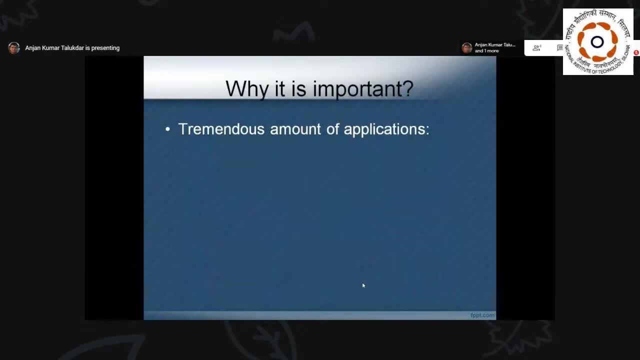 the- yeah, other camera processor or the glass or, and not one, is the outer image is used to be flashed. uh, called zweithey, is its ability to read the carrier and can be used for, uh, uh, like to tell that people know that you guys are mashed or you know how you see your body. 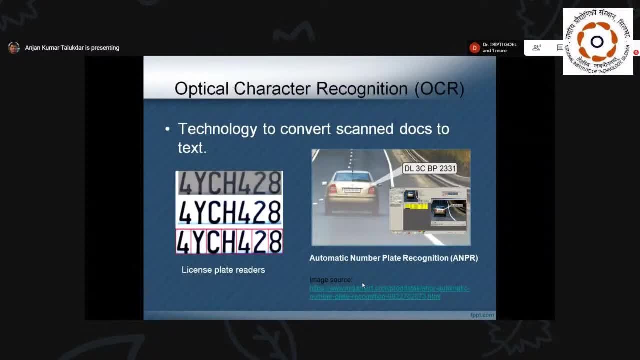 you can write it. marshes other things, you can correct it simply into your brain. optical character recognition: it is a technology to convert scan documents into text. one application can be license plate readers, so this is the scan image of the license plate and this is the output. 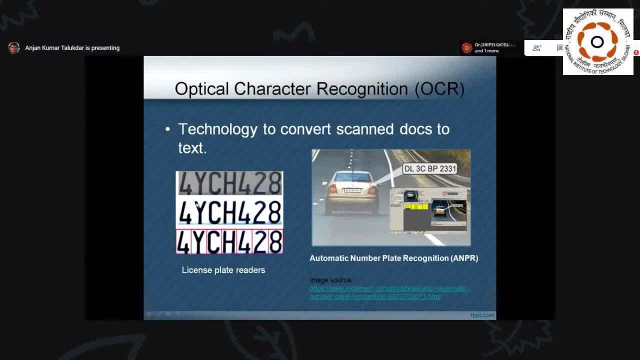 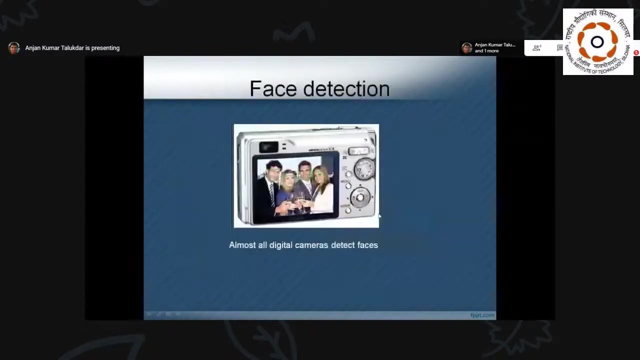 where we are reading the visits or letters present on the number plate. so so now, nowadays, this automatic number plate recognition system is being applied. so you can see on this image, the right side image, that this technology is being used for detecting the number plate. so then, second application can be your face detection. so nowadays, most of you have smart cameras, so 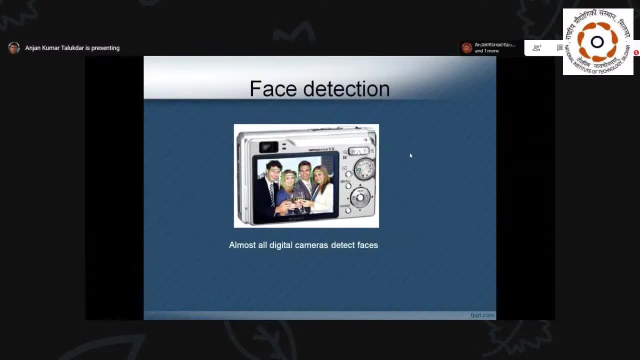 you have smart mobiles, so in your smart mobile phones your smart cameras are there. so, yeah, these cameras can not only capture image, but also it detects faces, or even your age also in some cases, and many features are there, okay, so these are becoming possible only because of this. 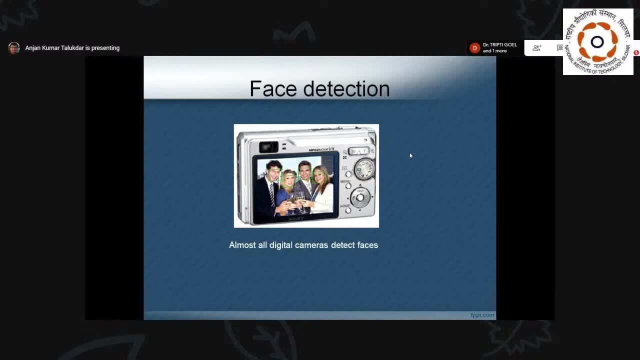 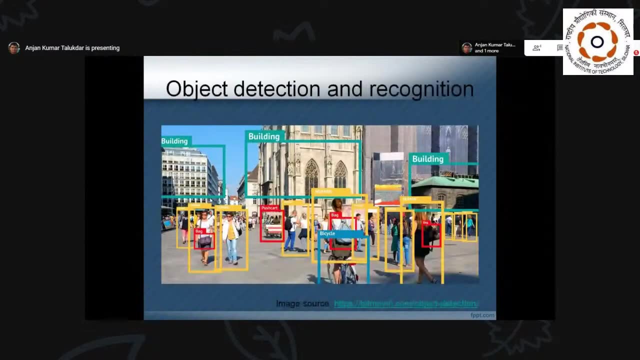 computer vision technology, then object detection and recognition, so you can see from this image that various objects that are present on the image are being detected. this is building, this is human, this is babe, okay, so like that. so this is. this is not only detecting, but also localizing. this means it is also finding: where is it, where is the human? where? 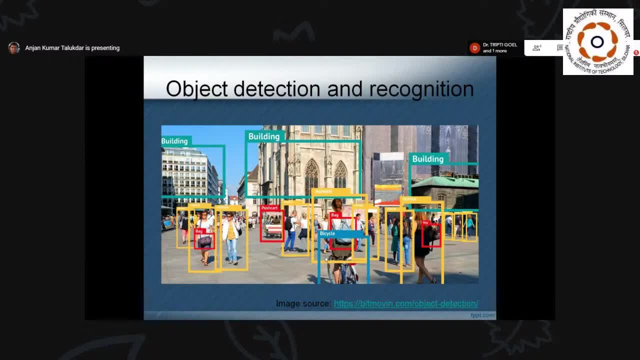 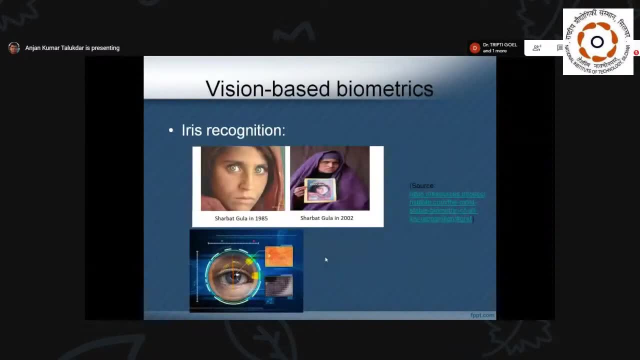 is the bicycle, so this is the object detection and also recognition. so next uh application can be your vision based biometrics. so nowadays we use uh this kind of biometrics, like finger pins or this iris recognition. so this iris recognition, actually uh is one of the applications of computer vision based system. so this is an uh nice example we can discuss. 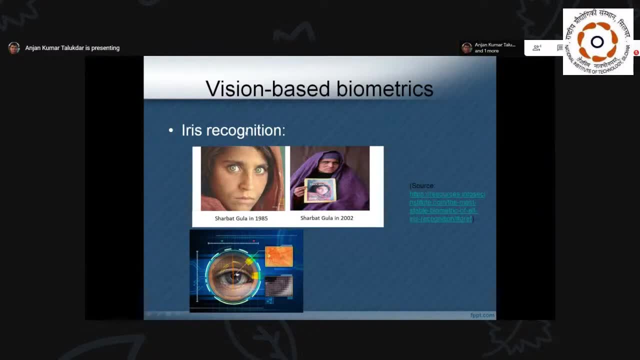 for this iris recognition. there is a story actually behind this that this uh side, uh, she is basically from afghanistan but uh, even the invasion in afghanistan, she fled with her family to pakistan. so one photographer actually uh capture her image because her eyes are green in color. so 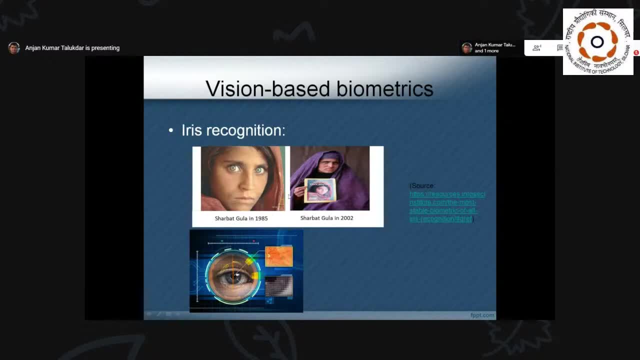 this is the peculiarity cee had. so the photographer took her image, But after almost 17 years, when the same photographer tried to find her, it was difficult to find her because this was a picture of the same lady, Sarbat Gula, in 2002.. So, actually with the help, 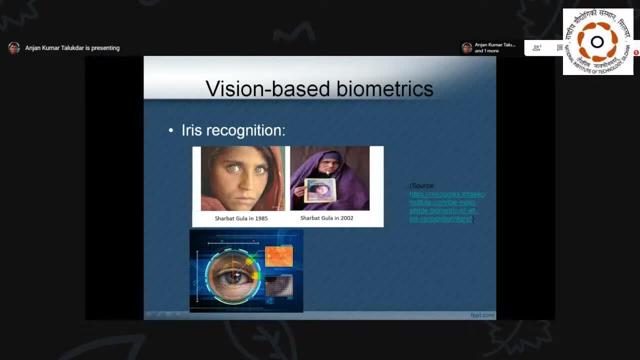 of this iris recognition, it was detected that she is the same girl, Sarbat Gula. So, actually, because our iris has one peculiar pattern which is unique and does not match with others, so this iris recognition can be used as one of the important biometric techniques. So 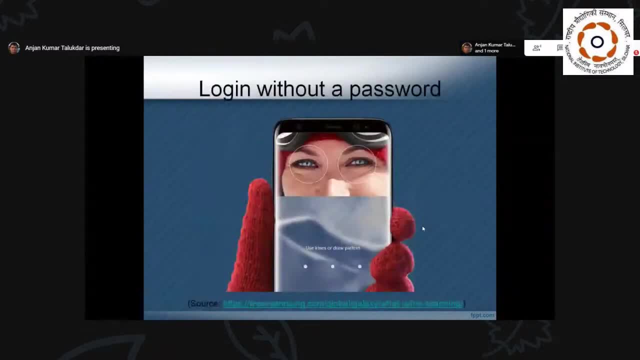 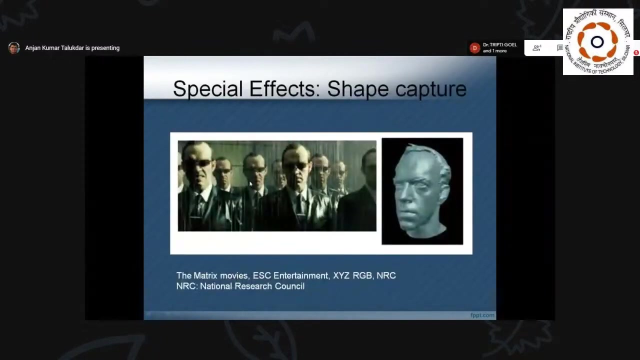 then you know that this feature is also now coming and come to our mobile phones. login without a password means it basically takes your iris as input and it detects whether you are at the authorized person or not, so this technology has already come. then in movies also, we see some special effects. so this movie i think you can remember this is the. 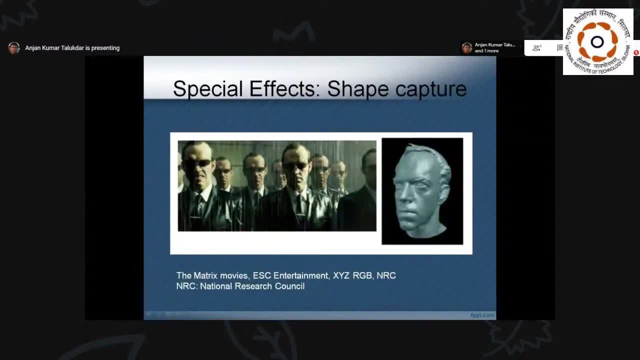 the matrix movie, right? so here, actually, what is done? suppose this person first his 3d, save his model like this way, so using cameras from various sites. so first a 3d model of the person is a model, and then we vary the parameters of the model to. 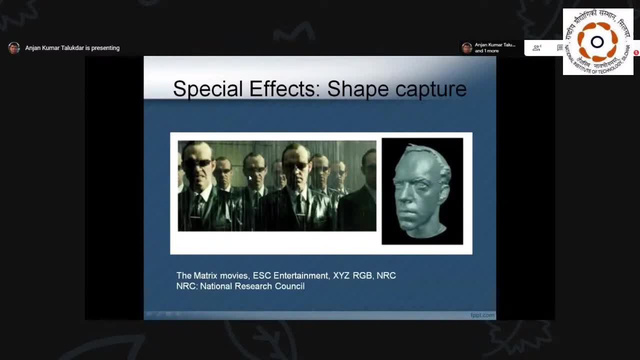 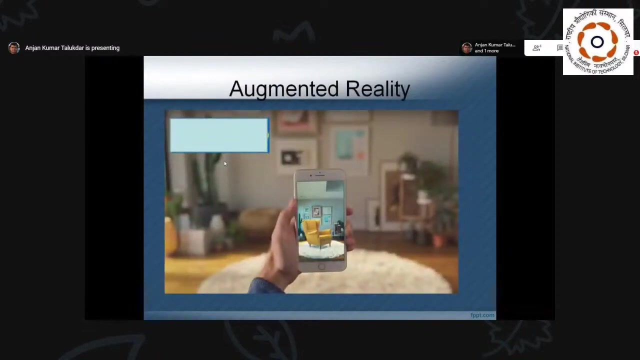 generate various or replica of the same person. you can see in the background the same person, but with various expressions, or like that. so this technology was also used. movie, so then augmented reality: as you know, uh, this visitor basically uh mixing up your uh, virtual and reality, virtual and reality. so so it has now many applications. 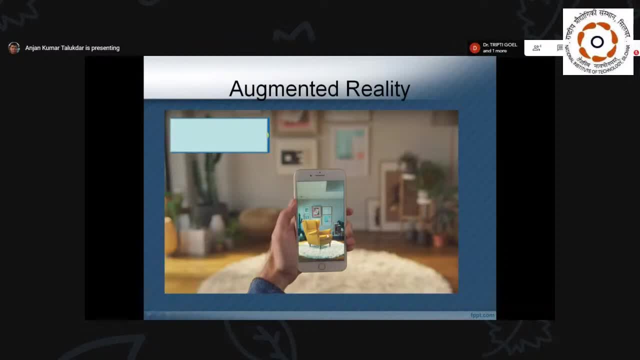 so for example here: suppose uh that person is going to uh buy one sofa, so we can actually uh test whether that sofa will be matching um in his room or not. actually, this uh background image is the real image of this uh room, but this sofa is the virtual. okay, so it is a mixing, mixing. 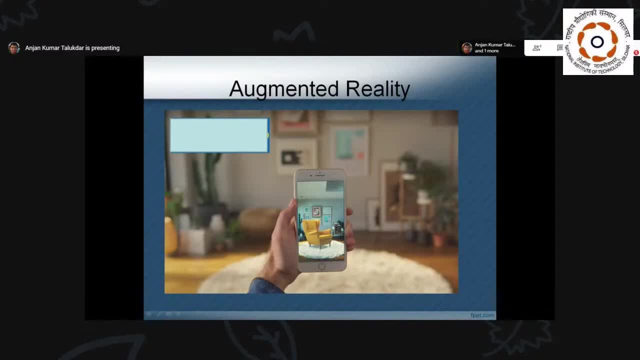 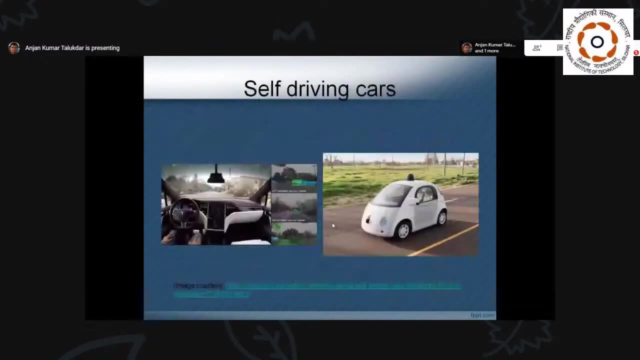 of this area really, and the virtual. so apart from this also, it has many applications. so then you know, self-driving cars, uh is also coming, so so without driving also, the car can determine the its part and other parameters. okay, so for that one, is uh camera is there or some radar? actually, this system is there then. 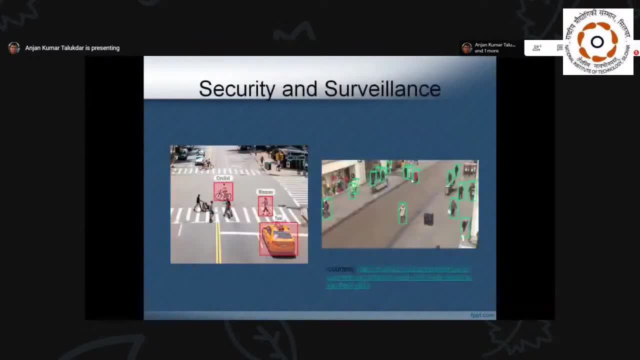 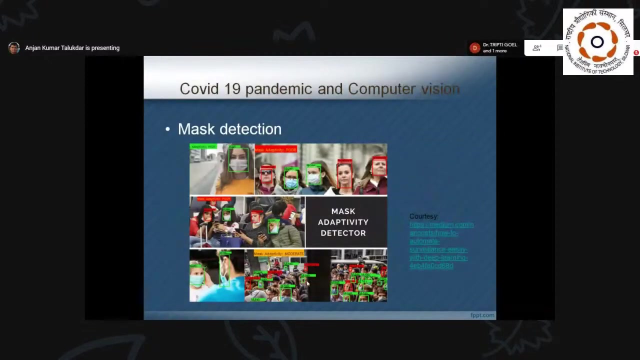 and this is also one very important area- that security and surveillance. okay, so nowadays this is also being deployed for security and surveillance. so then, uh, in now in present situation means with nine pandemic. uh, how computer vision can play an important role. so people have already done uh, works on it. 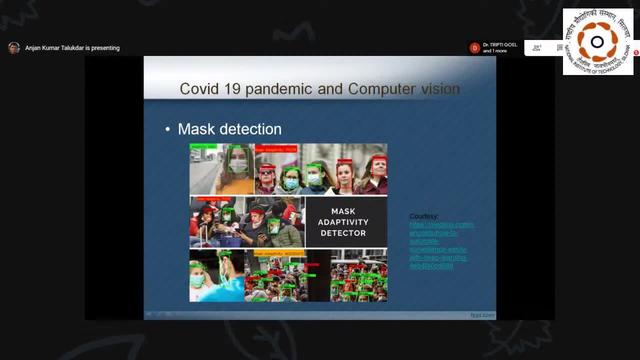 for example for a mask detection, whether a person is carrying masks or not. so this uh kind of detector has been already implemented. for example, you can see that here this no max, then max, max, no marks, like that. you can use uh computer vision or technique for this also. then 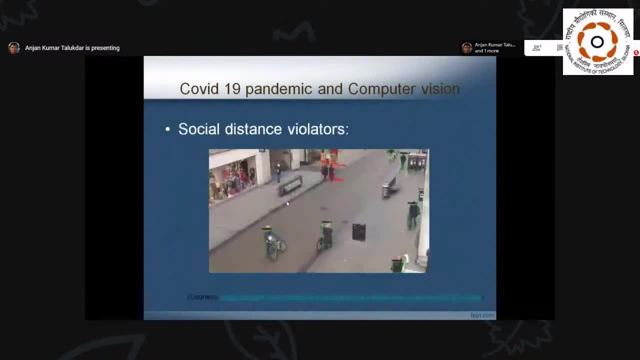 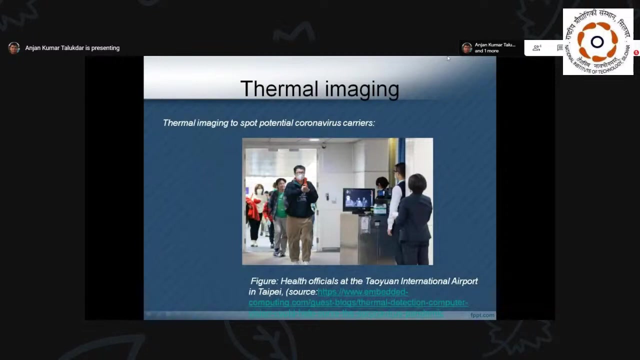 social distance violators. you can check whether people are maintaining social distancing norms or not. for example, if the green box is coming means they are maintaining social distancing, but if it becomes red means they are highlighting the social distancing norms. so, similarly, thermal imaging is also becoming one very important. 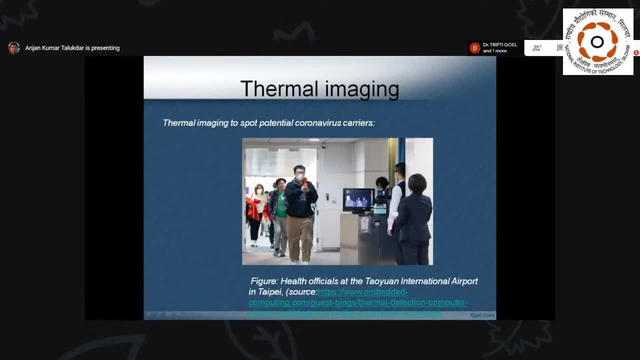 for this situation that with the help of thermal image, we can detect whether person is having some fever or any symptoms or not. so, for example, this is the image taken at the taiwan international airport in taipei. so basically, it is believed that number of people infected in taiwan. 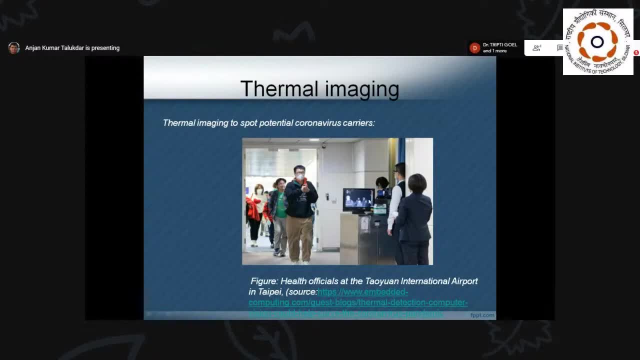 was very less because of this technology they implemented. so now these are some applications in general, and now i am going to discuss some application related to your biomedical applications, because i believe that many people have joined this workshop, uh to know about machine learning applications in biomedical and handheld. 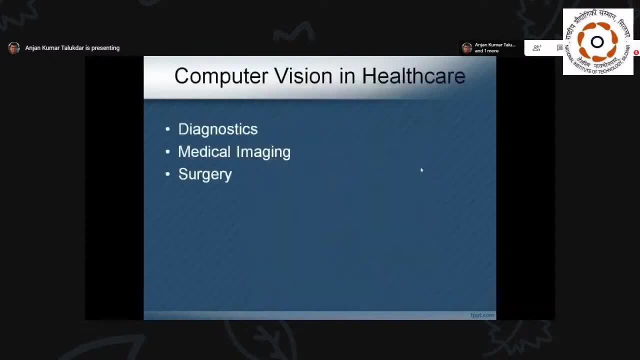 sciences, so i will be discussing briefly about how computer vision is playing important roles in healthcare. so i'll uh, so these are the excellent major areas where resources are are going on and those who are interested may work on these fields. uh, so i will please discuss these three fields. 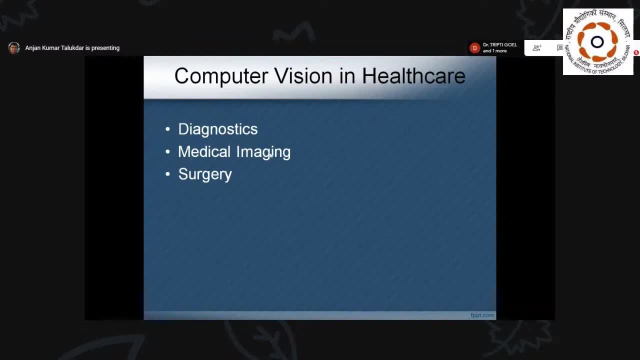 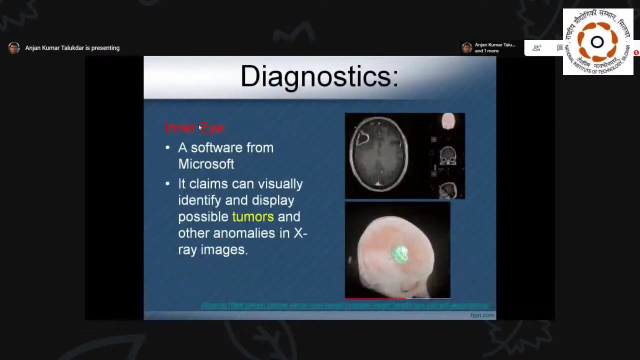 one is diagnostic, then medical imaging and then surgery. so how computer vision is playing, uh, its role in this place. so first a diagnostic, so one actually software called inner eye that is produced by microsoft, actually, so a software from microsoft, uh, and it claims, uh, that it can visually. 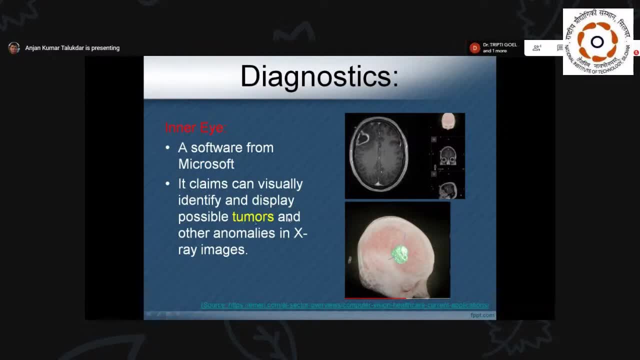 identify and display possible tumors and other anomalies in x-ray images. so, for example, you can see um this, this portion, this white boundary portion, so there is a tumor there. so the software can uh detect this uh tumor. and once you uh detect this tumor, and if you uh mark it uh, then you can see. 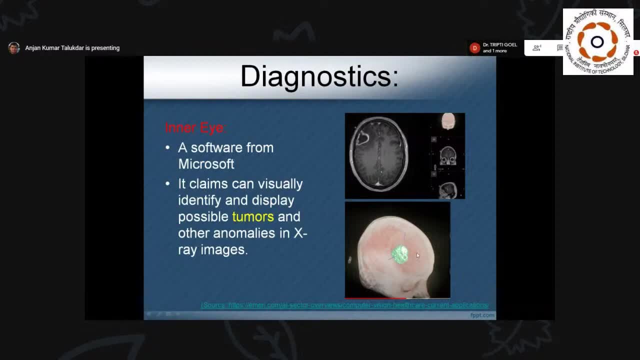 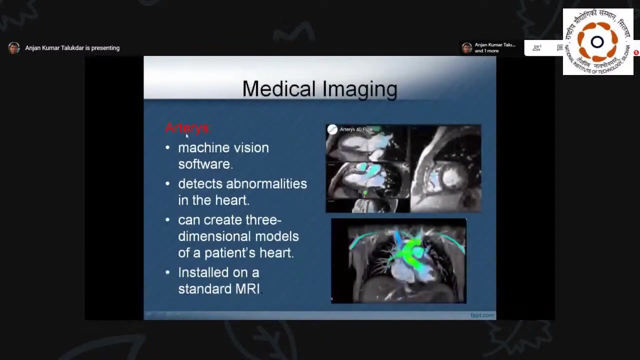 see the 3d shape of this tumor. so it helps to diagnostic, to diagnose this tumor and also do a person this tumor easily. and the important thing is that it takes very less time compared to manual diagnostics. so the second reason can be medical imaging. so one company called Arteries they have produced one. 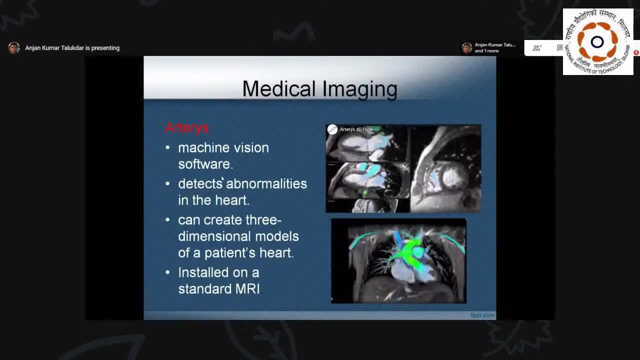 software, a machine vision software that detects abnormalities in the heart, so their algorithm is known as Arteries 4D flow, and so they detect abnormalities in the heart and also can create three-dimensional model of the patient's heart, and this software is installed on a standard MRI machine. so this is how we 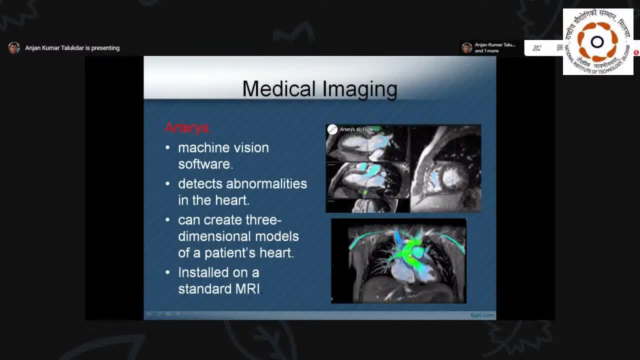 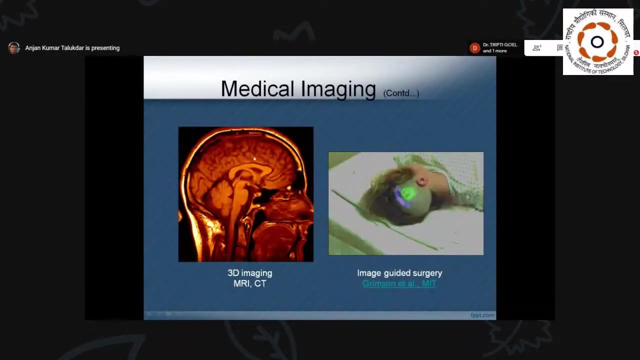 can also even monitor the flow, blood flow through this heart and everything. so that's this is one application. then other application can be your 3d imaging. in case of MRI, on CT scan you can have 3d image also. this is right hand image side is an image of image guided surgery. so like that, you can have a 3d model of. 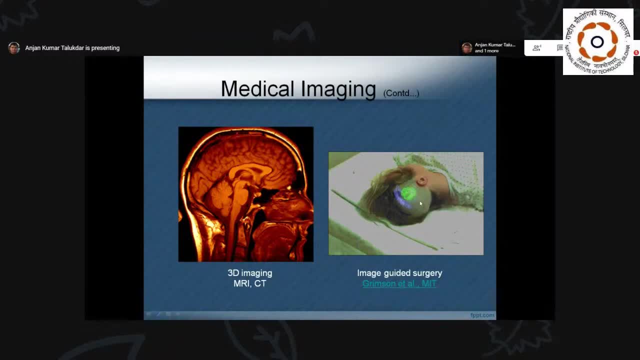 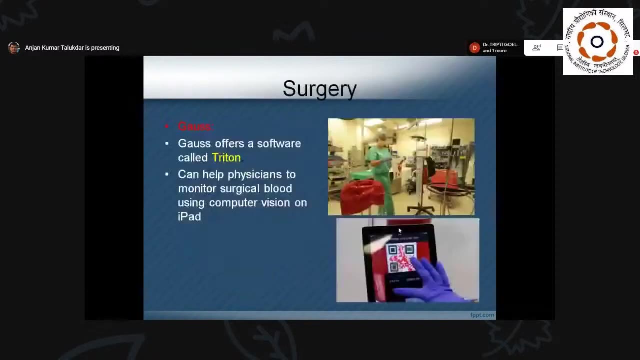 this tumor suppose, and also the brain. so it is helpful for robotic surgery or also remote surgery. it helps in those cases then in surgery. also one software called Triton that is offered by one company called Goss, so it helps actually physicians to monitor surgical blood using computer vision on iPad. so what is? 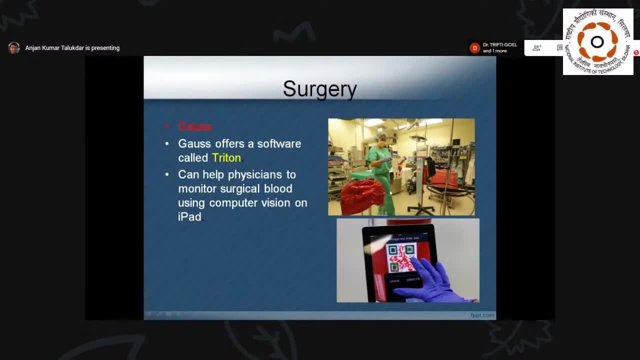 done, basically, actually, this soaked blood towels or this sponge- these are actually displayed in front of this camera and this camera captures this image and it processes this image and ultimately, it determines how much blood was lost by the patient like that. so they have not disclosed their algorithm, but, uh, this is working fine. 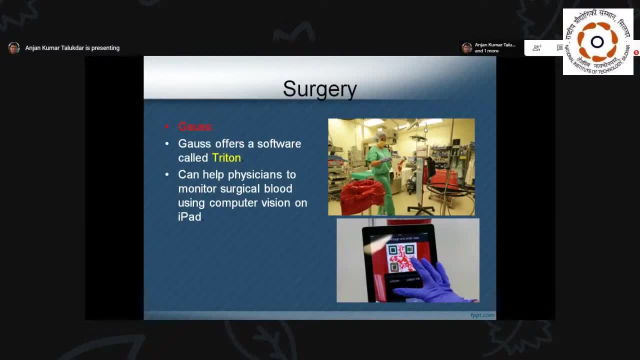 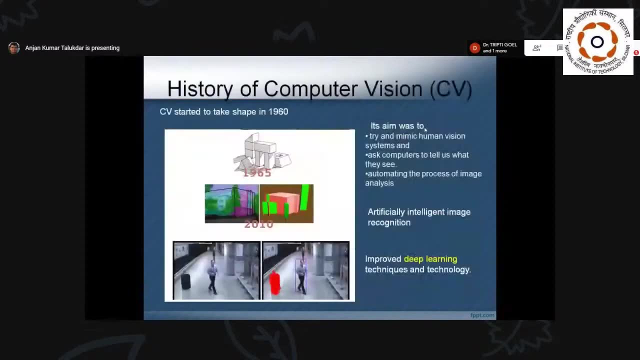 then uh, this is some application in case of medical fields. so now I will briefly go through a history of computer vision, actually how it actually came. So computer vision started to take shape in 1960.. So it aim was to try and mimic human vision system and ask computers to tell us what they see. 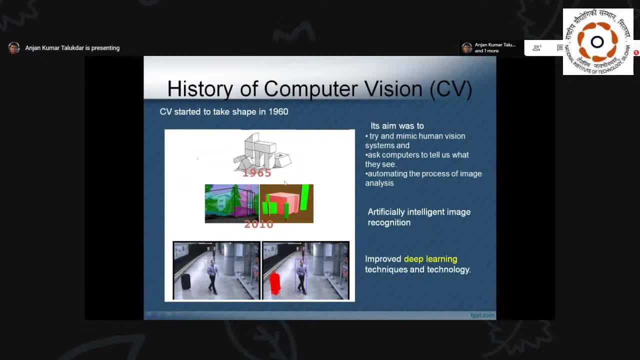 So initially, around 1965, basic features were actually detected, like shape, boundary, etc. And then in mid, around 2010,, artificial intelligence came into play. It was mixed with the computer vision algorithm, And so image recognition became very, very important. 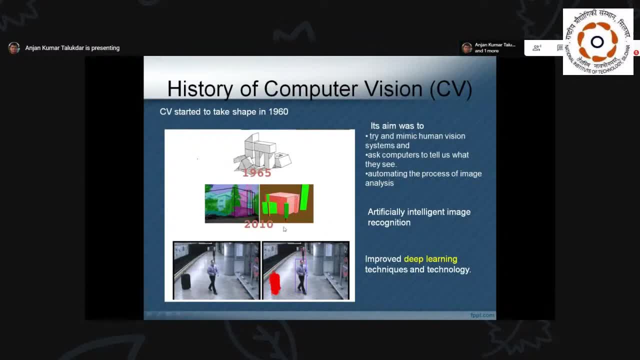 So basically these new features were added also, And then segmentation techniques were also improved. So this is how the computer vision techniques were evolving Then. nowadays this is the present situation that deep learning has come into play. So input, deep learning. 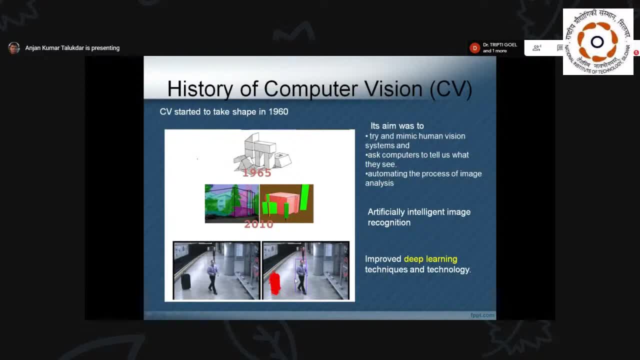 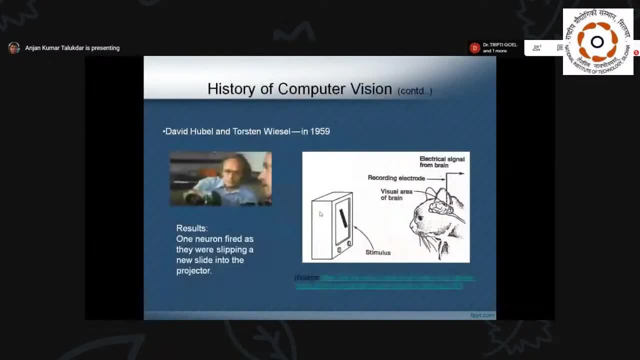 you could then uh phenomena like uh in 1959, actually how actually completely started? uh, you can say from 1959 that david google and torsten wish we sell these two. uh, professor, actually they tried one experiment on a cat. actually they placed some recording electrode on visual area of brain. 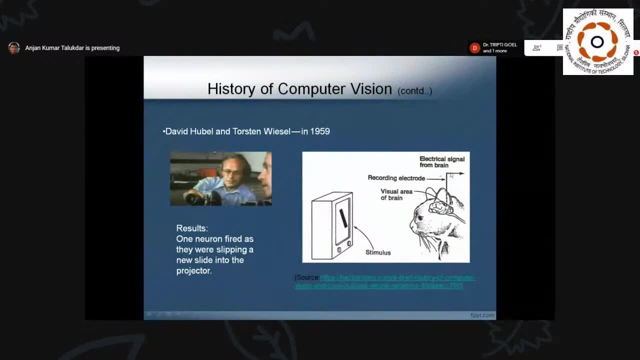 and they recorded electrical signals from the brain and actually they gave some stimulus here, like they were changing the pictures. they were giving various uh shapes here or then they record the response actually. so initially they did not get any result, but after a few months, uh, suddenly or accidentally they saw that one neuron fired as they were. 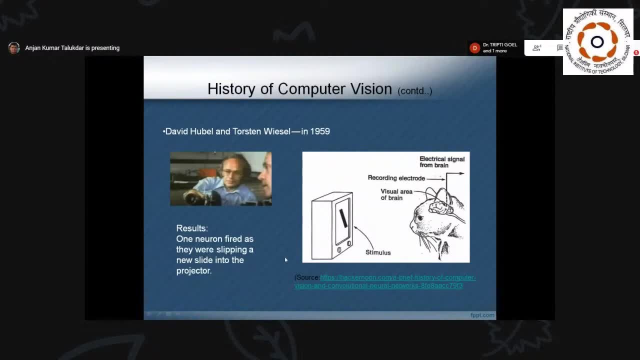 skipping a new slide into the projector. so so this is some accidental result that was observed and, and we can say, this is the starting point of uh artificial neural network or uh deep learning network that is being used nowadays. so, although it has no direct connection with computer vision, 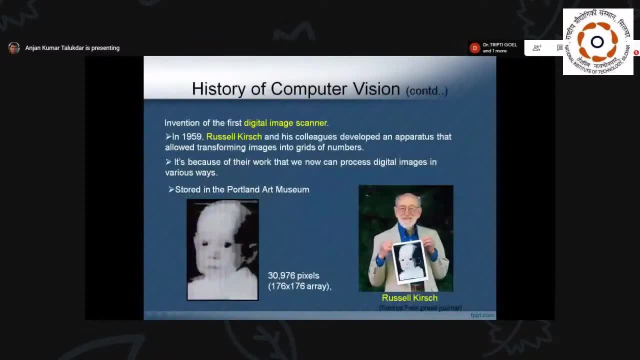 then uh, um, one major invention was that that uh digital image scanner by russell's uh kids in 1959 and his colleagues. actually he is the- uh, we can say- inventor of pixels or digital images. so it is because of there we now can process digital images in various ways. 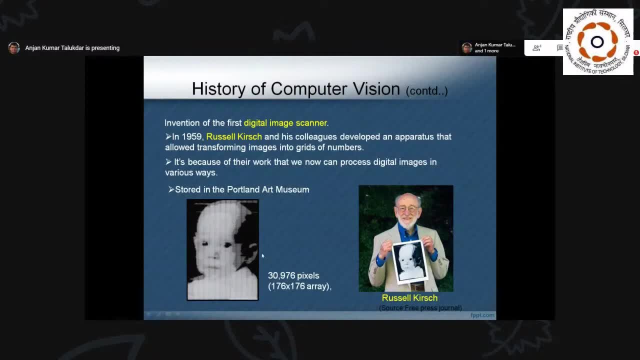 so now this is the excellent first image. that was first digital image. you can say that was uh captured, uh. it was of 30 976 pixel and his size is about 176 by 176. actually he is the uh son of sales. he was the son of russell quiz and his son russels, and russles were the son of rational piece and 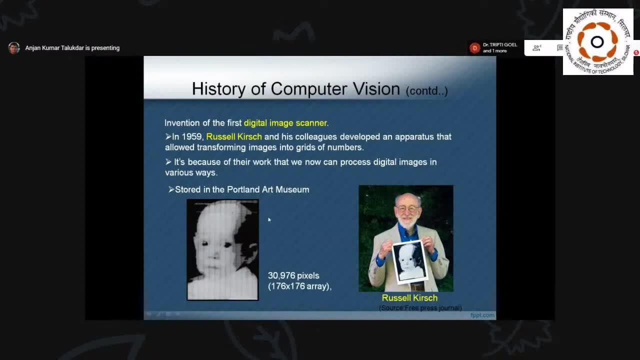 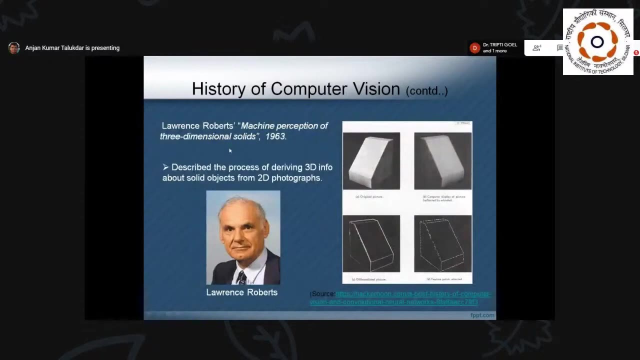 Now this image is stored in the Portland Art Museum, So this is one major invention in this field. So then, one major invention was that Lawrence Roberts this paper Machine Perception of Three-Dimensional Solids. Actually, he described the process of deriving. 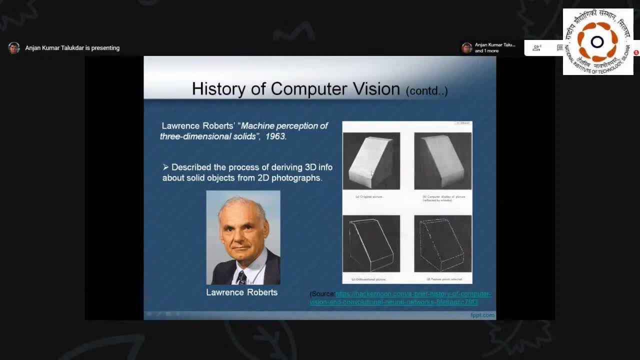 3-D information about solid objects from 2-D photographs. So what he did actually? he basically he extracted the lines from the object and then he removed the inner lines and then we got some 3-D view of the object. So this is also considered one of the major milestones. 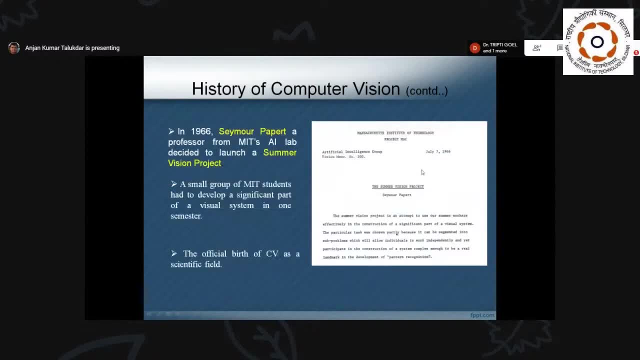 in this field. So then, actually in 1966, Seymour Pepper, a professor from MIT's AI lab, decided to launch a summer vision project. Okay, so he asked a small group of MIT students to develop a significant part of visual system. 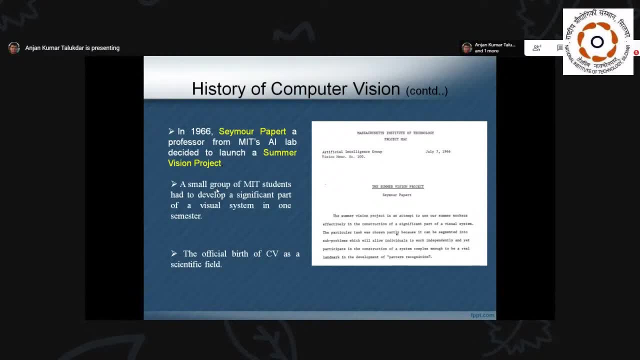 in one semester. Basically, he asked to segment the foreground object from the background and to recognize that. Okay, So, although it was not completed in the semester, but this is considered as the official part of computer vision as a scientific field, So we can say that from this project actually. 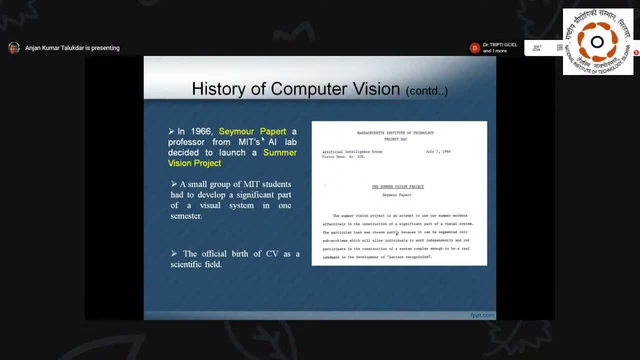 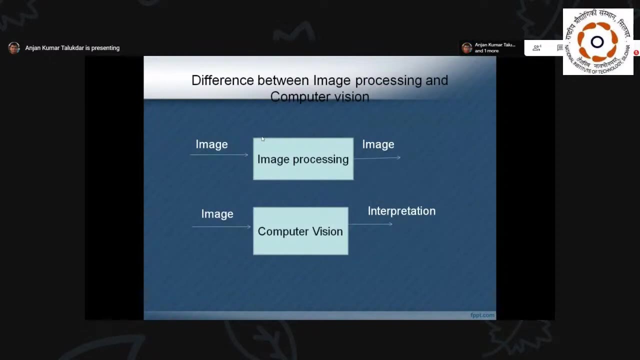 the computer vision started. So this is about brief history of computer vision. Now you might be confused. what is the difference between image processing and computer vision? So in case of image processing, our input is image and our output is also image. 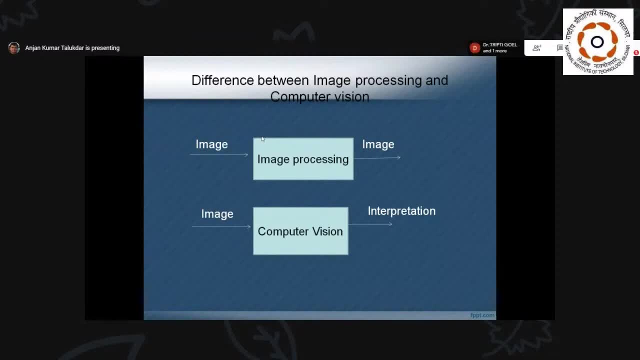 Okay, we do some processing or transformation of the input image and ultimately we get some output- image. Okay, we basically do some filtering As the name image processing. so it's input and output. both are image Okay, But in case of computer vision, 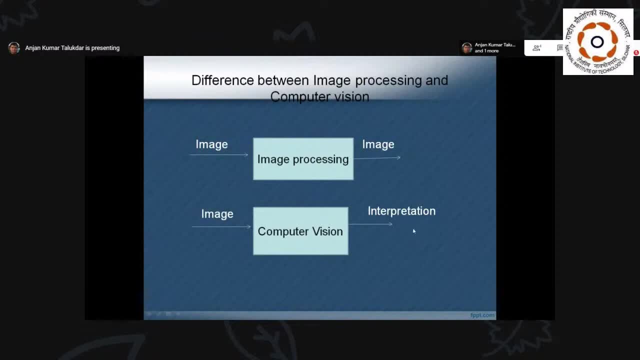 your input is image, but output is some interpretation of the image. For example, what are the objects there, What are the colors of the objects, How many objects are there, Et cetera, et cetera. So, but this image processing plays an important role. 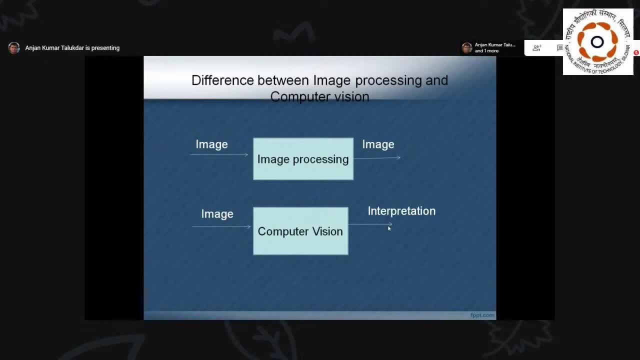 in computer vision, because to model this computer vision problem image processing helps a lot. So we can say image processing is a part of the whole computer vision system. So till now I have talked about what is computer vision, briefly about computer vision, its applications. 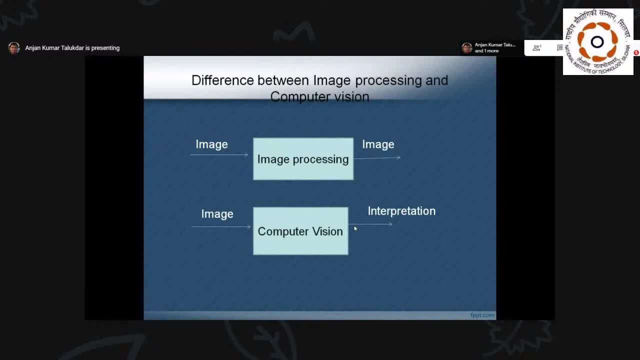 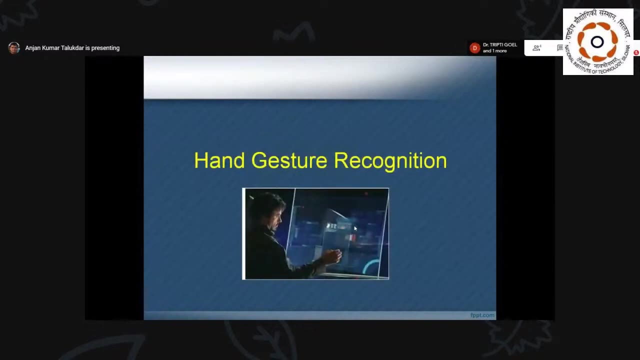 and a brief history of also computer vision and a comparison between image processing and computer vision. So this is about computer vision. Now I'm going to discuss an application of computer vision, that is, hand gesture recognition. So what is a gesture of three? 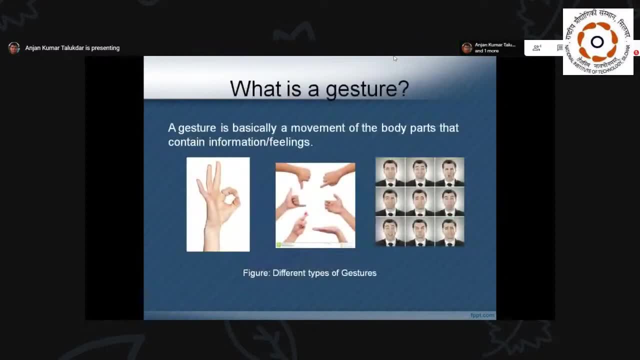 So a gesture is basically a movement of the body parts that contain information and feelings. okay, So a gesture's basically the movement of the body parts that contain information and feelings. okay, So we always, in our day-to-day life also, we use our gestures to convey some information, right? 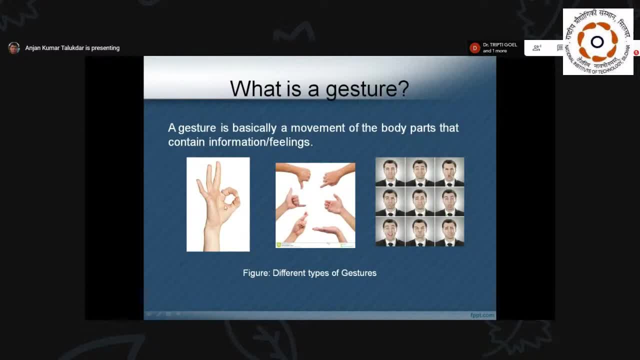 So this is basically gesture. You can see some hand gestures here and also the right hand side. you can see some facial gestures. We express some of our feelings, our emotions, through our facial expressions also, So this is also one type of gesture. 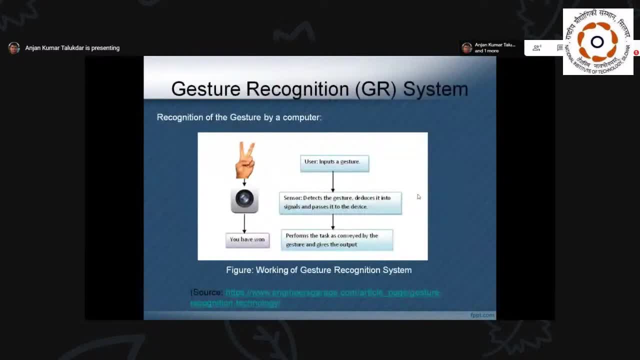 Now, what is gesture recognition basically? So gesture recognition is the recognition or the understanding of the gesture by a computer or a machine. So this is basically the gesture recognition. So in case of gesture recognition, our input is a gesture which is given to us. 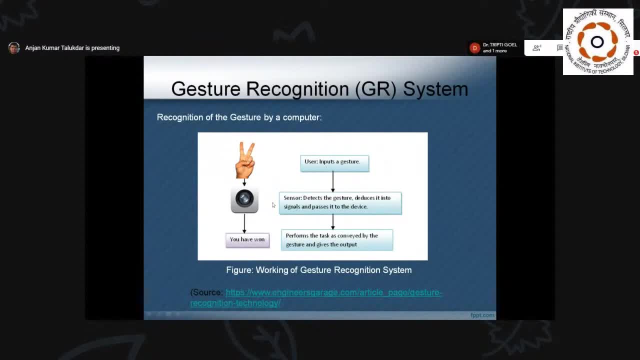 It is given by the user. Then our sensor, basically the camera, detects the gesture, reduces it into signals and passes it to the device. So then the processing device processes these signals and performs the task as conveyed by the gesture and gives the output. 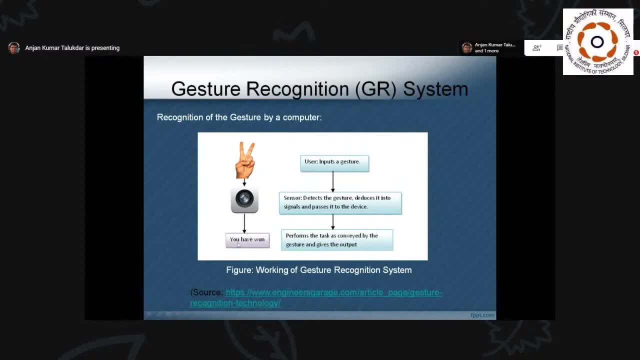 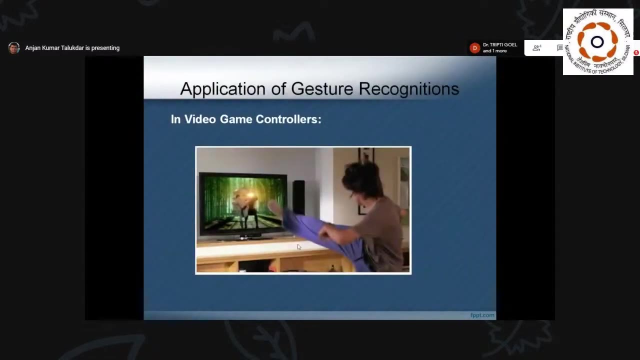 So it will interpret as this sign, suppose Gesture that you have owned. So this is basically the working of the gesture recognition system. Now applications of gesture recognition. It has many applications nowadays. First of all, suppose, in video game controller. 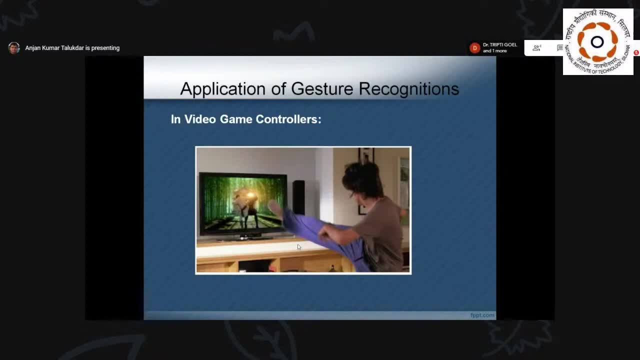 So nowadays smart TVs and smart cameras are coming. For example, Microsoft Xbox is a nice example. It uses one camera called Kinect sensor. I will show it later part. So here what happens: You can directly actually interact with the game or the player. 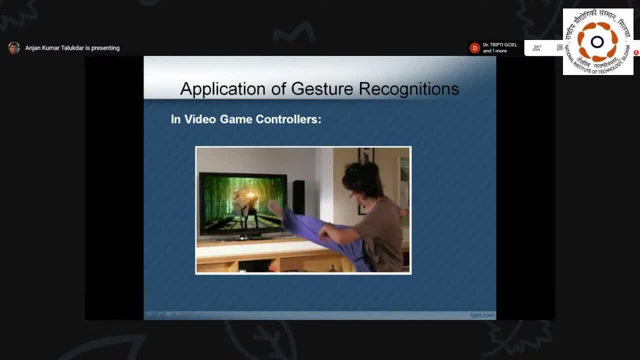 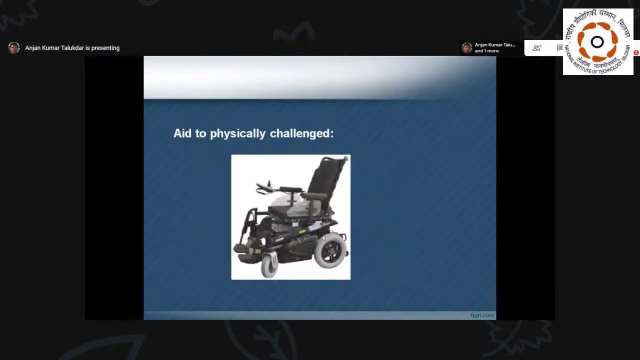 So suppose you are kicking, then this player will also kick. So like that, In real time you can directly interact with the game. Okay, So this one application in video game controllers, Then aid to physically challenged, So the people who have some motor neuron problems or some who are visually impaired. 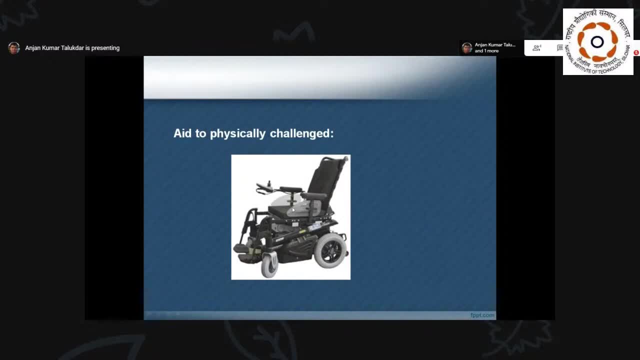 So they can use this actually chair. Okay, So basically here, Sensors are there, So with the help of your hand gesture we can control this chair. So, speed direction, So everything is controlled just by one hand gesture or finger movement. 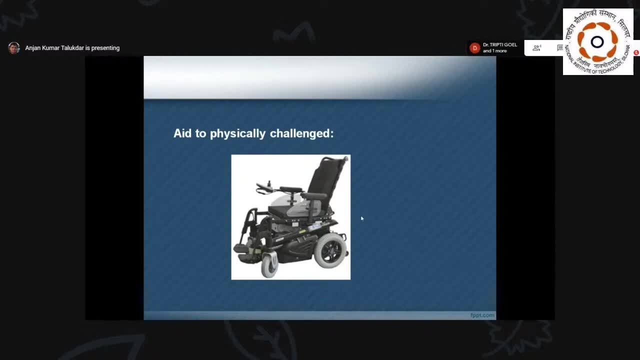 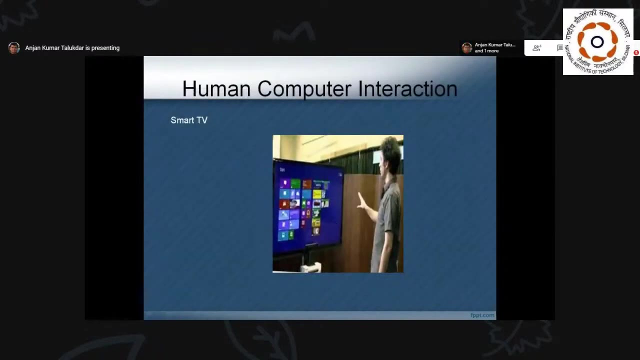 So this one example. Then human computer interaction. Now smart TVs are coming to the market where, with the help of your gesture, you can control your TV. So no remote is required. Your hand is your remote actually. So that is also coming nowadays in smart TVs. 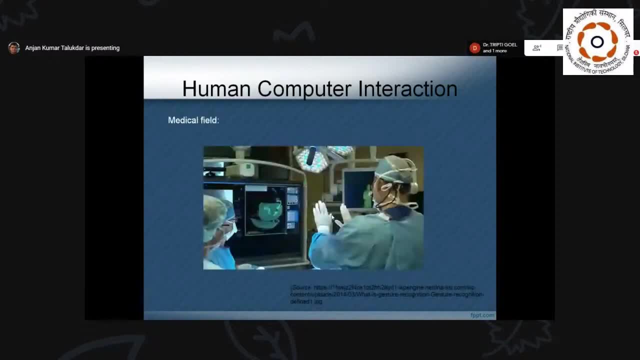 Then in case of medical field also, it has many applications. For example, suppose a doctor is doing some operation So he is wearing gloves So he can't touch the machine, But he has to control the machine to see some images, or like that. 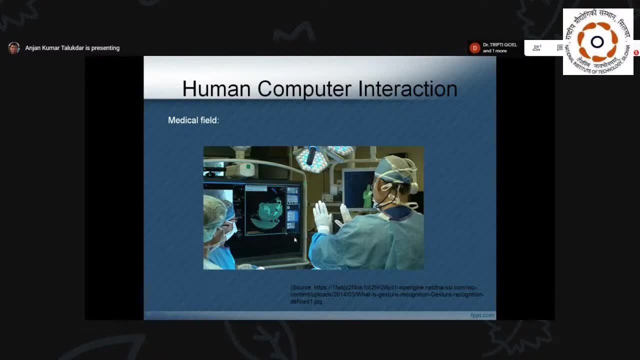 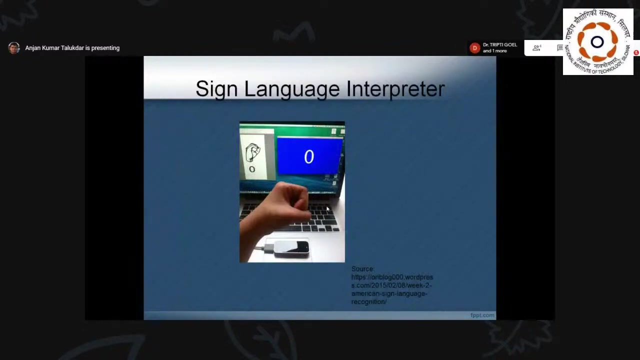 So, without touching this machine, with the help of gestures, he or she can control this machine. So it is playing a very important role in case of surgery or medical field Medical applications, Then sign language interpreter. So this is also one very important application of gesture recognition system. 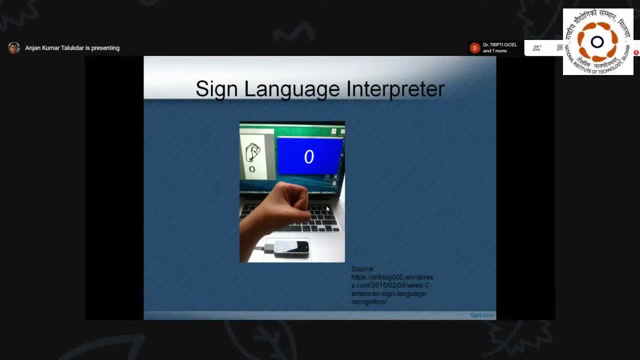 Sign language recognition. So what is sign language? basically, Sign language is the language used by deaf and dumb people. So many of us don't know sign language. Only those hearing impaired people know sign language and they communicate among them. But to communicate with hearing impaired people, by healthy people like us, so we have to learn sign language. 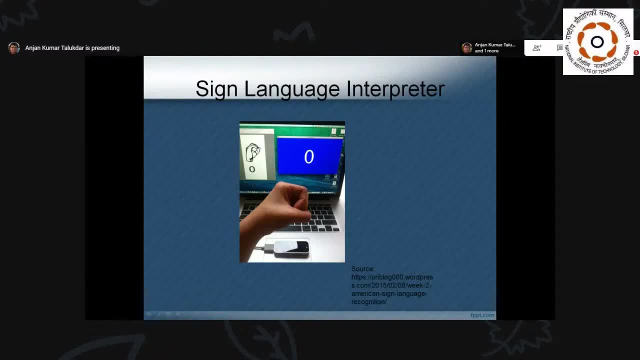 But it is very difficult to learn sign language also. So in that case the sign language interpreter can help us. It can convert the sign language into some audible text or speech signal which is understood by one healthy people, or vice versa. So in that case, the sign language interpreter is actually bridging the gap between the hearing impaired people and the healthy people. 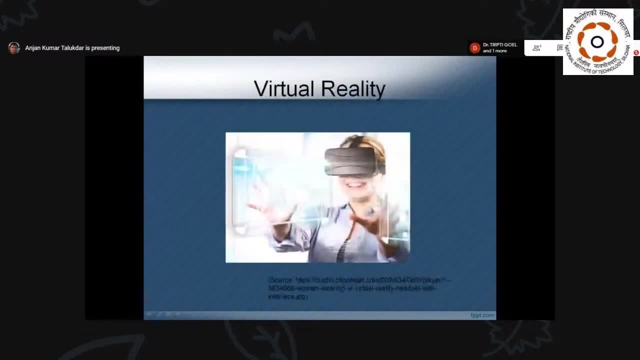 Then what is sign language recognition? Then, one more important field is the virtual reality. So, as Nam suggests, a virtual environment is actually built surrounding the user or surrounding us, But it seems to be real, So we can directly interact with this virtual environment. 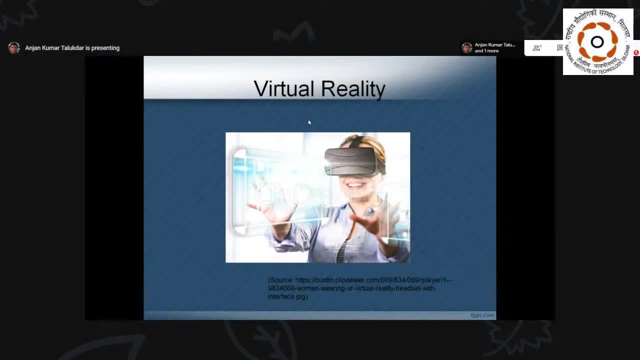 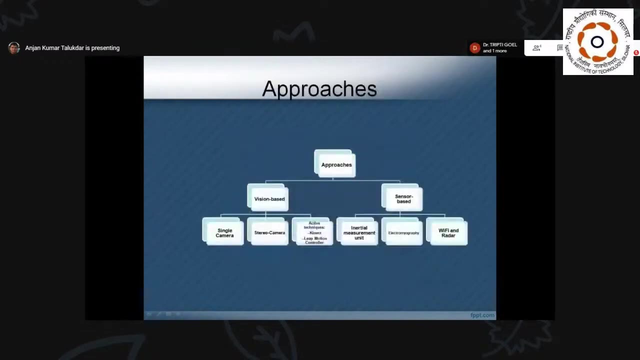 So I think you are familiar with this virtual reality. So this is also becoming possible only because of the hand gesture recognition system. Now what are the approaches for hand gesture recognition system or the sensing technologies that are used? So there can be two approaches. 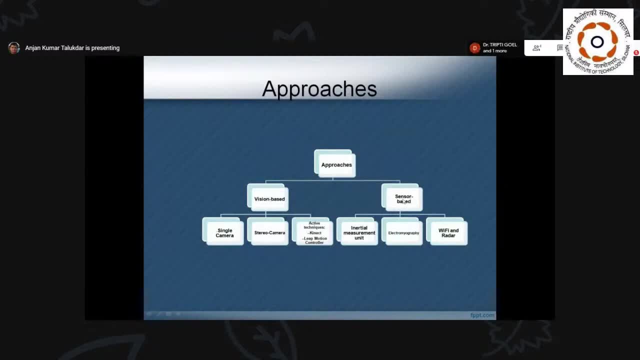 For example, one can be your vision-based and sensor-based. So in case of vision-based, basically the cameras are used Okay, And so we can use a single camera, or we can use a stereo camera having two cameras. 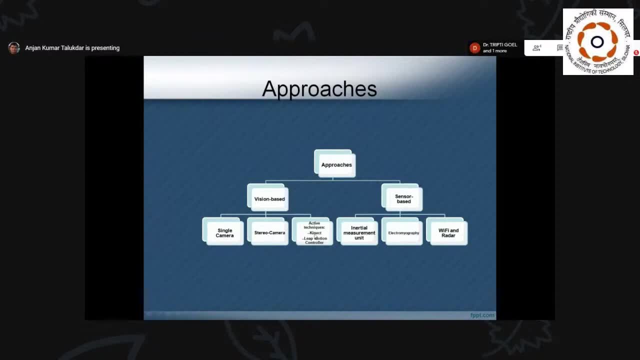 And then we can also use some techniques which uses some IR sensors also along with the camera, RGB camera like Kinect or motion controller, etc. And in case of sensor-based, actually we can use some inertial measurement unit-based sensors or electromyography or EMG signal-based sensor or Wi-Fi or other field-based sensor. 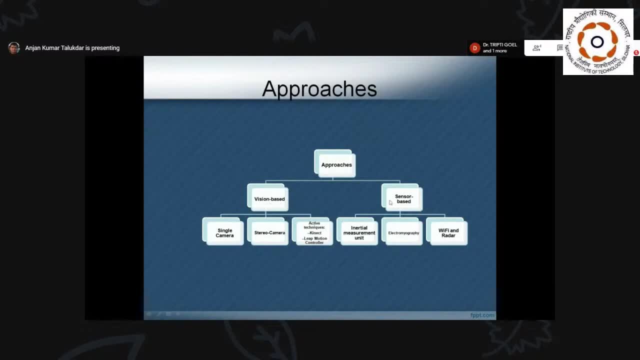 But if you compare these two- vision-based and sensor-based- actually accuracy in case of sensor-based approaches are more compared to vision-based. But the problem is that the user has to wear the sensor or the globe on his or her hand, So it is difficult to move the hand freely. 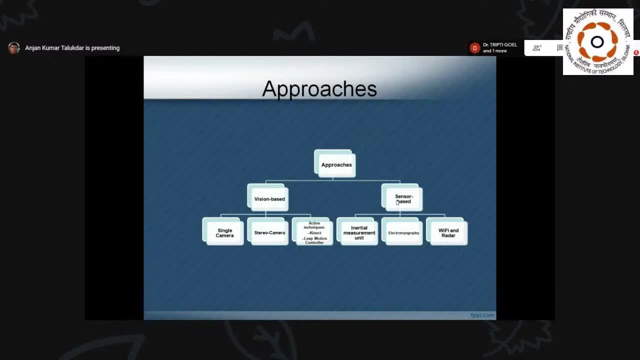 This is one drawback: If you wear this sensor, then it is difficult to do the free movement And also they are costly also. These sensors are very costly also, But in case of vision-based, you can freely move your hand And they are less costly also. 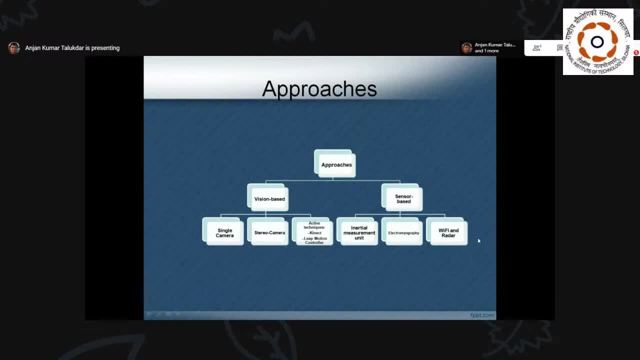 But accuracy is more in case of sensor-based, Basically in sensor-based. So in case of vision-based, we can use single RGB web camera like this, But we should not use a camera with very high resolution. We should use a camera with medium resolution, not very high. 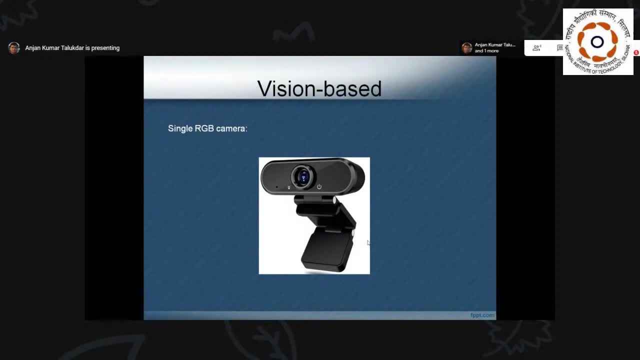 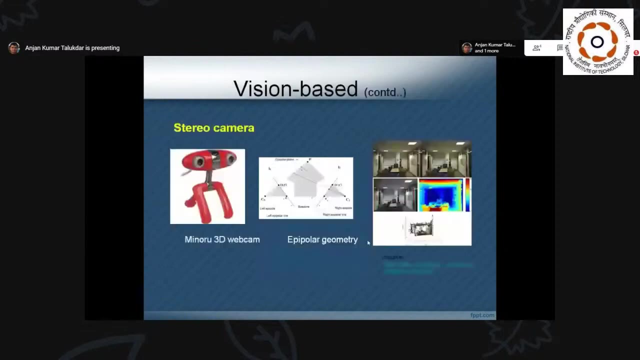 Because if your resolution is very high, image size will be more And the processing algorithms will take much time to process your images. So that is why we should use some images with some low or medium resolution. Then we can. But in case of single RGB camera, 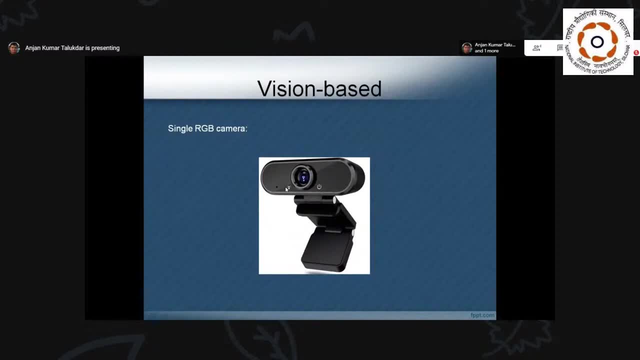 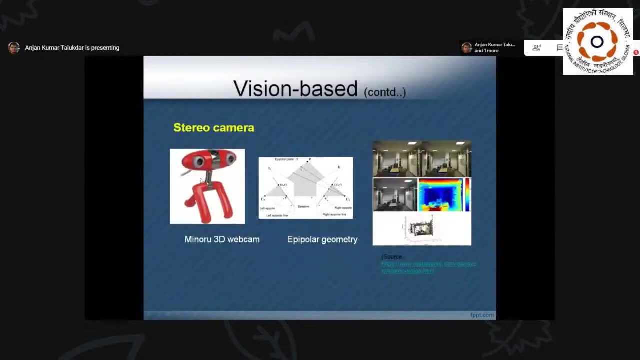 we only get two-dimensional information or 2D image, But if you go for stereo, camera means two cameras at a time, so you can extract that 3D information also. So this is one Miniro 3D webcam we can see. 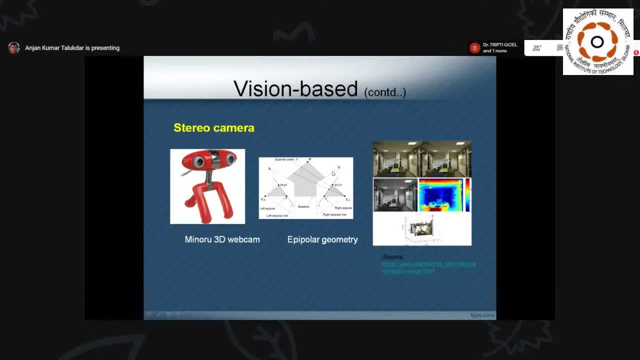 So, So this, actually this is a molecular geometry which is used to represent this stereo camera And using this technique, actually, we can find the third information, That means the depth information from these two cameras. This is the depth information. 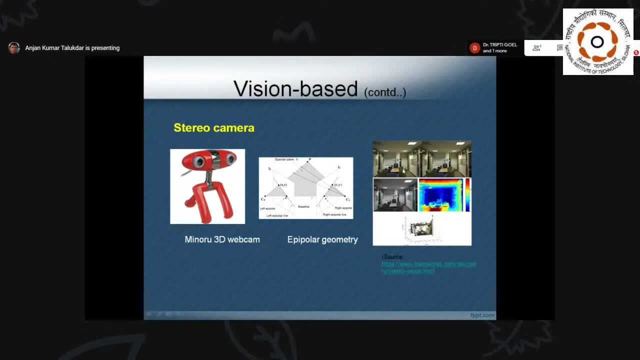 So we can extract this depth information. For example, suppose this is one same scene. This is captured by left image, This is captured by right image And this is actually the disparity map, which is giving you the information about the depth. 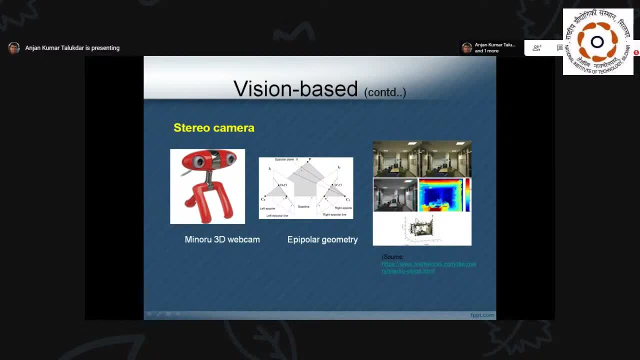 And this is a 3D projection of this depth image. So means, with the help of stereo camera, we can not only extract that 2D information, but also depth information or the 3D information. Then one more camera is there. 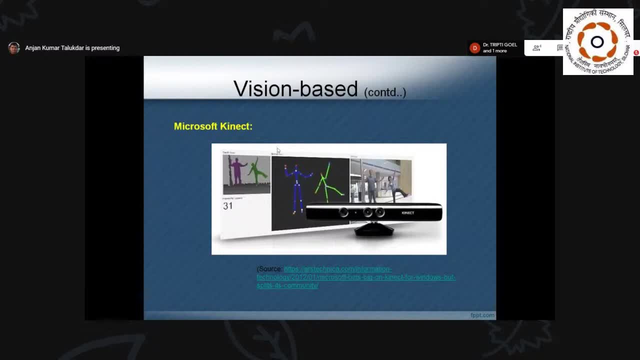 This is called Microsoft Kinect, As I would like tofish this Kinect also works. But what is the advantage of Kinect sensor is In Kinect sensor there are two cameras. along with this, one IR sensor is also there, This dish IR sensor actually. 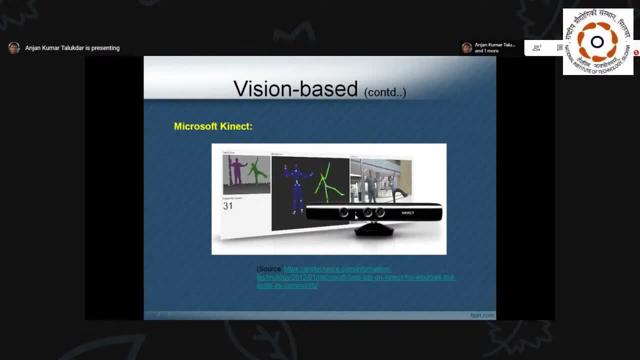 if it takes z information also. so it basically gives three outputs. first one is that you can easily draw the skeleton of the object. suppose this is your rgb image and these are the skeletons of these two people. so skeleton information is easily extracted and this is the depth information. 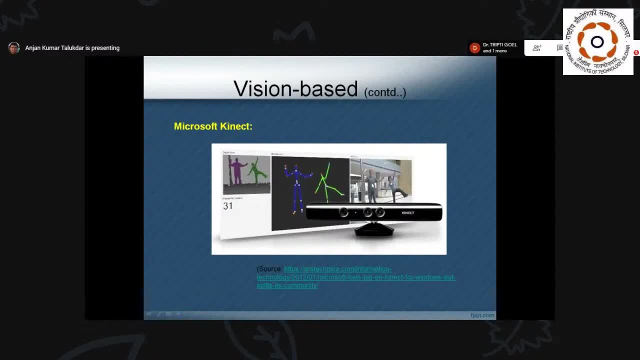 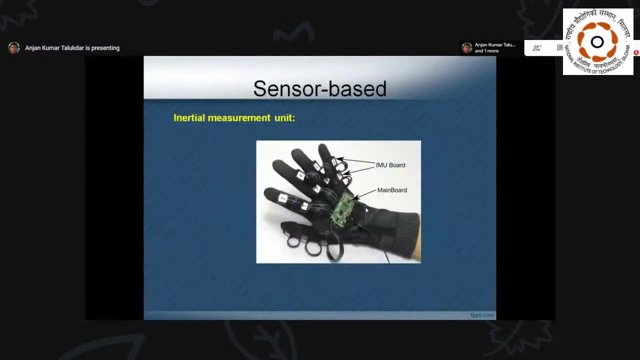 itself, so we can have the depth information also means which person is nearer to this camera, which is uh far from this camera, so we can easily determine that then. uh yeah, sensor base, that is, inertial measurement, image based sensor support. so this is one uh image of this kind. 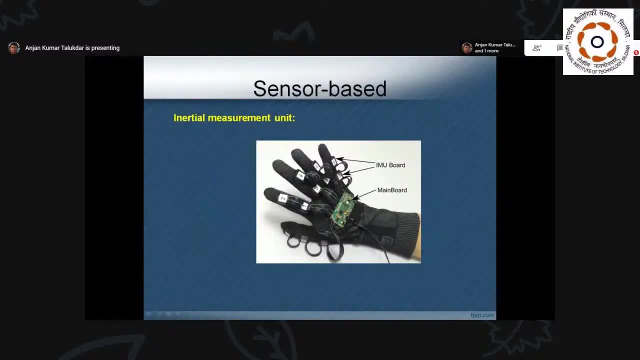 of sensor, basically these sensors, uh, these sensors determine basically the angle information between the joint angles of the fingers, uh, etc. also to determine a movement of the fingers, like acceleration velocity, uh, angle movements etc. so that's why, uh, they are very uh accurate but they are costly. 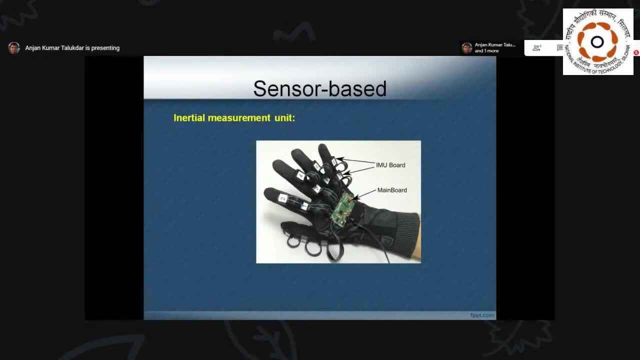 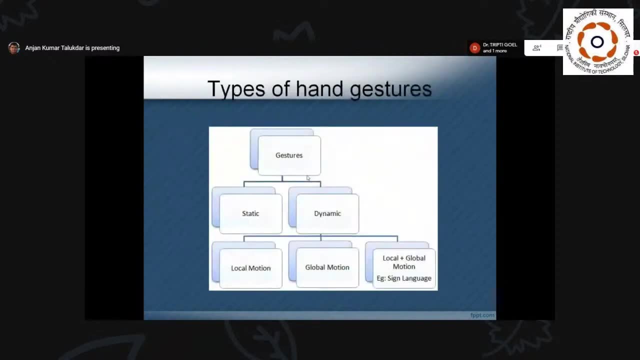 so these are the various uh sensing devices that are used for and what are types of hand gestures now. so so, basically, uh gestures are two types. you can say one is static and dynamic. so in static gesture, what happens? that your hand or your finger fingers are static? but in case of that, 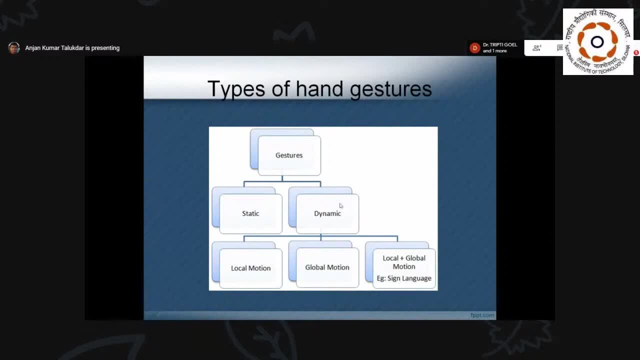 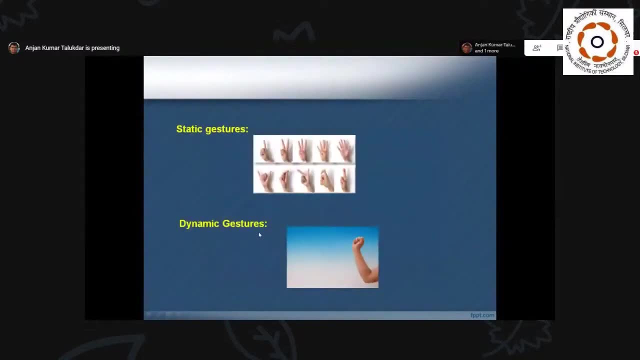 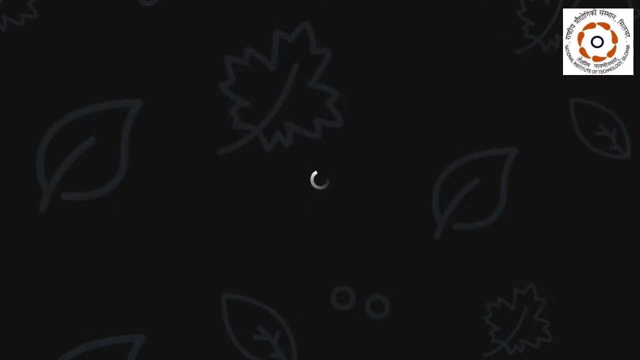 there's a movement of the hand or fingers, so this figure will show you there's. these are aesthetic gestures and this is your dynamic gestures, where the hand or the fingers, they are actually moving me. there's a global motion of that movement. uh, so your fingers are moving. i suppose you can watch your hand, Jerris. 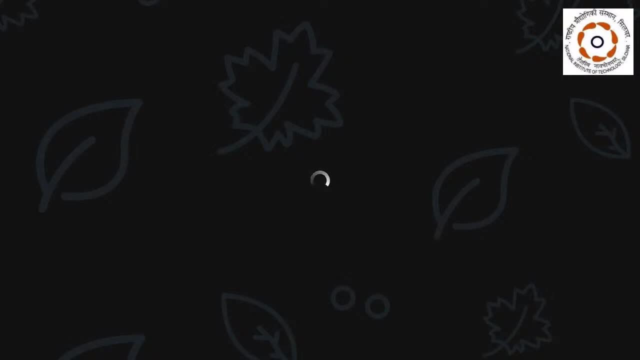 started to walk like that you can move your fingers right the same way also, like after going parallel. just like you're Jacob, and now you can see FA whichbau Z bal Heil are two Hi-With unserer body. die stand die die? no, is not the body. 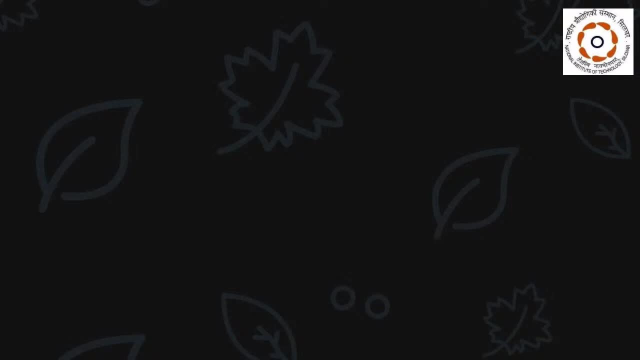 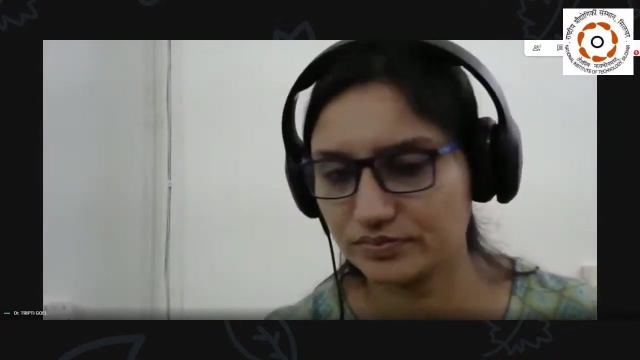 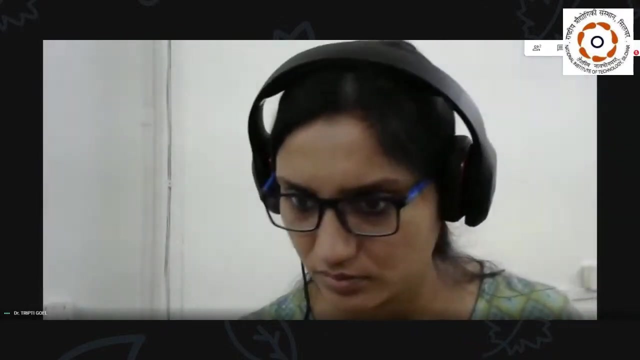 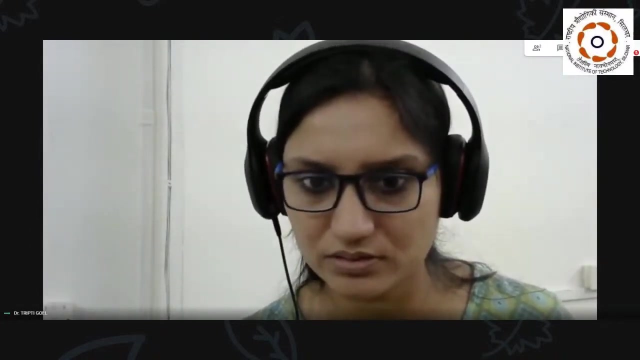 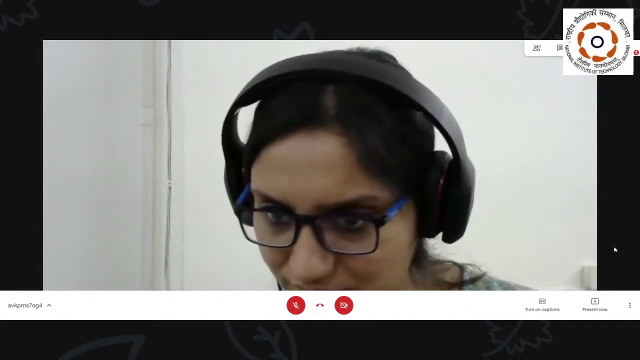 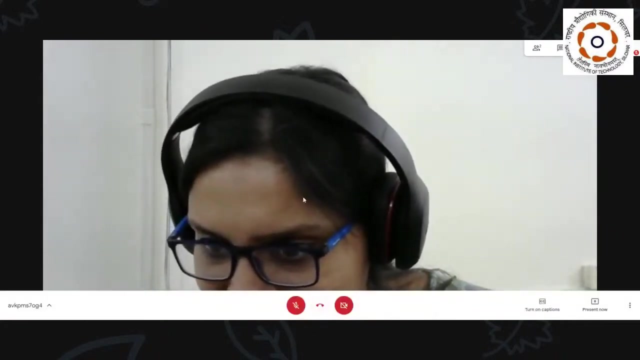 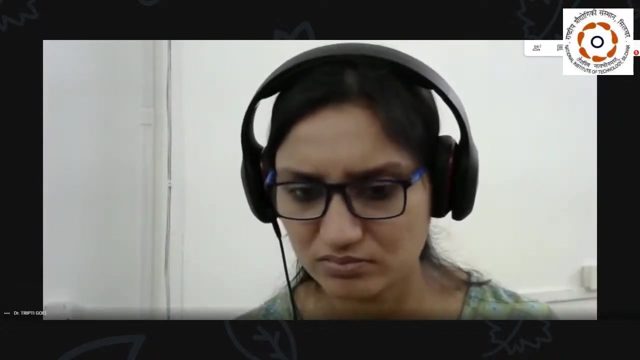 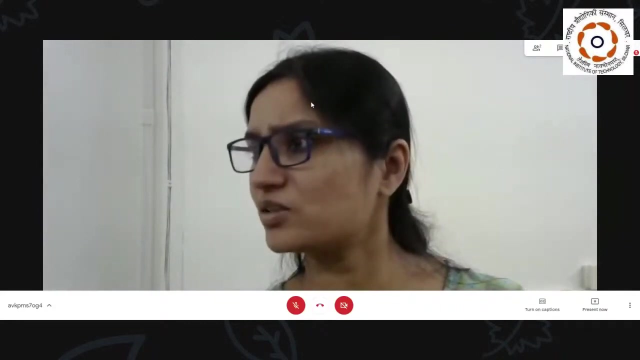 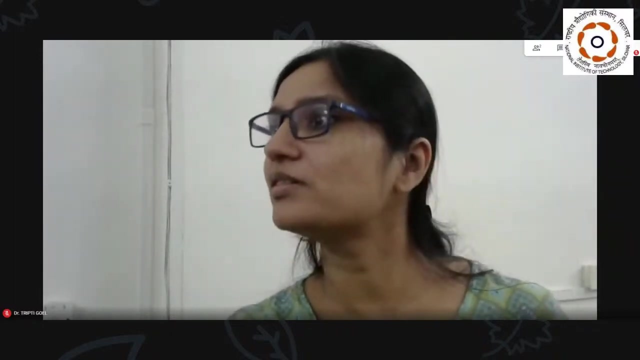 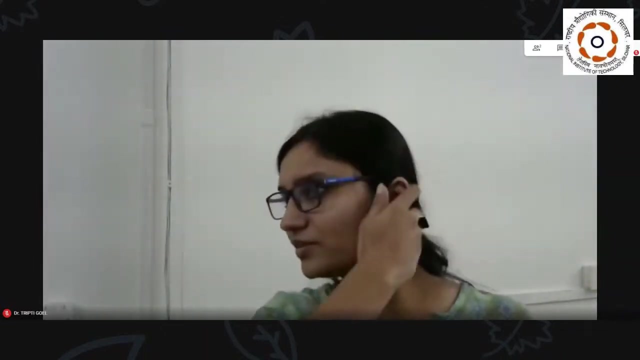 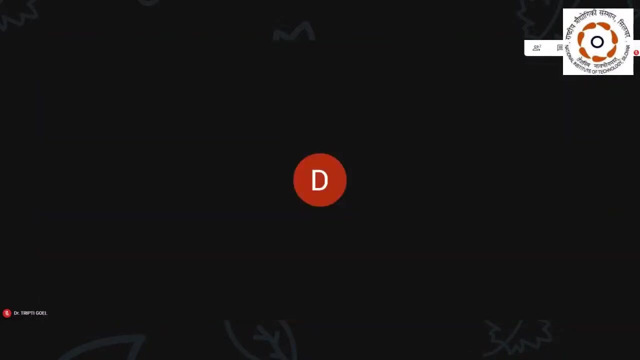 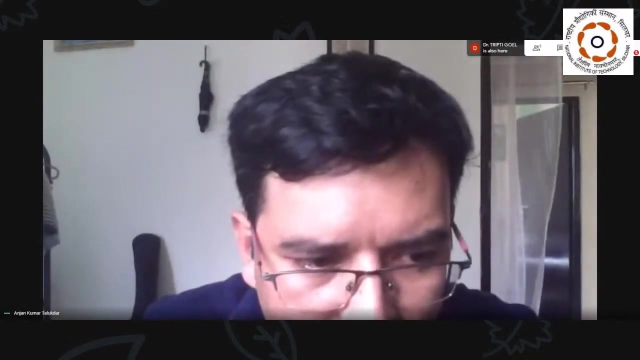 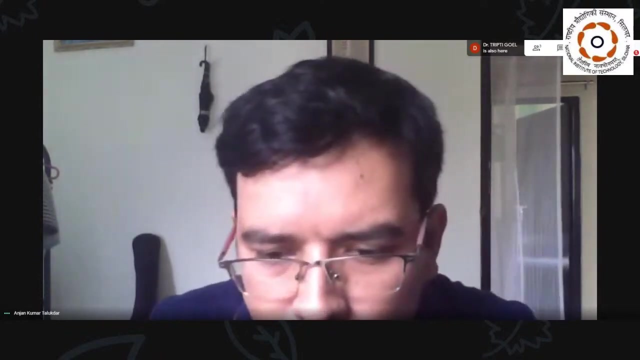 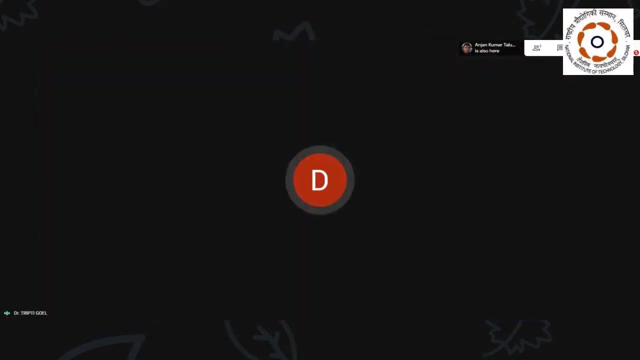 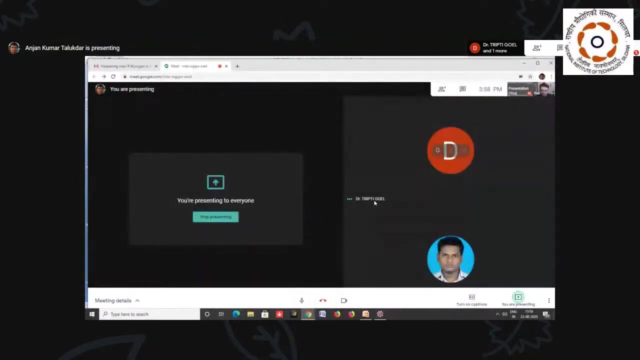 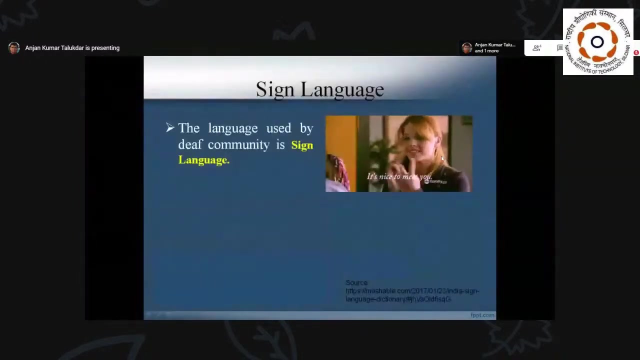 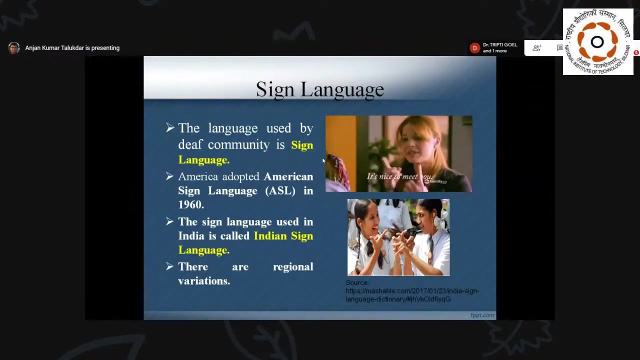 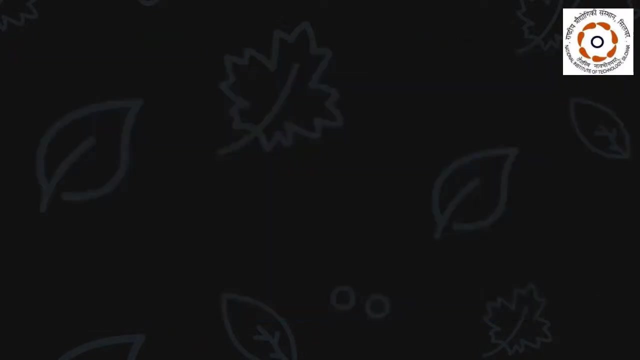 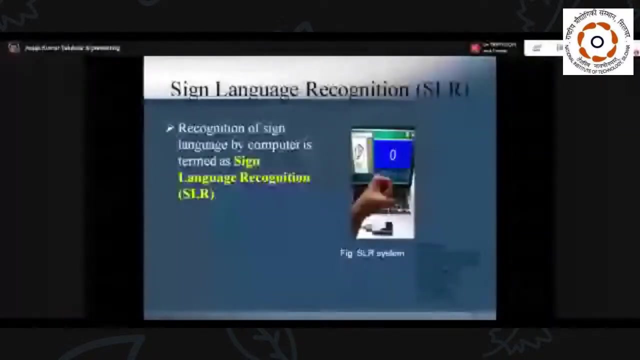 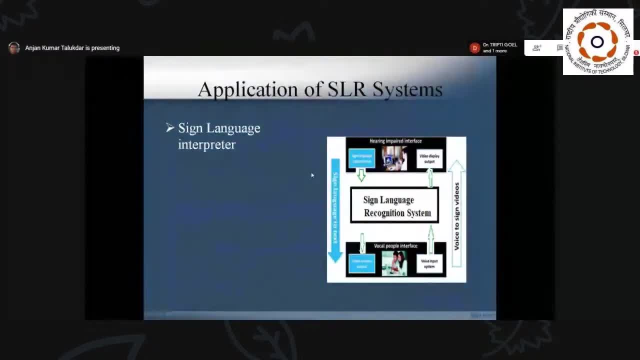 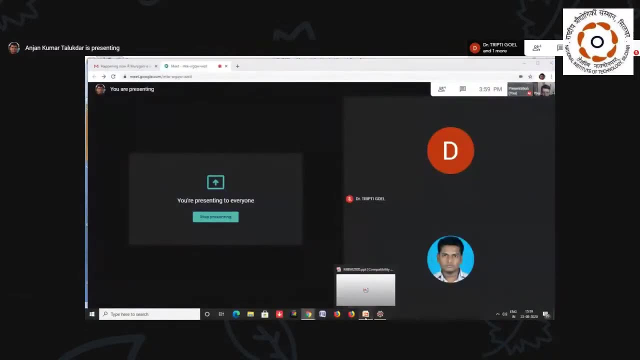 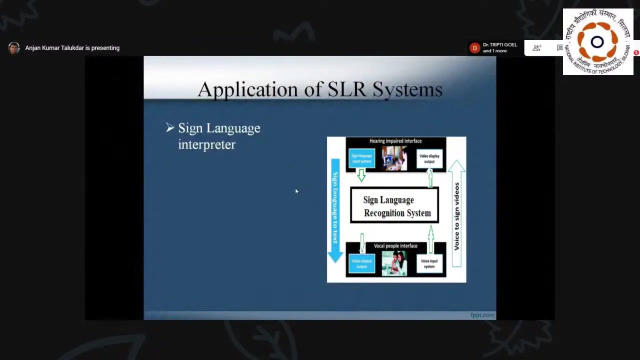 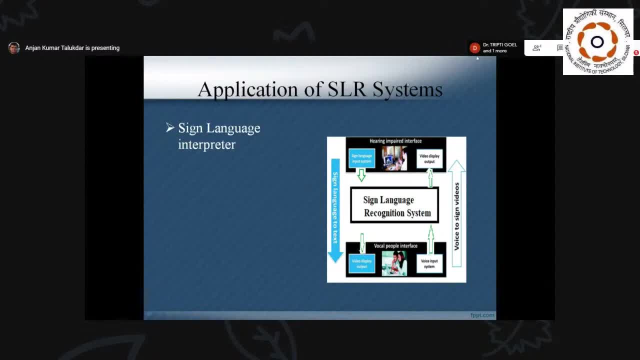 okay. so, as i have already told that, our healthy people generally find it difficult to communicate with hearing impaired people through sign language because they don't know sign language. so if there is one sign language interpreter, so with the help of that sign language interpreter we can communicate with them also, and it can be. 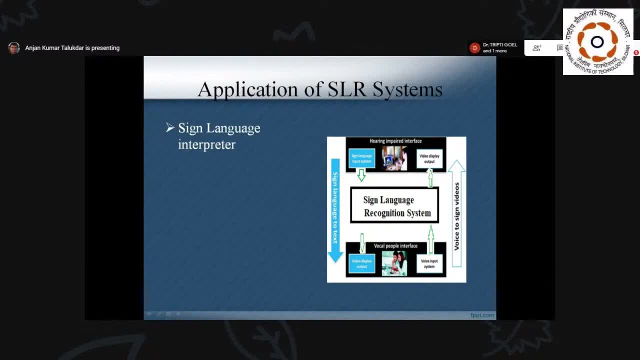 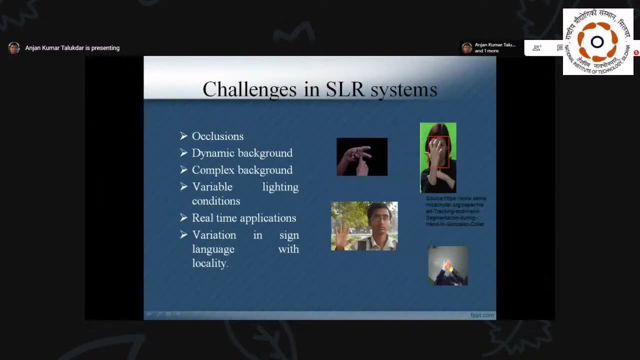 placed in various places like airports, always banks, etc. etc. so, um, so, it can uh bridge the gap between a hearing impaired and healthy people. now challenges in sign language recognition systems. so there are many challenges that come in sign language ecosystem system. some of them are like occlusions. so what is occlusion basically? 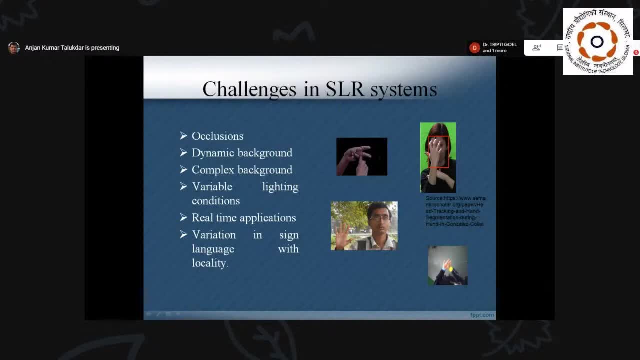 when one body part comes about the other body part. that is called occlusion. as you can see here, this hand or this pump part is coming above this face part. so this is one occlusion problem. similarly, here also you can see this uh, this finger, your uh is coming, is on above this, uh. 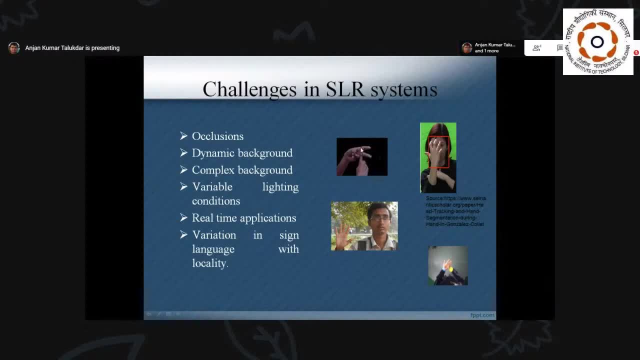 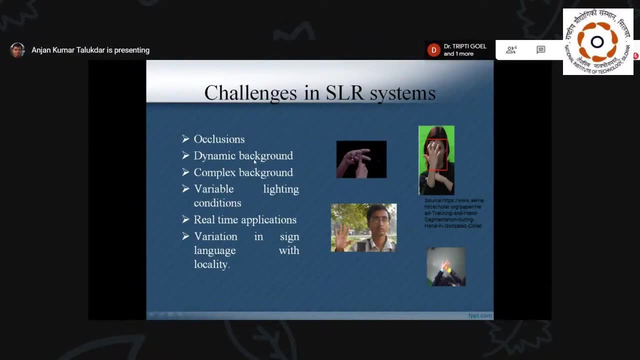 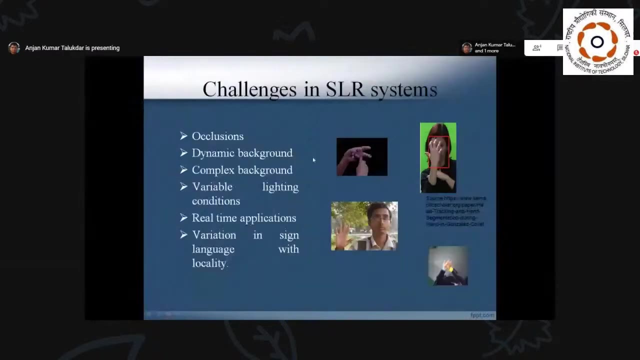 palm. so this is this index finger finger is coming above this palm. so, uh, this is occlusion problem. all right, so we will talk a little bit more about occlusion. some of the most common problems, um can be affected by occlusion also. that is basically this problem. 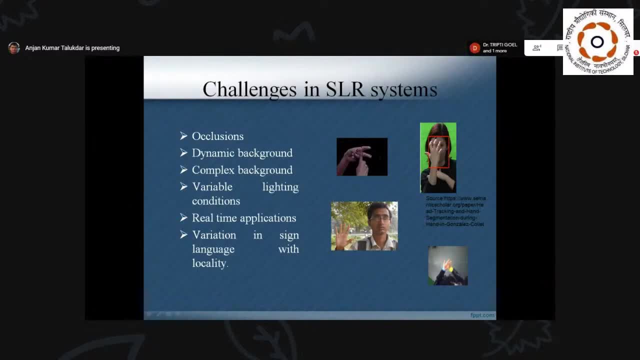 occlusion problem. so if the person has or, uh, if you have a courage, or if you have a desire or desire to go into occlusion, so this is also a problem to deal with, when you have a courage to go into occlusion. and this is where occlusion becomes very dangerous. 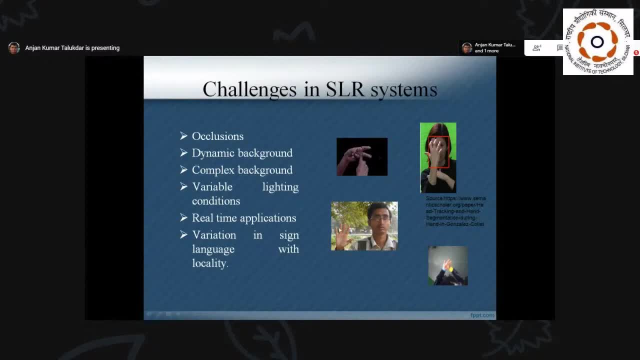 and it's also very difficult to practically move our attention to this background and you're not allowed to experience the specific background. so if your background is moving, suppose part or the palm or hand part, so this, this is one major problem. there's complex background, then variable lightning condition. as you can see here, the lightning condition may be varying. 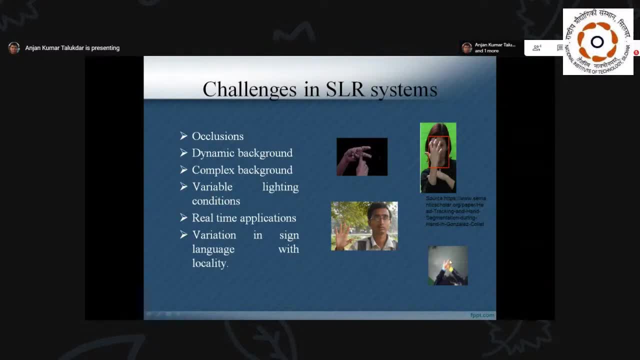 if sometime it may be darker, suddenly it may be brighter, so so it is very difficult to basically segment the hand part from the background for the variation of lightning conditions. then a real-time application. so what is real-time application means your recognition should be very fast. you have to recognize a sign before the next sign is entered. so it's. 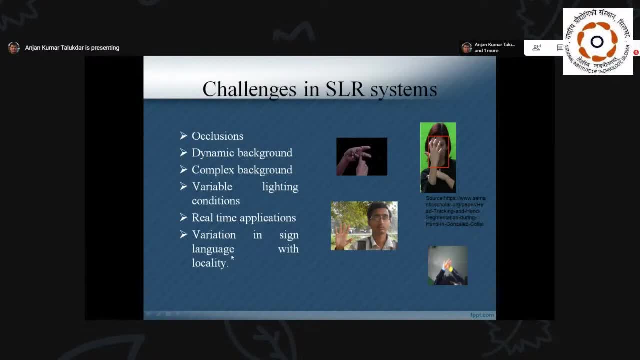 very fast. then also one more problem is there. it is called variation in sign language with locality. it means the sign language that is used, suppose, in Delhi. that language may not be used in Mumbai also, so there may be some variation. so there is also one problem in indian sign language system. 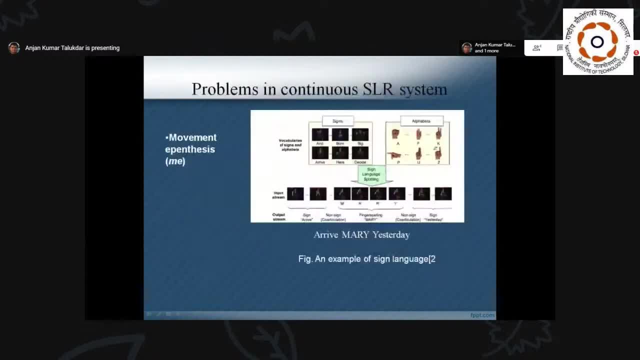 so, apart from this, if you consider more problems in continuous sign language recognition system. so sign languages can be two types: one can be your static, another so the isolated, another can be your continuous. so in case of isolated sign language, we use one single sign at a time, but in case of continuous sign language, 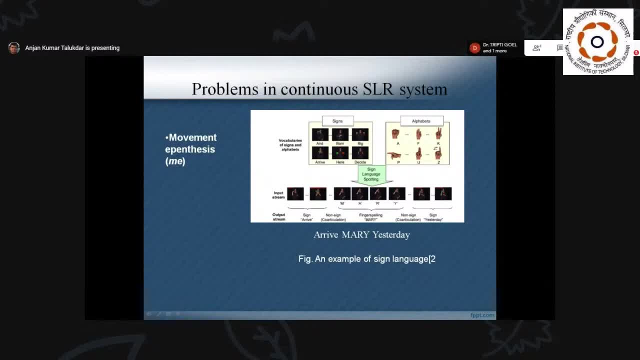 for example, in case of sentence, one sign is followed by other other signs in single video. so it means there is a continuous sequences of signs. that is the continuous sign language is your anyways, so you continue. scene language, so say assign language, consist of these two parts: finger spelling and the 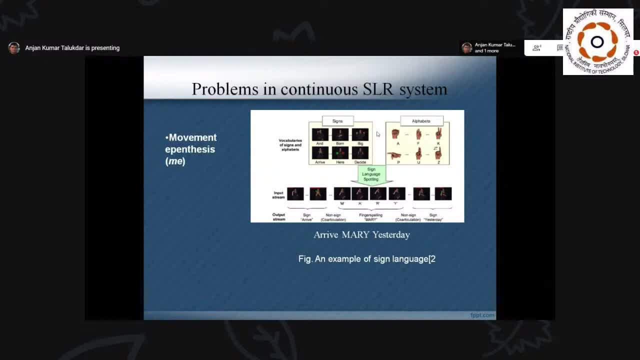 sign. so what are fingers filling? finger spellings are the. you are basically the static signs, as you can see here, the alphabets for alphabet, strategic signs or fingerspins like a f, okay, for the, all the 16 alphabets, except uh, z and j, all are static. but and what else? uh? 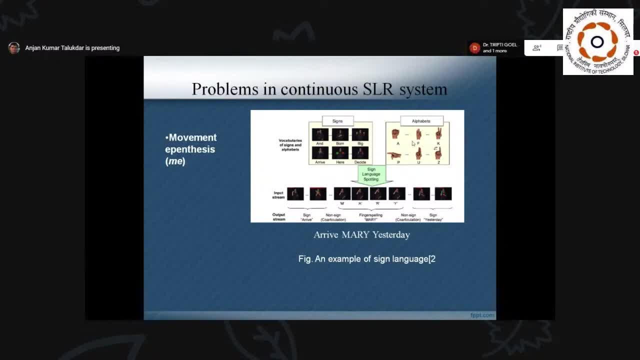 so these finger spellings are used basically to articulate and suppose name of place or name of the person, etc. for which actually no particular vocabulary is out there. but in uh and signs are the actually uh sign language for uh? which actually uh vocabularies are there? which some dictionary is there only there? for example this: 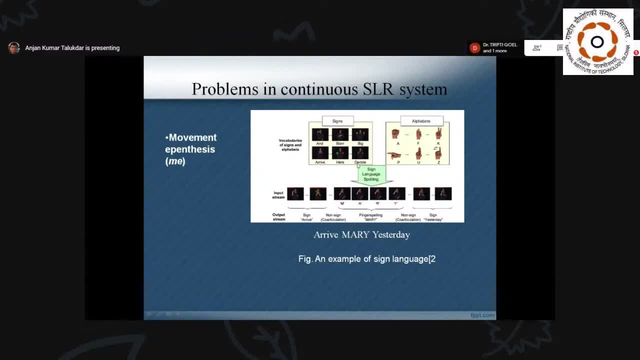 suppose uh and big arrive here. so these are signs with some vocabulary. okay, so now a complete sign may con language may contain uh, the mixing of both. for example, if you write one sentence like arrive, mary yesterday, so for arrive and mary there are uh predefined uh signs, but for mary we have to um spell each of the letter one by one: m a, r, y, because this is a. 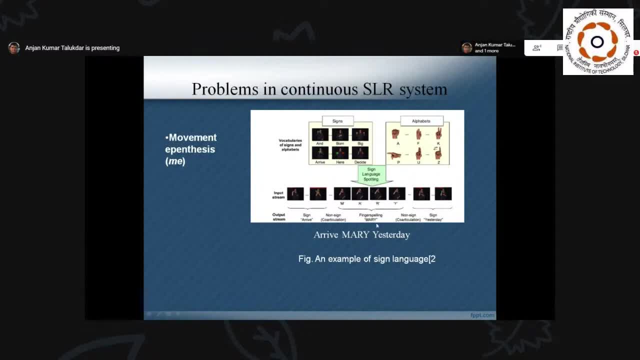 proper noun and there is no particular dictionary for it. so now, what is the problem in this continual sign language information? that uh, one problem is called movement. appendix is: uh, there is a lot of soy in uh. uh, that tentang movement in anoraoma obj. now, what is movement ap Liveren problem basically, uh, when we move from one sign to other side. so 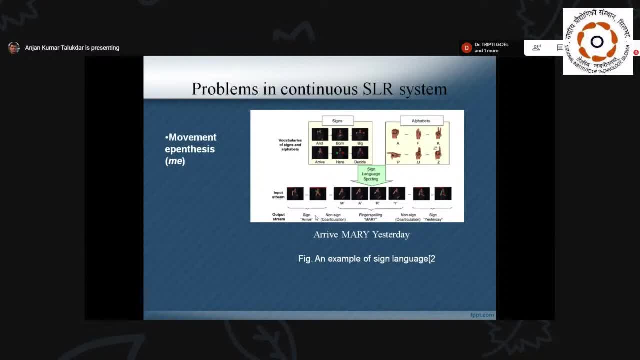 there is a joining part, means some extra movement of the hand from one position to other position, means from the, the x-ray signs as they have arisen because of the continuous sign language and so, and second problem is the co-articulation. so what is co-articulation problem basically? 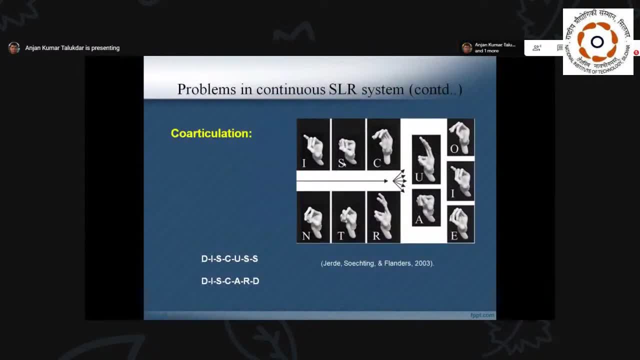 the one problem there is: what, what, what, that is, the articulation of the current sign is uh affected by its previous as well as its uh future sign. okay, and so, of course, uh, this is our s is the current sign. so the articulation or shape of this uh sign, uh, in case of uh continuous case, 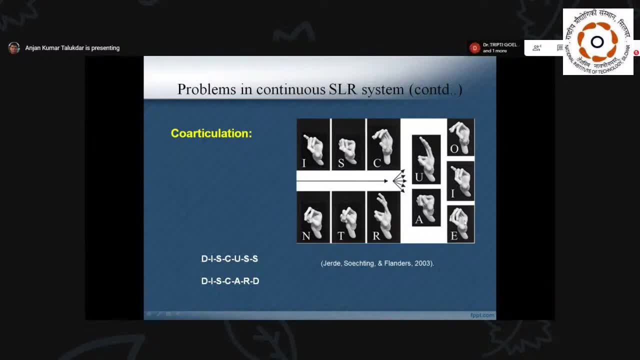 will be different from its isolated uh case. okay, its shape will be varying from its isolated case because of the effects of this uh previous sign as well as of the next sign. so also there are two problems basically, one is called assimilation and dissimulation problem. suppose, yeah, in case, suppose. here you can see. 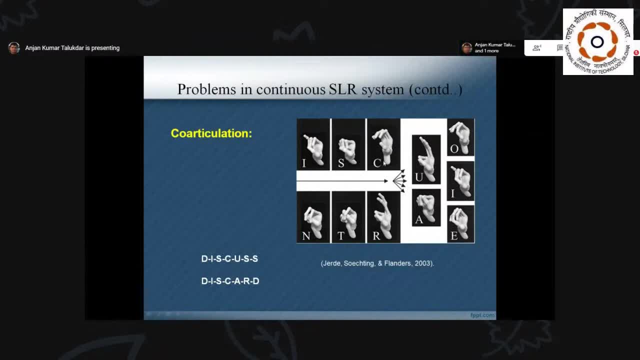 the suppose uh c, this letter c and this letter a, uh, they are almost uh similar, they have similarity, so, or so what happens? if uh c is followed by a, then uh, articulation of s will be affected by this because they are similar. but if uh, uh c is followed by u, uh, then uh effect on this articulation. 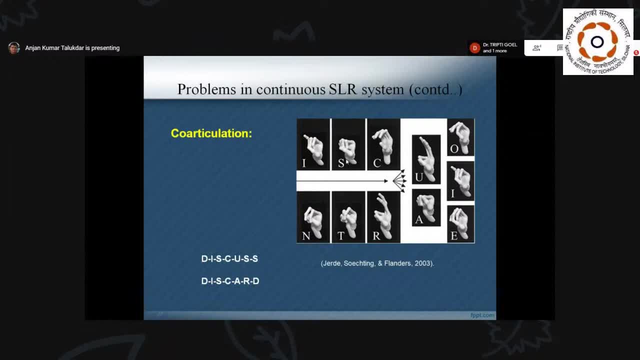 uh will be uh different. so this is one major problem. in case of uh continuous sign language, for example, suppose uh, there are two uh words. one is discussed and discard. so in case of uh, discuss, s is uh, sorry, c is followed by u okay, and in case of disgrad, c is followed by a. so here you can see, c is followed by u and c is. 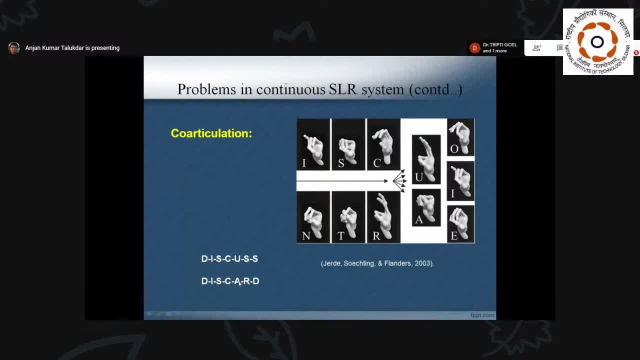 used by a. so in both this uh cases, the articulation of the letter s will be different. because of this problem before to, because of this case, we are performing just that. the picture what's happening, have already told, is assimilation and dissimulation. this is assimilation problem. that is because they 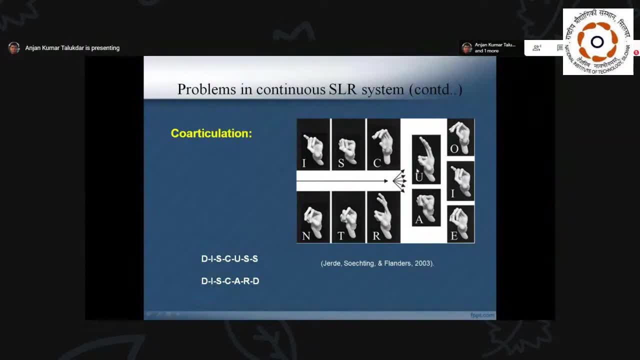 are all similar and this is the simulation case that they are different. there is a significant difference between this, so this is about some problem. there are again many problems for co-articulation that i have not discussed here because of the time constraint, so i have just given a glimpse of that. so now we come to the last part of my presentation, that is: 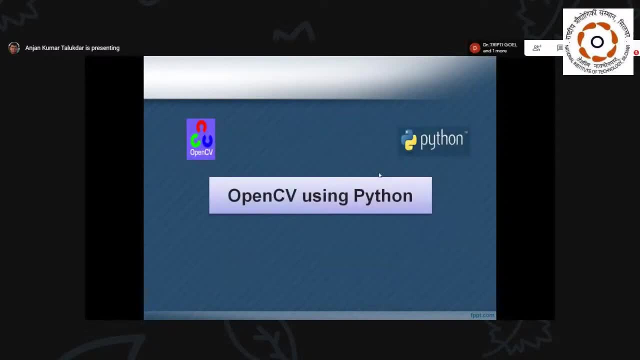 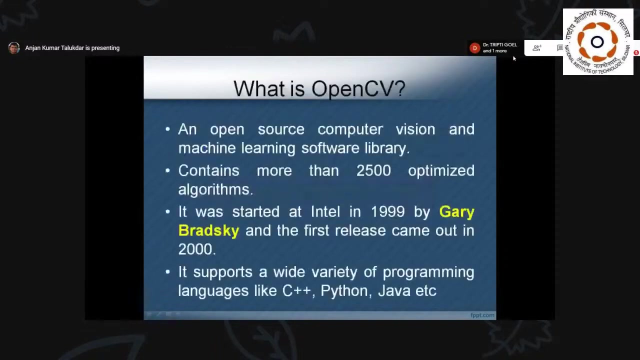 opencv using python. so many of you may be familiar or may not be familiar with this opencv library to implement this opencv based projects. so i'll just briefly give you some idea so that we can start. so, basically, what is opencv? so this is an open source computer vision and machine learning software. 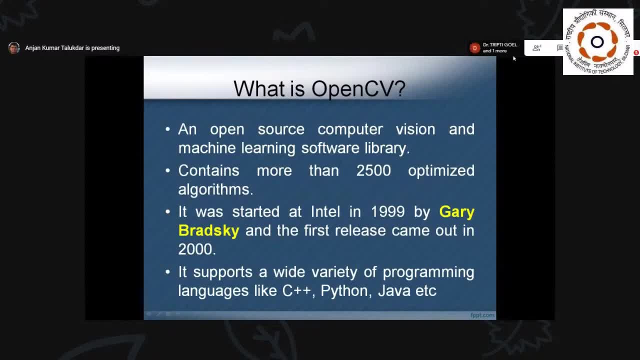 library, so it is basically built for computer vision and machine learning applications and it is open source. so it contains more than 2500 optimized algorithms and it was started at intel in 1999 by gary bratzke and the first release came out in 2000 and it supports a wide variety of programming languages. 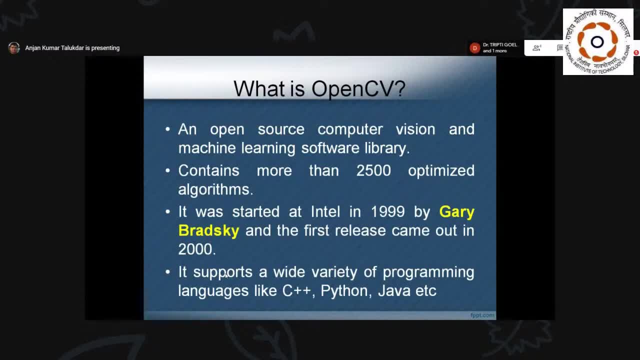 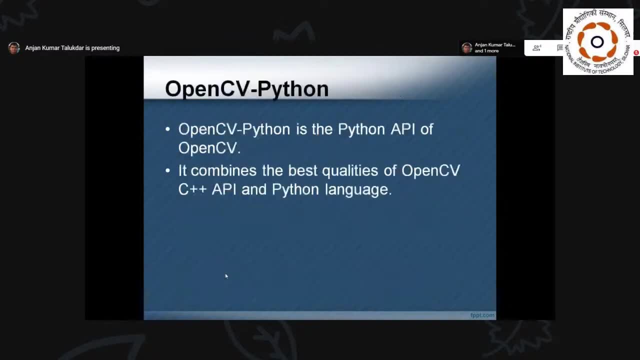 like c plus plus python, java, etc. so so um now opens the python, so opencv python is the python api of opencv, so it combines, uh, the base qualities of opencv, c plus plus api and python languages. so now, why python actually? why python language, or what is python basically? uh, i think, 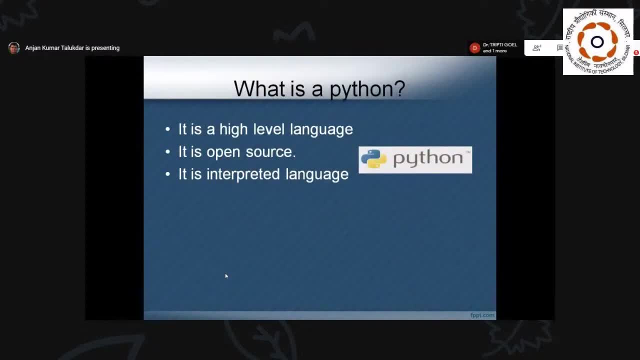 most of you have the idea, so i'll just give you the brief idea about python. it is a high level language, so it is also open source and it is interpreted language. what is interpreted language? basically, it means while you are writing the code, suppose, at that instant only it is compiled, uh. 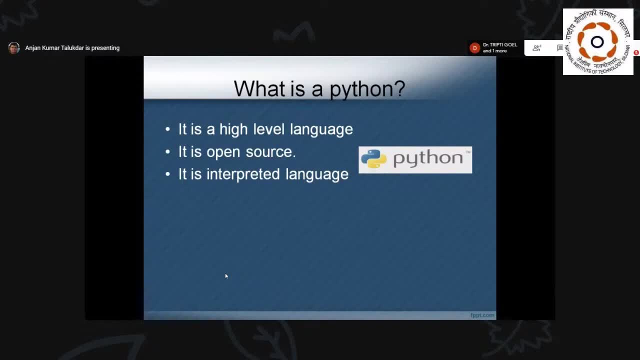 so means if there is an error in your code, it will be shown at that moment only. so it is basically interpreted language it's. it does not wait, uh, for completing the whole program, like other languages here. at the moment you write the code, it will compile and click save. okay, like that. so now why uh? 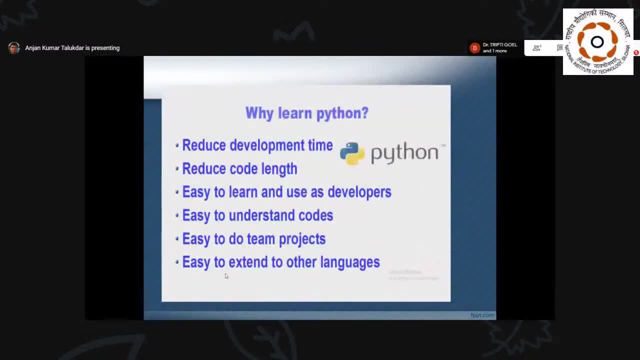 uh learn python. actually, why people are using python nowadays? because it takes uh. it uh has reduced uh development time. reduce code length. easy to learn and use as developers right. easy to understand codes and easy to do team projects. okay. easy to extend to other languages, so i will not. 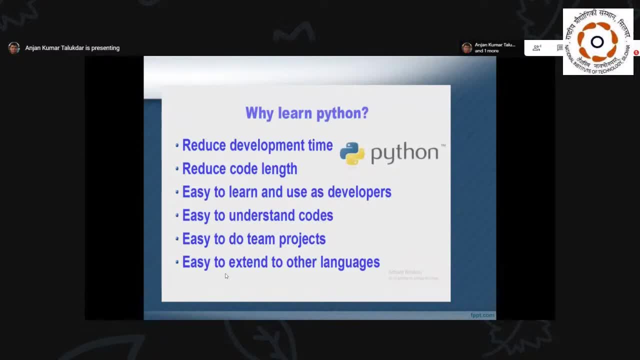 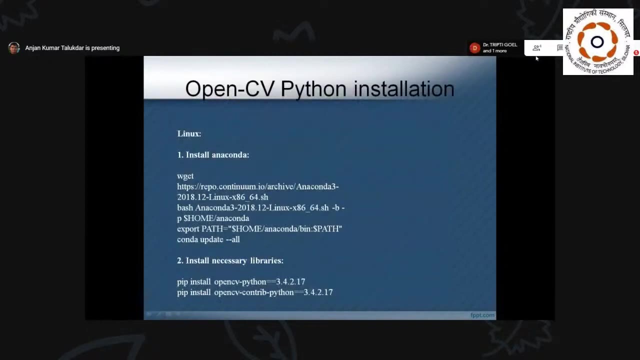 um, discuss python here, because it will take again more time also, uh, and there are many resources in which you can learn python also. so now, uh, open cd python installation. i will give you brief idea how to install python and opencv in your system. so if you are using linux system, then install an. 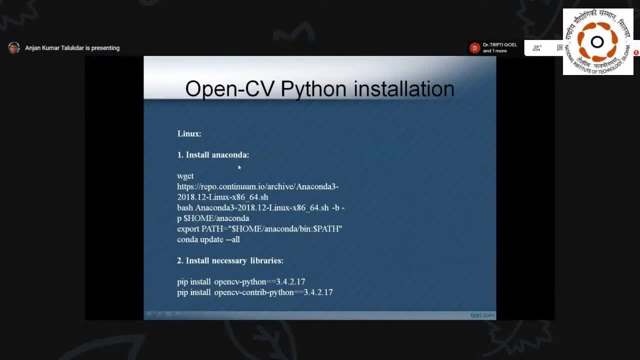 anaconda. actually anaconda is the complete package actually that contains all the library lead to python. okay, so otherwise, Otherwise you have to install Python separately. but better to install Anaconda. it contains all the supported libraries and packages. Then you can install OpenCV. just simply typing tip: install OpenCV- Python. 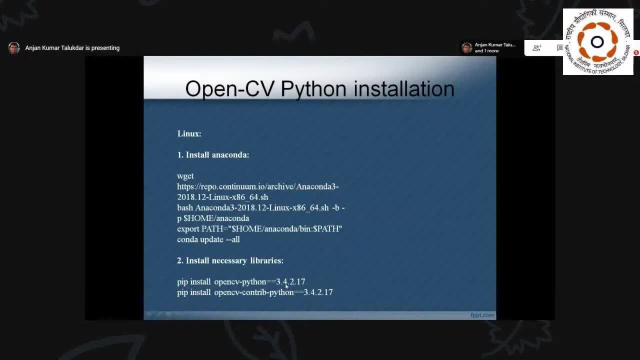 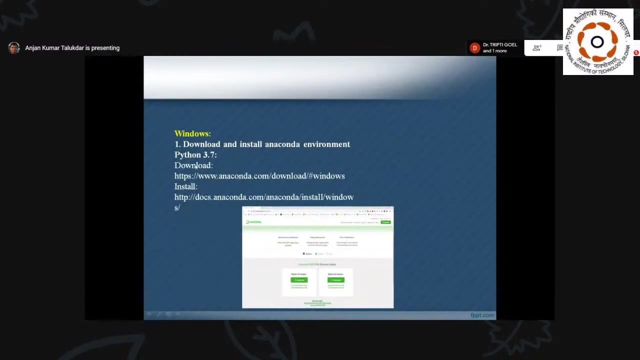 This version you can type. but whatever is the current version, you can type here and you can install it. So I'll show you how to do that. So in case of Windows, download and install Anaconda environment and Python 3.7.7 from. 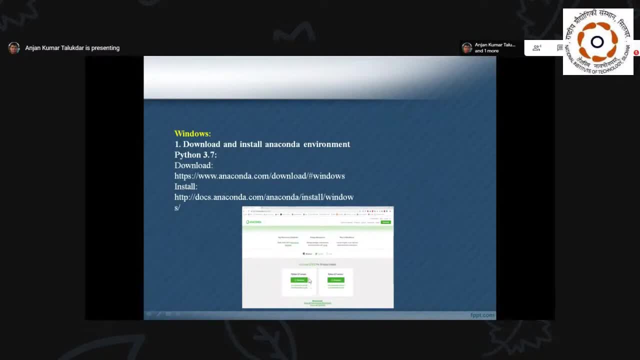 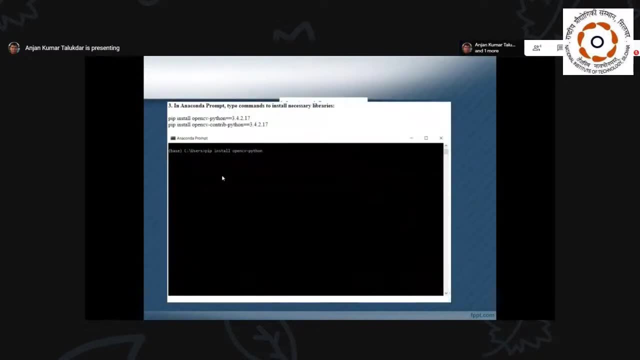 the Anaconda website you can download it. Then, after downloading and installing the Anaconda, then you go to Anaconda prompt and type this: pip Install OpenCV Python 3.4 point. whatever this person you want to download then also. 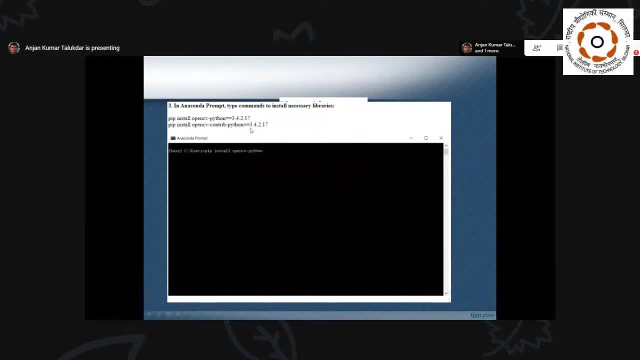 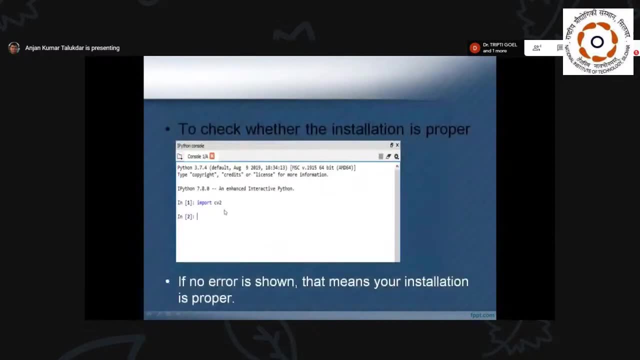 you write. after completing this, you write the second one, then you download the second one also. So that means then, whether your download is okay or not. you can check by typing import CV2 in the Python console. If no error is shown, then that means your installation is successful. 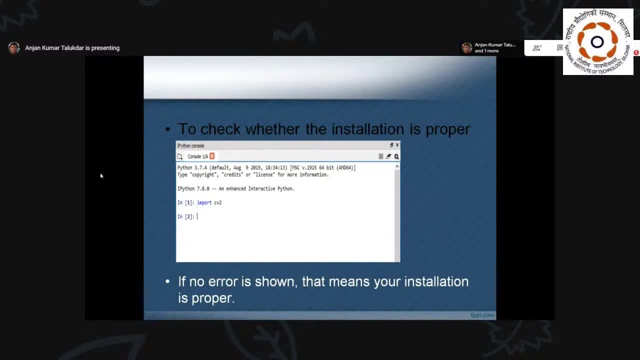 So that's it, Thank you, Thank you, That's it, Thank you, Thank you, I hope that's it. That's it. So your installation is perfect. Import CV2 means your CV2 is the actual library If you are importing, suppose. so if this, no error is coming, means your installation is. 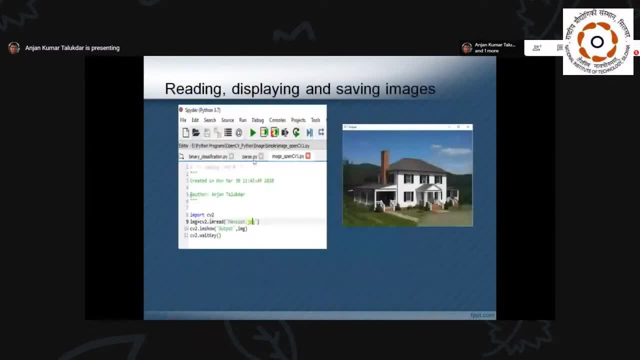 okay, Now I will briefly show you how to read, display and saving images in case of OpenCV. So for that, suppose, import, import CV2.. We import the code. Okay, import the support libraries of computer vision. Then you read the image using cv2.imgrid command. 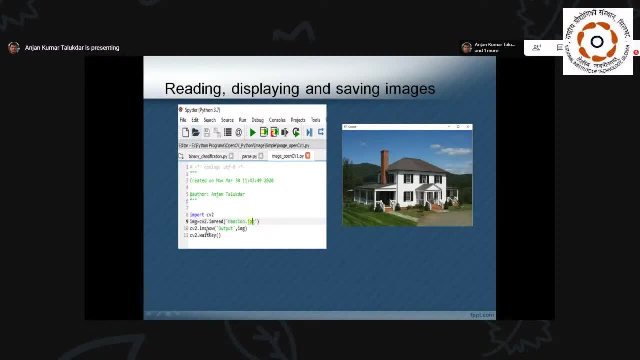 Then this is the name of the image. Then you can show your image by using the cv2.imshow. Then name of the window you are giving, then name of the image: this image, okay. Then cv2.waitkey- okay. So what does it mean? 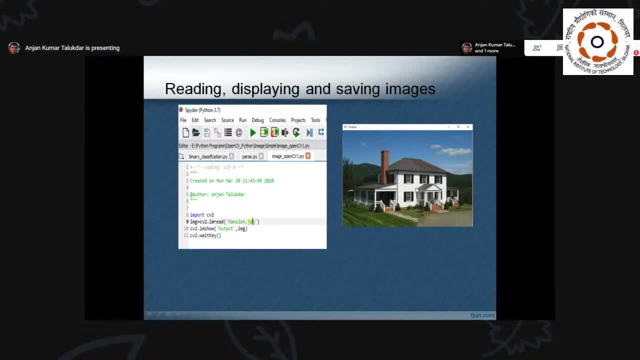 It means this image will be displayed- the output, unless and until you don't touch any keyboard. Whenever you touch the keyboard, then this program will be closed. So then, suppose this is just to display, read and display an image, And this is how to save the image actually. 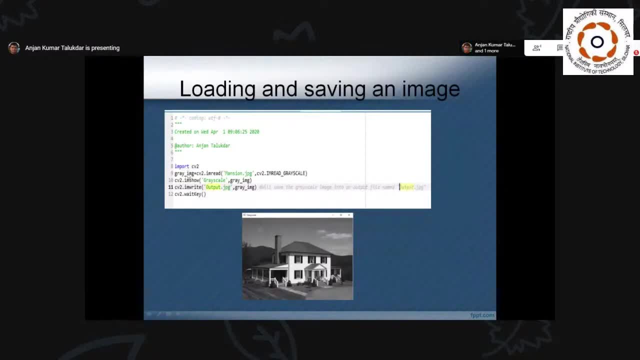 Suppose: loading and saving an image. You are suppose loading the image. also you are converting into a grayscale. okay, Along with reading, you are also converting this RGB image to suppose grayscale. Then cv2.imgrid underscore- grayscale you have to use: 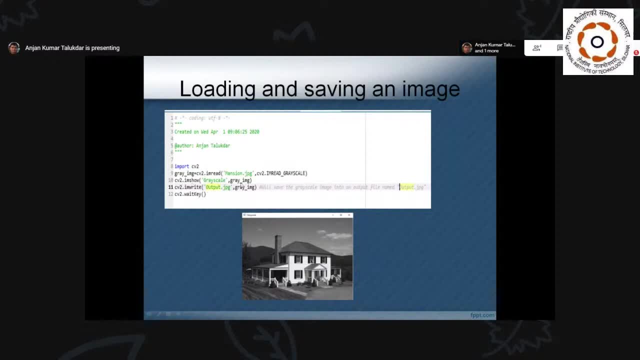 Then you can display both the original image and the grayscale also. Suppose, display the grayscale image. This is a grayscale window, This is the name of the window: grayscale, then gray underscore image. But that will display the image, okay. 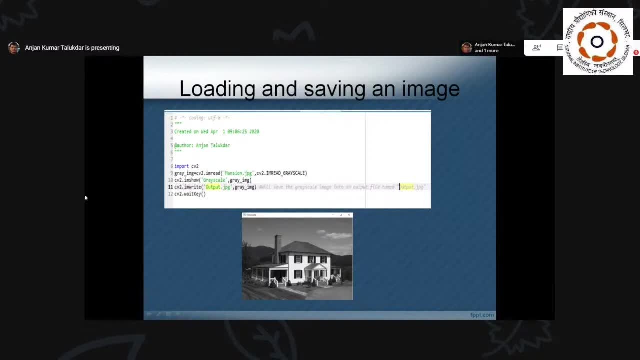 By opening a window called a grayscale. okay, Then after that you can save this image, suppose cv2.imgrid. For that the command is cv2.imwrite. okay, Then you write the name of the image, then the name of the file name you want to save the image. 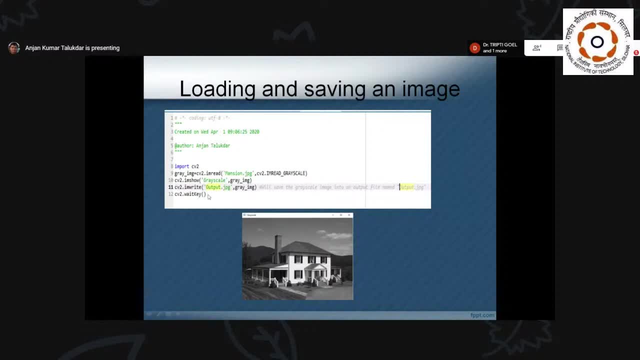 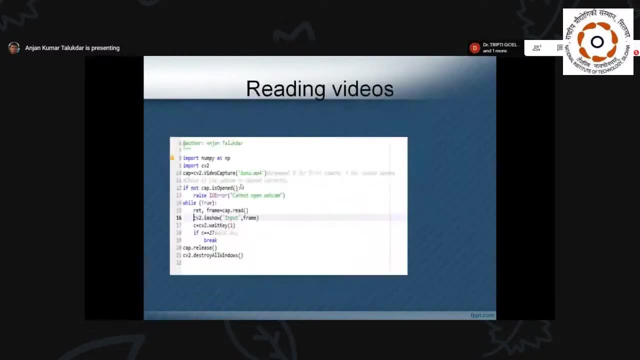 Then the name of the image you want to save, Then again cv2.. So this will save your image. Then comes, suppose, videos, how to read videos? So for that you have to import, suppose, numpy. Numpy is also another. 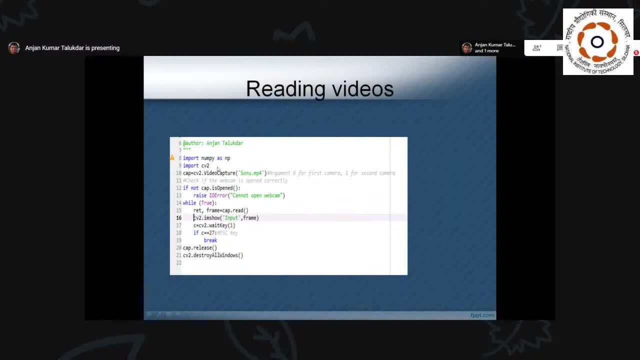 It is an additional library for numerical calculations. Basically it provides arrays and all functions. So import numpy, then input cv2.. Then you have to, then you can read the video by using this command: cv2.videocapsule. 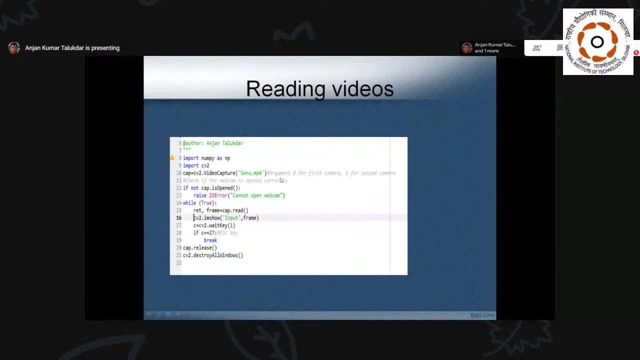 Suppose this is the name of the video. okay, So this then you can write: suppose 0.. Okay, You can. if you write, yeah, suppose 0, then that means it will take. is Suppose 0, then that means it will take. 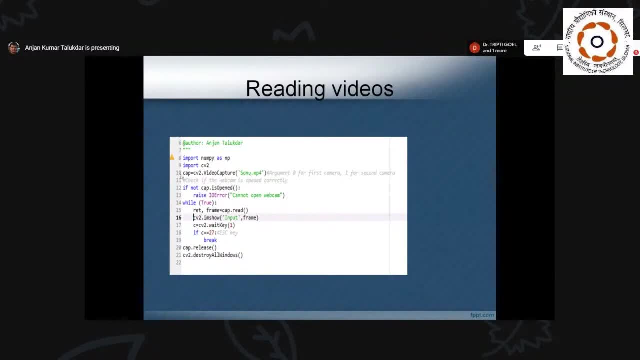 the video from that camera directly. okay, Instead of reading some stored video, you can read it, really read video from the camera also. Then you have to use argument 0 for the first camera or we can use 1 for the second camera, like that. 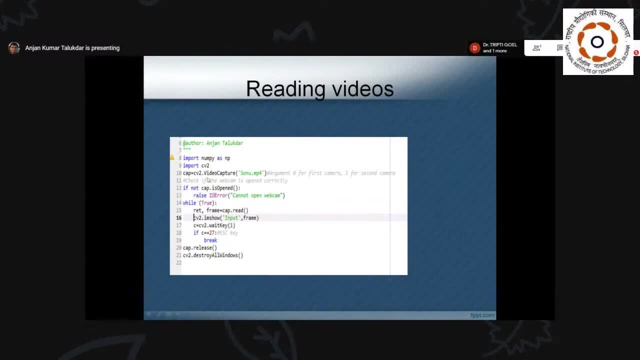 Then you can stay with the camera like that in that wheel. it is perfectly capturing the video or not. you can check if, if not, cap is, cap dot is open, then this, this error display this line that cannot open webcam and otherwise, while true, you can read the frame. uh, frame by frame. okay, then you can. 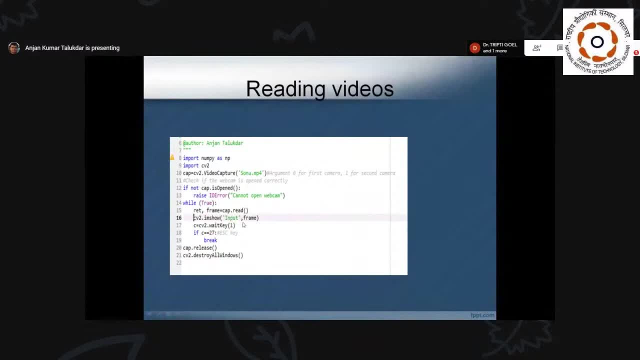 input display the frames one by one, and you can use cbt, dot, weight, key, dot. one. that means here, uh, you can wait for one millisecond. means one frame will display, for suppose, one millisecond. uh. and if c is equal to 27 means we have put the condition that if you press the 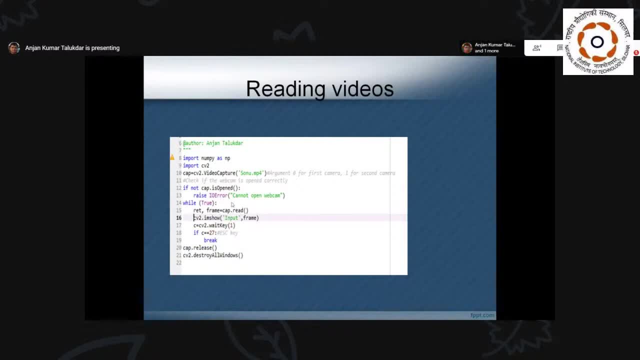 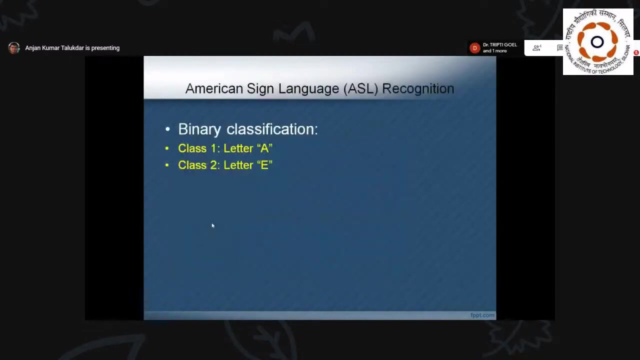 sd key, then your file will be closed and it will stop uh capturing the video. okay, then we can release the window and destroy all the windows. okay, so this is uh how to read a video from camera or from your drives. now uh, i'll briefly show one uh program uh for american sign language. 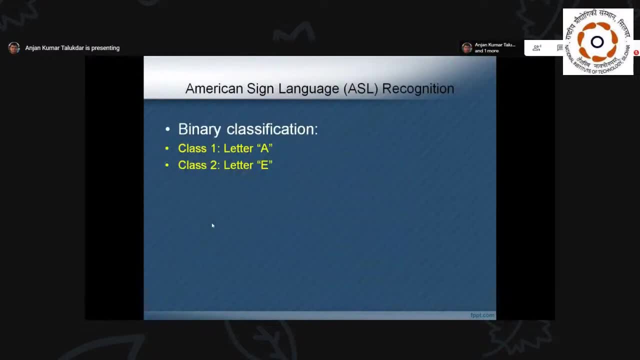 recognition. uh, basically for binary classification, suppose, suppose i am considering two letters, a and e. okay, i want to classify whether the input letter is a, or input sign is a, or input sign is e. okay, so this is basically my uh block diagram. so first i have suppose, 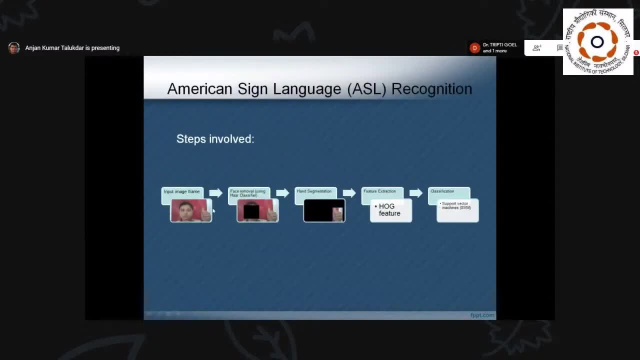 read the in input image frame. okay, then i have removed first the face part. okay, we have to remove the face uh part because i am going to use uh skin color base segmentation technique to segment this uh palm from the background. so that's right, the skin color of the face is matching. 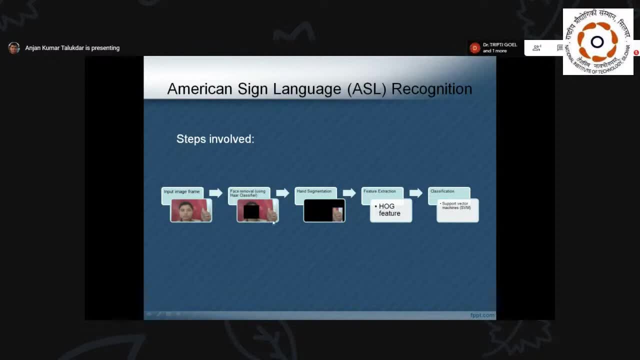 with the skin color of this palm. so that's why, first, i have to remove this face. so i have used face removal uh technique using hard classifier, okay, then, after removing the face- now, actually, i have converted this rgb image to some uh hsb image, okay, so so that, 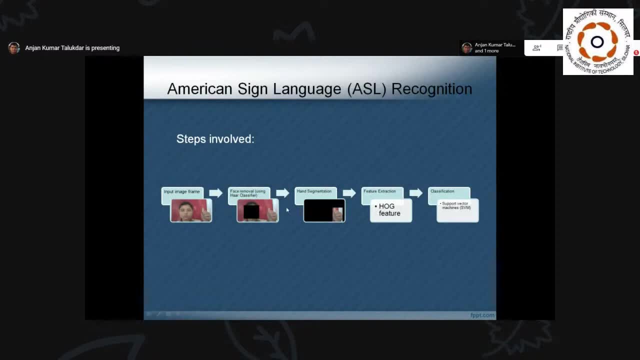 uh segmentation becomes easier because in case of rgb you have to control three parameters, rg and b. but if you convert to hsb or yuv, then color and intensity part will be separated, so you can uh easily segment the color part using hue and saturation parameter. okay, so that is the technique. 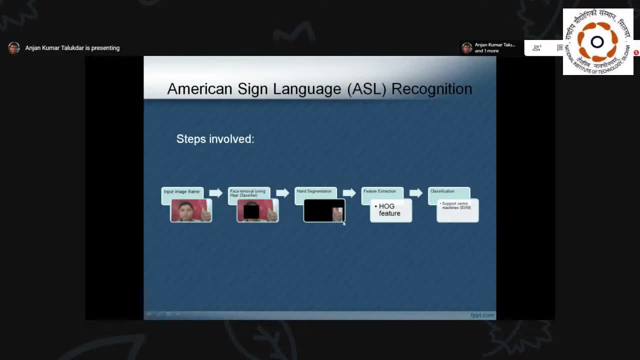 so then, after that i have segmented this hand also, i have localized this hand, suppose then i will, uh, we use hop features, actually histogram oriented gradient feature. okay, so proposed by nabneet dalal. he is an indian also, so i will be using hop features, histogram oriented gradient. 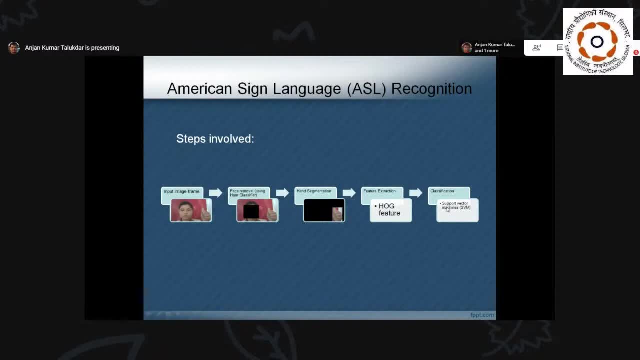 feature. then i will train this uh classifier called support vector machine, uh for uh different, uh different signs of a and e. okay, so after once training is done, i will input the any letter, a or e, as input and check whether it is classified or not. so for that. 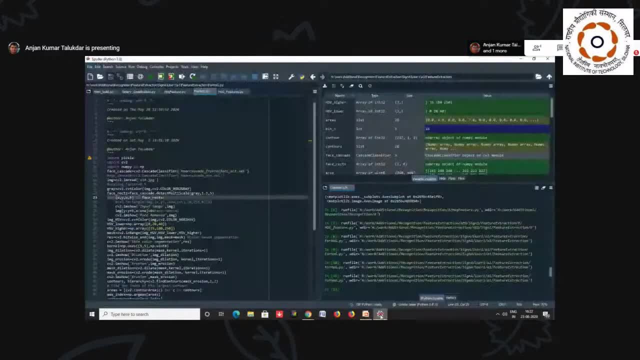 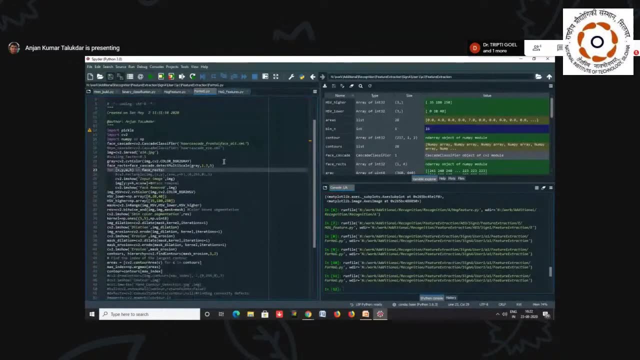 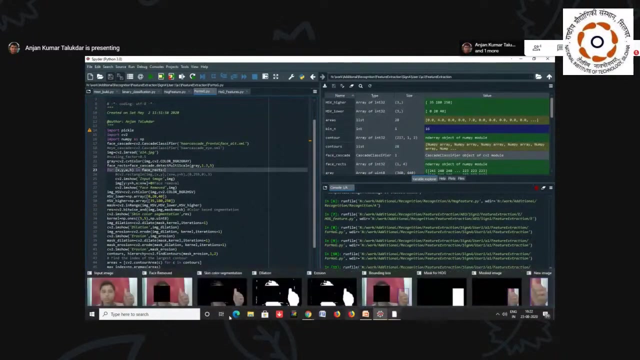 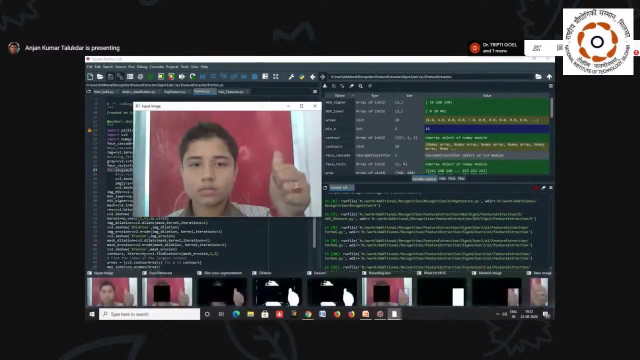 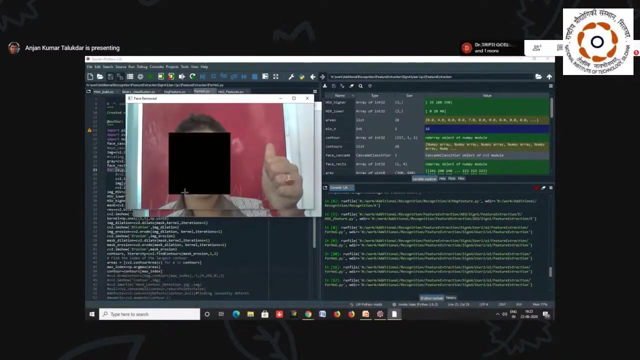 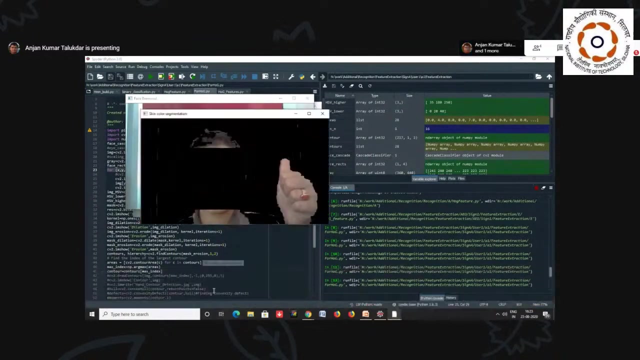 this is my actually programming part, so so first, uh, so let me first run this code, so here you can see. first, this was our input image, okay, then i have removed the face using high classifier. then i have used the uh- skin color based segmentation. now you can see: uh, i have used. 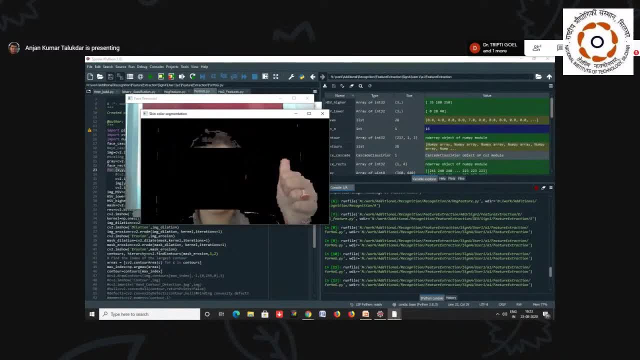 a skin color with segmentation to segment this skin part from the background. so, as you can see, this, uh, this part of the skin and this part of the skin is still coming, so we have to remove this part. but we can first remove this small parts, small, small parts, using dilution and 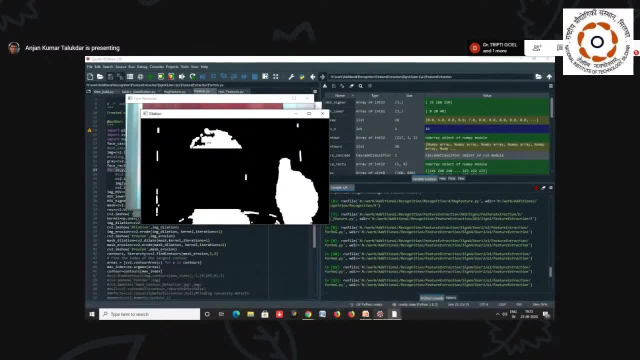 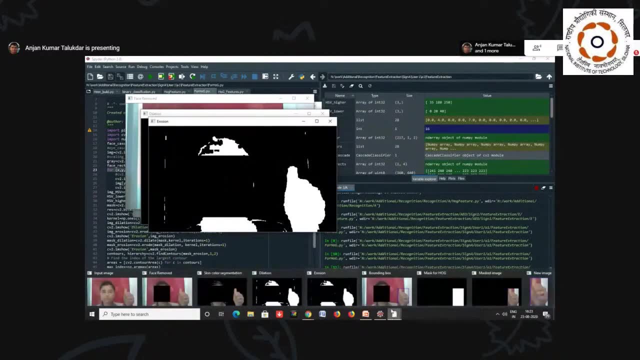 illusion technique. so i have used first dilution, then illusion, also to remove some parts. then finally, i have used a contour, uh matching base textile. so i have found in the contours of all these parts and i have selected a larger uh. contour means the contours have contour, having the largest area. 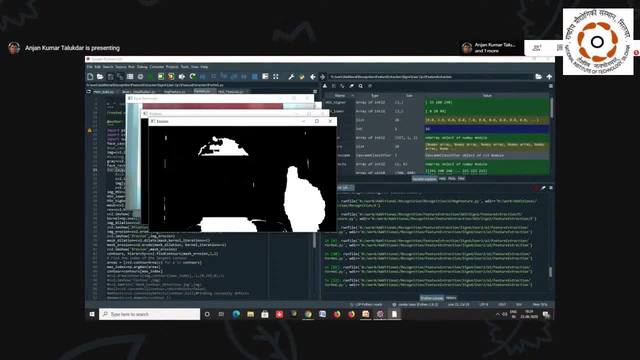 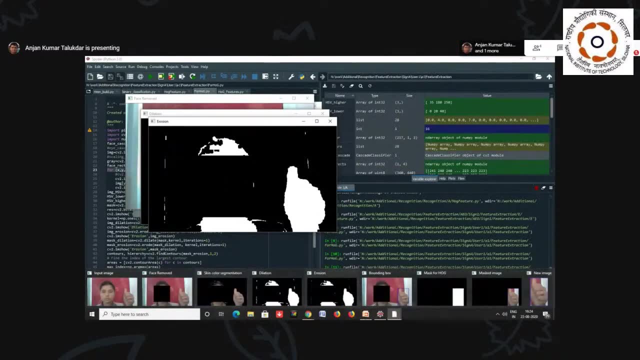 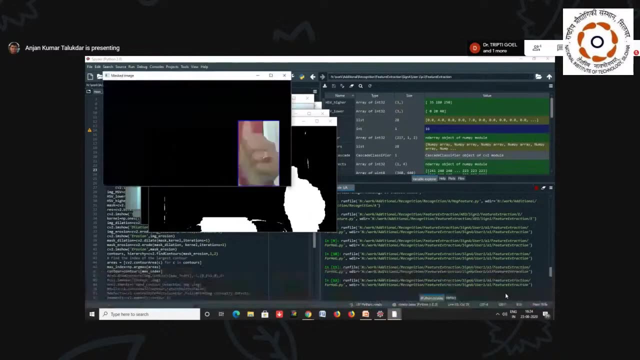 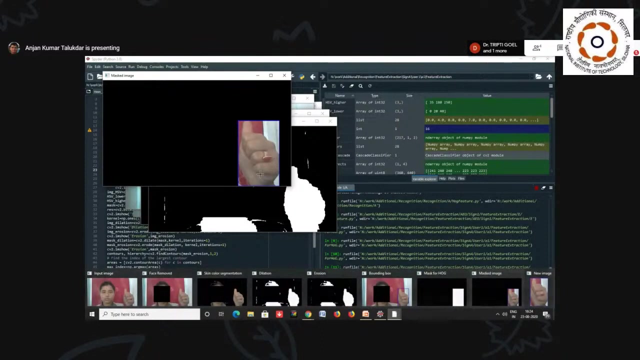 So here, obviously, this palm part will have the largest area. So I have removed the other parts and only kept the palm part. So now this is how I have segmented the palm part from the background. So now, after that, I want to cut this part actually so that I can directly input these. 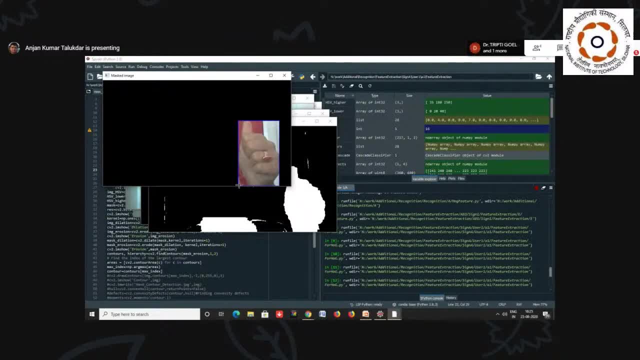 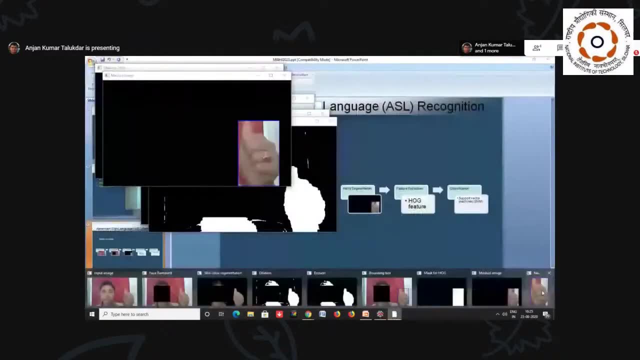 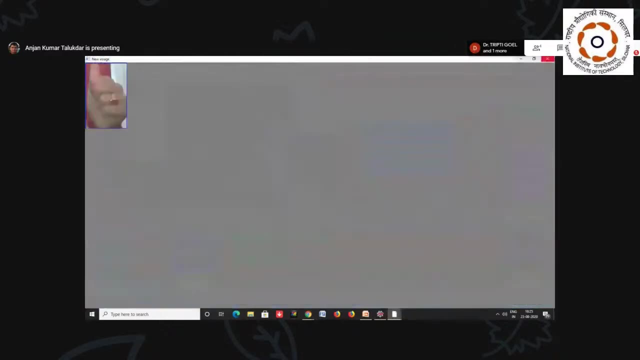 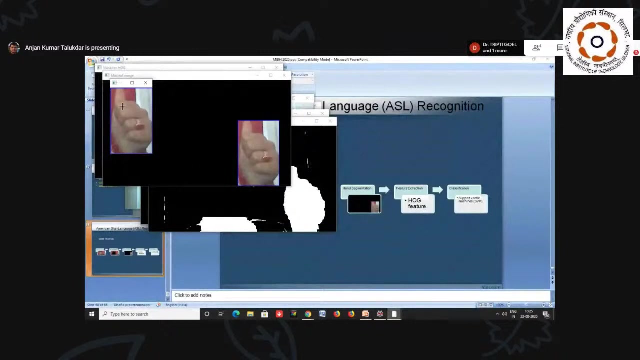 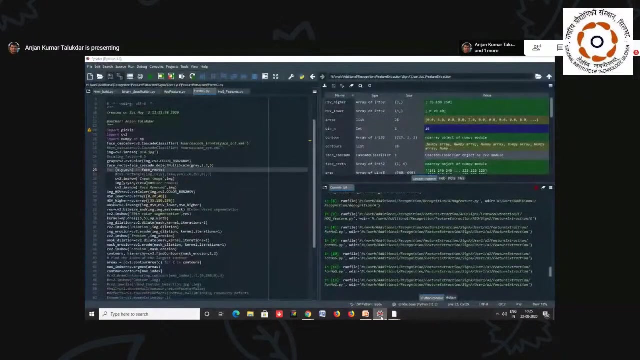 images to the hog feature detector. So for that I have separated this part from the background. So this part I have separated. This is now new image for feature extraction. Now then I have used hog feature detector, Then finally I have used the classifier. 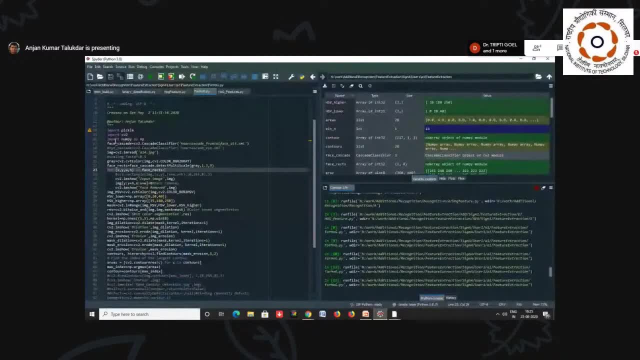 Now I will show you step one by one. So first I have imported this v2 and umpire, Then this phase cascade classifier means hard classifier for phase detector. It is already there in the OpenCV library. You can directly use it. It can be used for other detection also. 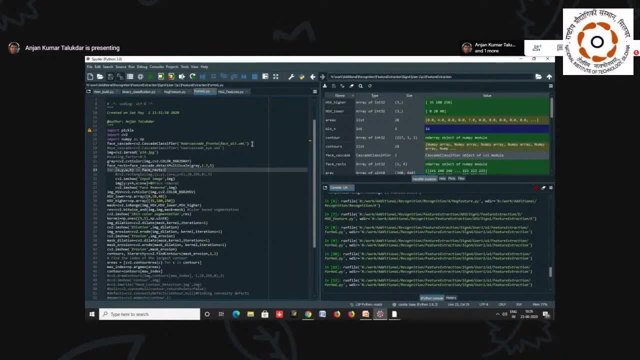 Not only phase You can. You can use it for detection of human or any other objects also, But for that you have to train it before that. So now then I have read the input image, suppose Means this image, Then I have converted it into grayscale image. 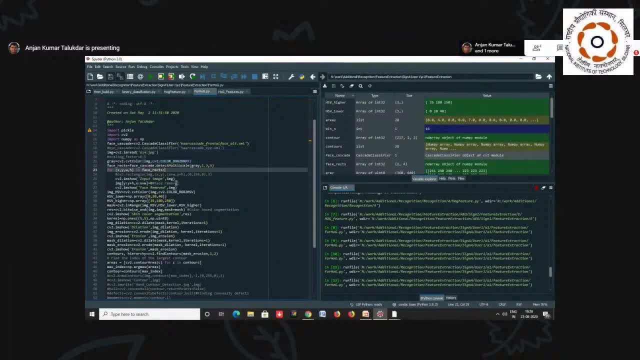 So that I can apply this hard classifier. So I have applied hard classifier, Then detected the phase part And then to remove this phase, To remove this phase part, I have used this, this part, basically. So first I have constructed a mask, actually, 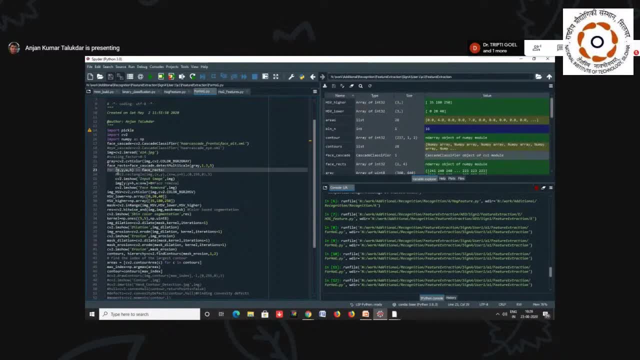 And then I have removed the face. So here actually, x, y, w, h are the x, y is the center of the point, of corner points, And w and x are the width and height actually Then, After removing the face, 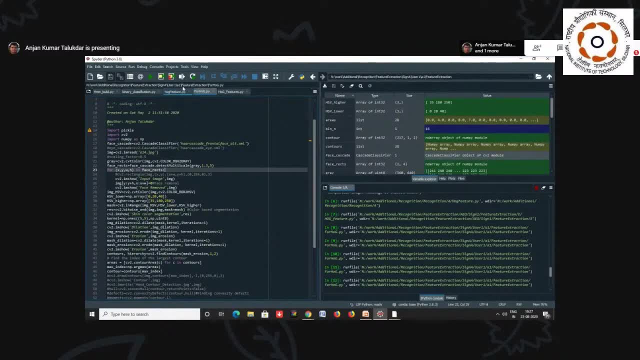 Then comes your. Then I have converted this rgb image to hsb image. Then I have selected the threshold values for skin color. Then lower values for hsb Plan is 0,, 20 and 40. And higher values for hsb. 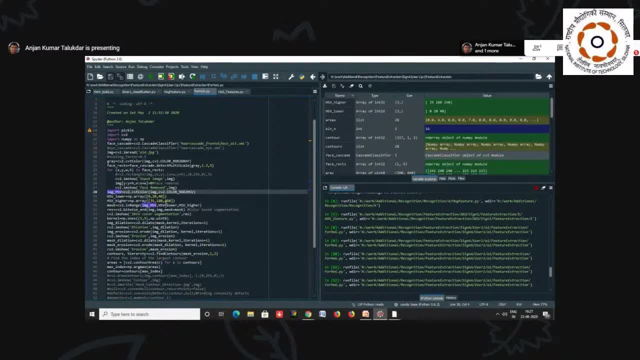 Then I have converted this rgb image to hsb image. Then I have selected the threshold values for skin color And lower values for hsb. Then I have converted this rgb image to hsb. Then I have converted this rgb image to hsb. 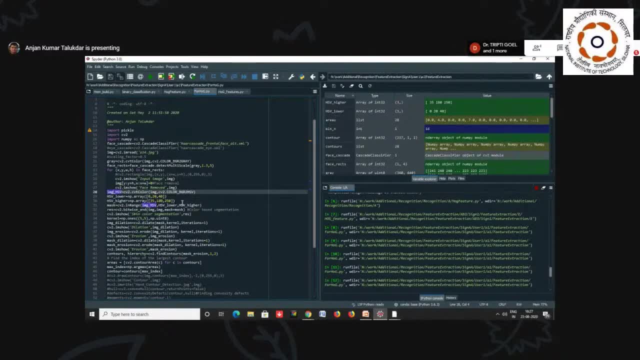 And lower values for hsb And higher values for hsb, And then my actual values are 0,, 3 and 25.. This is I have actually selected manually by going through the pixel values of this image for skin color. Then I have removed the. 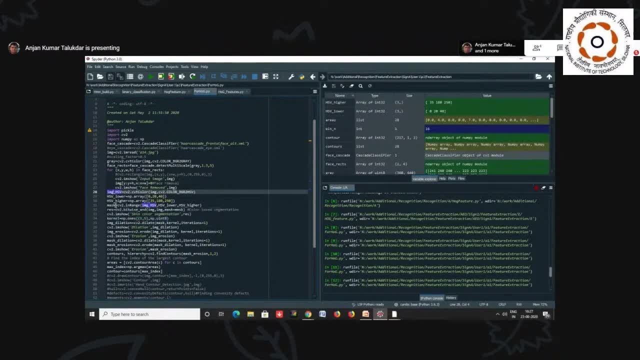 Then I have Masked using this threshold values, And then I applied my mask and then i applied these marks on this original image and this is basically nothing but the b twice n operation or the color based segmentation. then i have shown the segmented image. then this is for dilution and erosion. 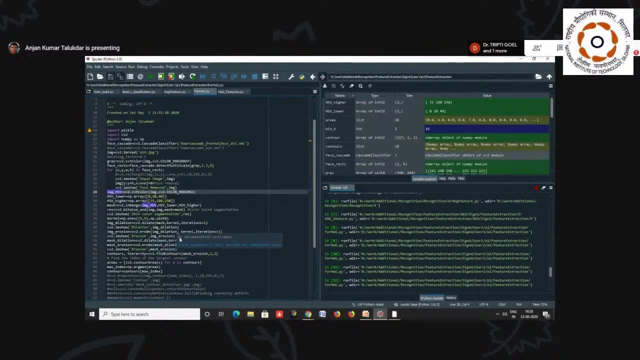 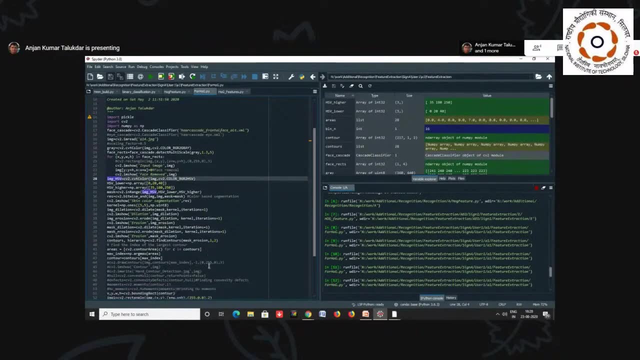 it may not be required in some cases. you can use it then. then this is the code for finding contours areas. okay, first we have found how many contours are there by using this common cv to the fine contours. after finding the number of contours, we have found the areas of each contour. 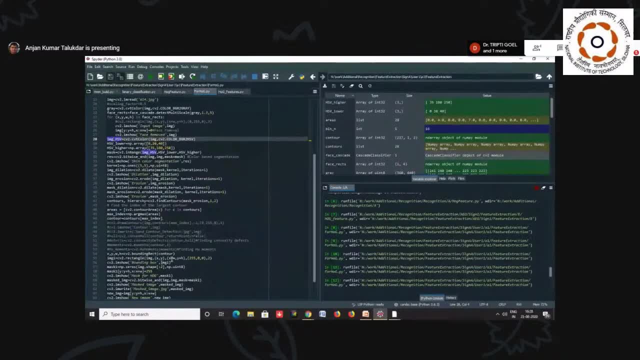 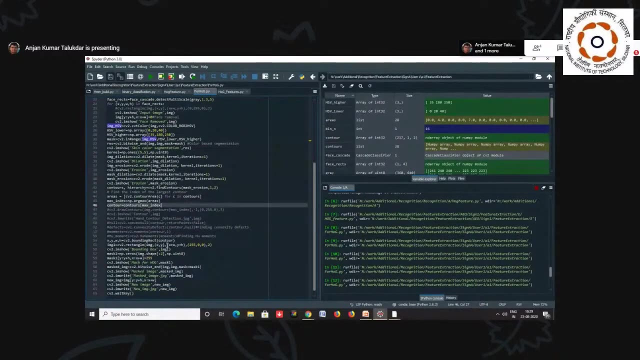 and we have selected, finally, the contour use, larger index. next index: we have selected the larger index, basically for the pump part. okay, then we have created on bounding box for selecting the pump part using the cv to the bounding red function. then i have separated that uh pump on the background for the hog uh fisher extractor. now we can now define the hog uh. 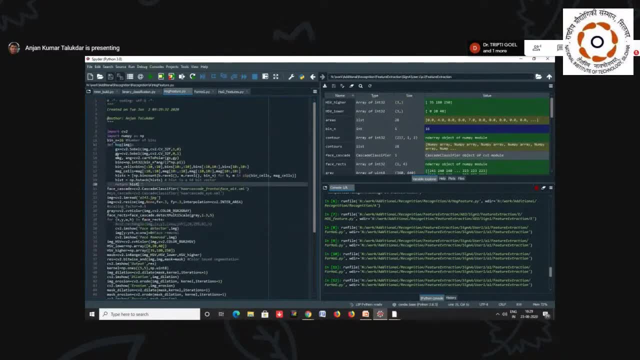 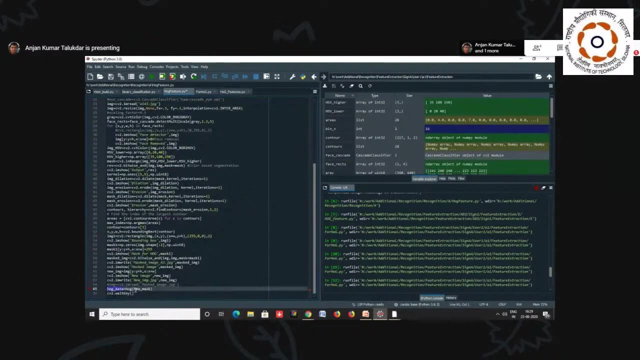 fisher extractor. here as a function you can. this is the upper home extractor part and you can input this as a hop. now you can give your segment here, part of the segmented pump part, as input to the hog extractor and finally it will give you the hog features. uh, likewise, after extracting the hog features, 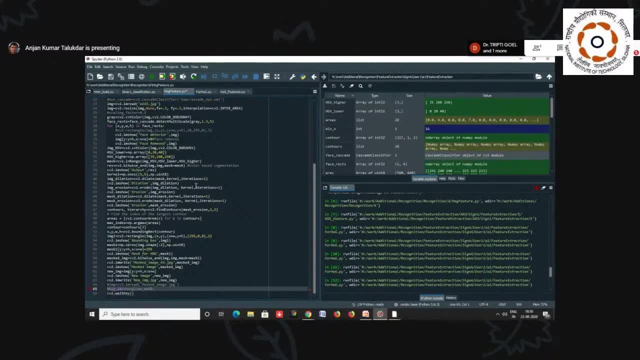 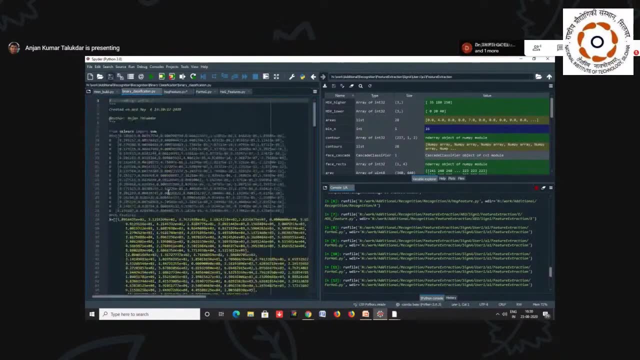 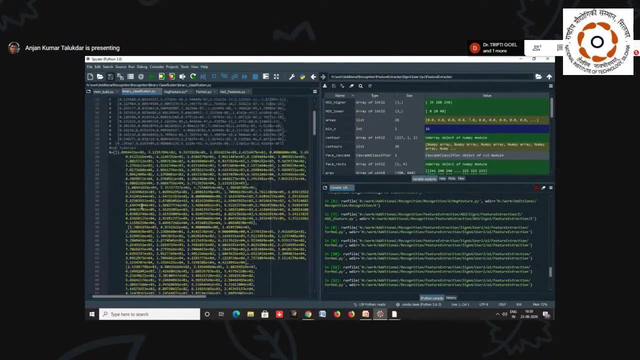 uh, i can now train the uh classifier. so for classification actually, uh, suppose we have to use a scale and library for a uh sbm. that means the support vector machine classifier I have- important is still on library. then included the all the input feature vectors for both a and e. I can generate a separate file also for that, then you. 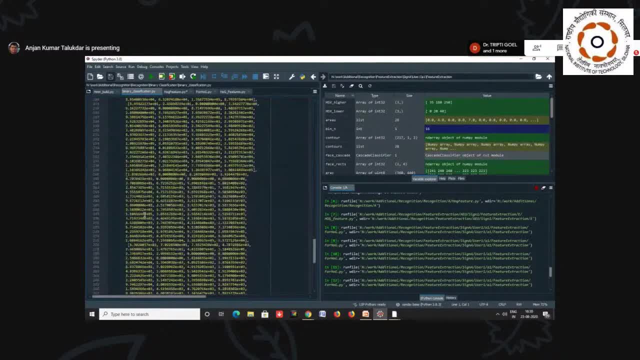 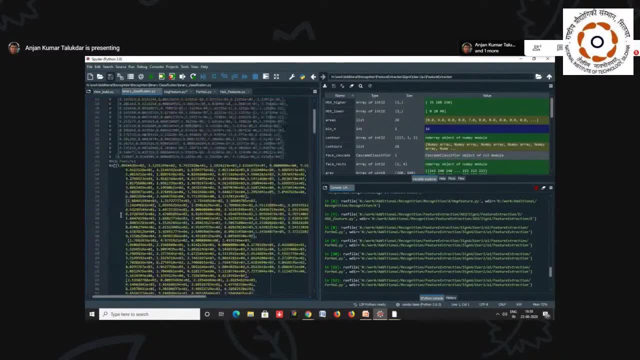 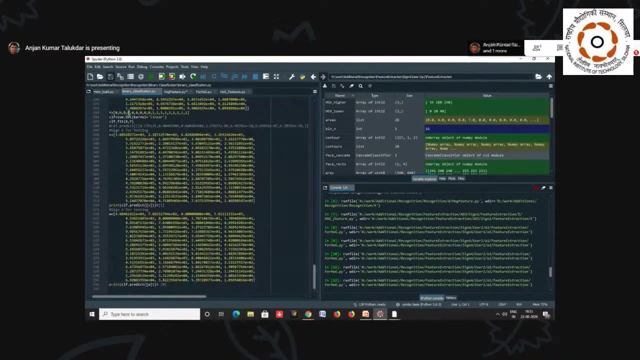 can read the file also. then this is about our input level or fear into features. it's our input feature vectors, metrics. then why is our output classes? 0 for a, 1 for e. then I have use a linear cluster as VM plus pair and then I have 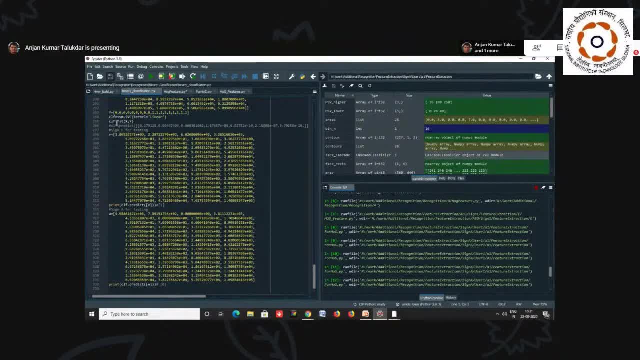 the training part, celebrity. we trained as VM and for testing support. after training is done you can taste whether it is perfectly classifying or not. then you can suppose I have given another input for testing. then I have. if you run it again now, this predict the output using this command. so once you, 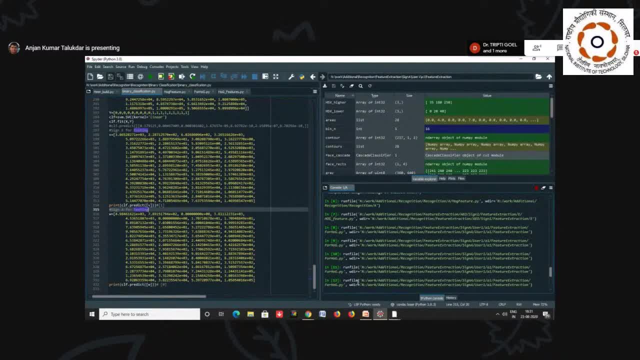 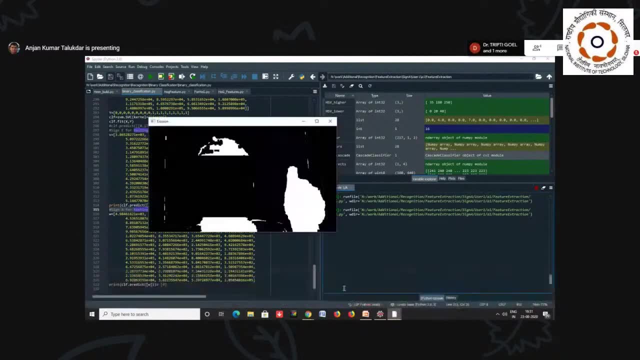 run. Oh, before that I have to close all the other previous windows. how to close it? it's really, you have to first place on the image. if you don't place the STP, then it will be closed. VPS program will be closed. ав. Separatist program. 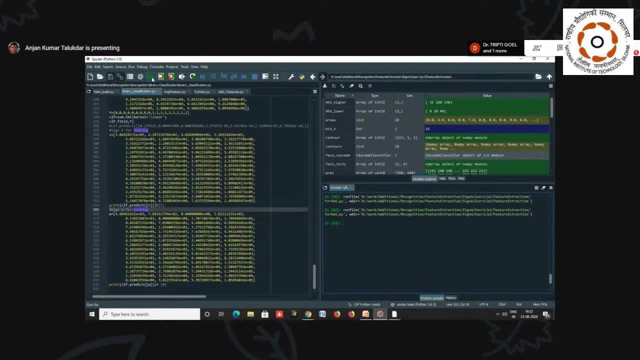 but now Portal will be there. but now Portal will be there. Oh, board is not. Well, the way that I can work with bah mission is the guys on my yourself voice. now it's being run. so we have basically tested for two signs: one for e, one for a. 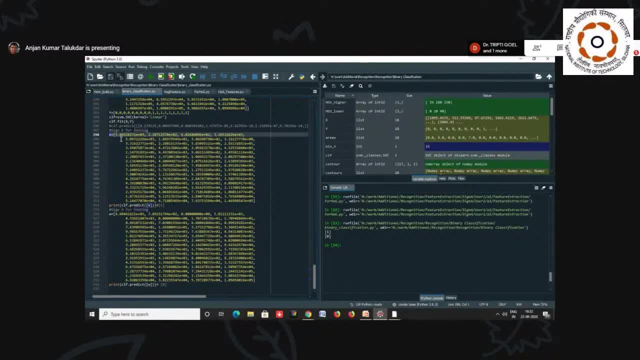 this is the actually input feature vector for e, so it is giving output as one. and this was the input feature vector for a, so it is giving output as zero. so this is how, actually how you can build one industry condition based system in Python using OpenCV library. 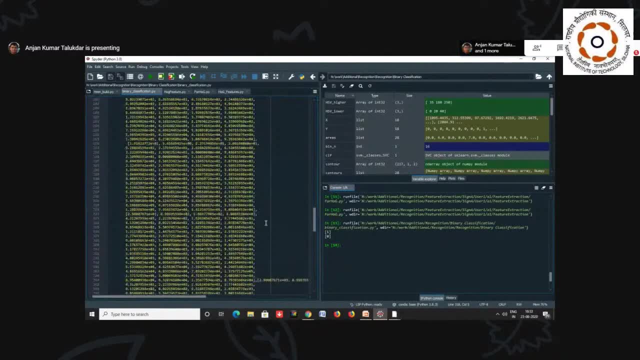 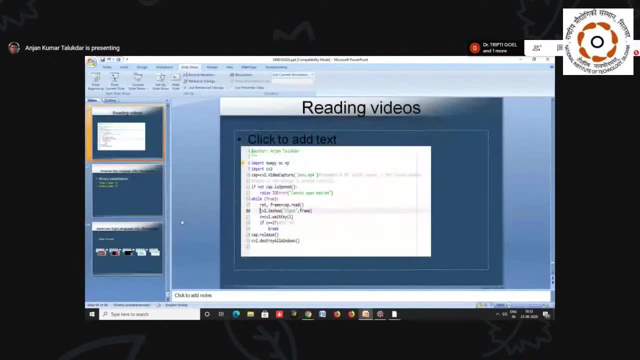 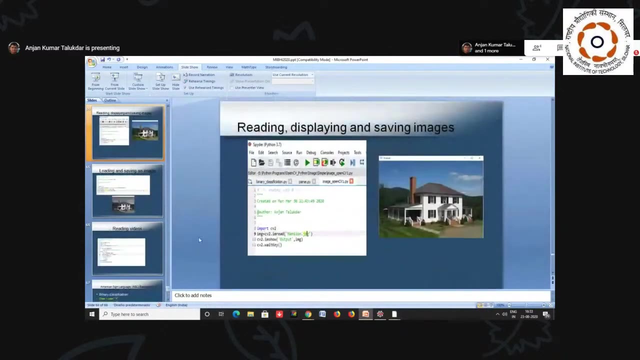 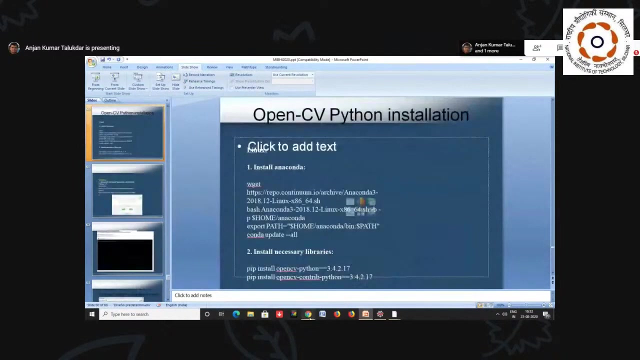 so this is the just to give you a brief idea so that you can start with this library. then you can learn many things step by step. so this is about my this class. now, for any query I can, okay, for that I think I have to go through, madam. 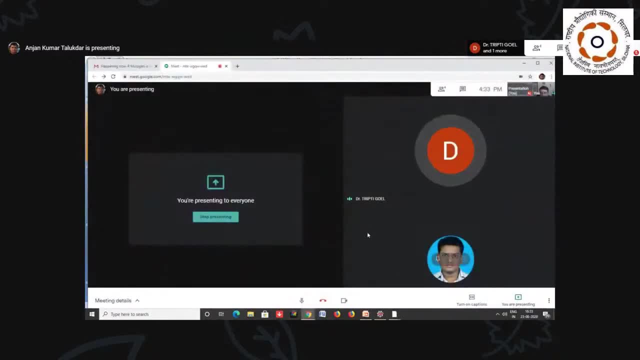 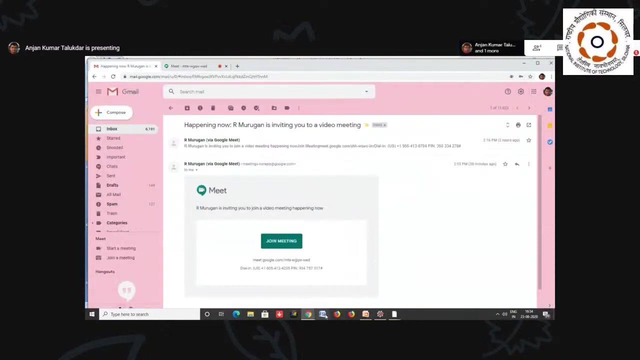 how many is it? how many seconds computer take to detect the fan gestures? that is a question that is coming, sir. how many second computer tape to detect the hand gesture? okay, okay, she, I have not slapped that part, but you can say there is a common in OpenCV using that. a second she that part. but you can say: there is a common in OpenCV using that. a second moment, okay, because we haven't just captured that by the app, so you have to activate the hand gesture power. that is that, Madam. just do that and you don't spell master by your hand. 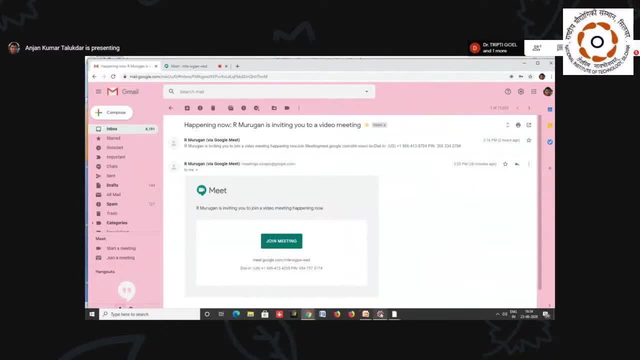 okay, then logical. so basically the computer cannot hela" ed An. here it is the. thats okay good question, isn't it me see from my mind? shit, okay, this is something down to my brain. okay, better, and did you command you can find out the time taken for calculation? yeah, you can do, that is important. 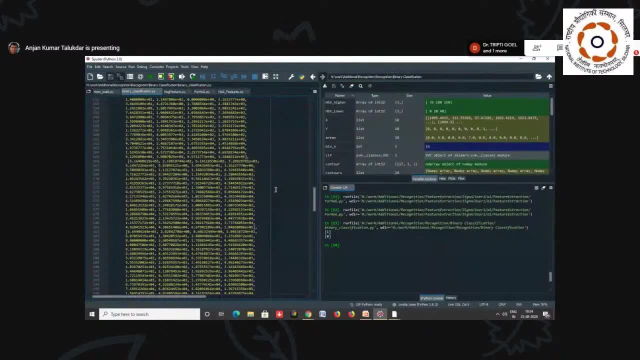 if you are comparing with some other techniques or some processing time, and then, yeah, this is important. yes, you can do that, you can find that, but i have not calculated that. yes, okay. so second question is if augmented reality and virtual reality is the part of a computer wizard. yes, yes, yes, there are some applications of computer using. 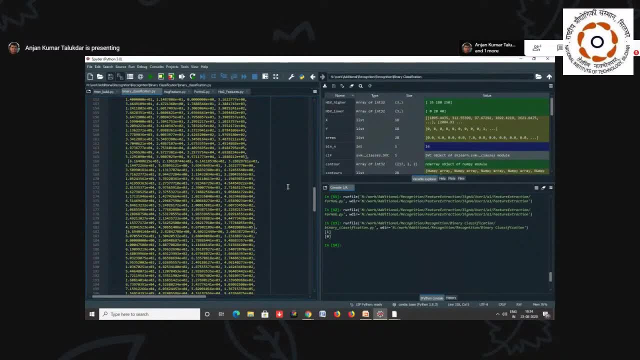 can we detect whole human system through hand gestures and diagnose the disease? sorry, can we detect whole human system through hand gesture and diagnose the disease, whole human system through hand gesture, whole human system. yes, okay, uh see, uh, you can observe uh his uh gesturing. suppose he's your heart is sharing. 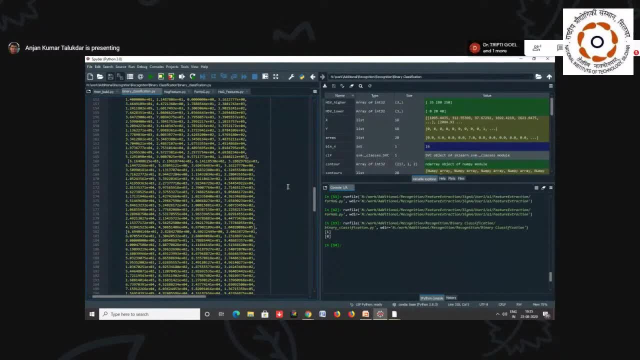 whether his sharing is okay or not, suppose uh, if he has some uh neural problem, auto neuron problem, he or she may not be able to do the gesturing uh properly. so this can be actually one technique through which we can detect uh some kind of diseases for a person. or we can detect his gait or walking style, suppose, or from those we can determine. 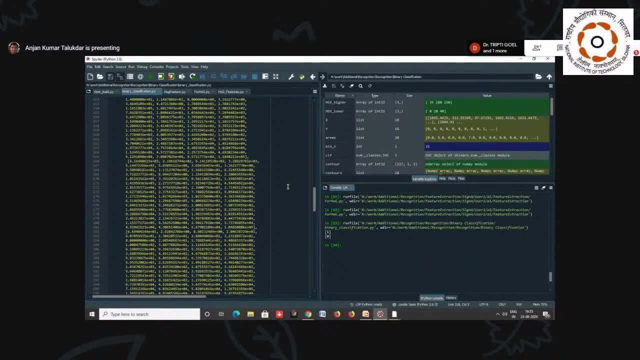 his walking style is okay or not, or his posture means sitting posture, or these are okay or normal or not. so by observing those things also, we can uh detect whether a person is maybe having some health problem like that. um, okay, sir, that's all with the questions queries. okay, thank you, sir. okay, you're welcome.